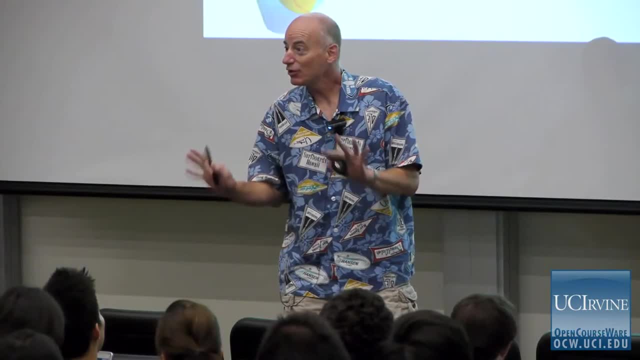 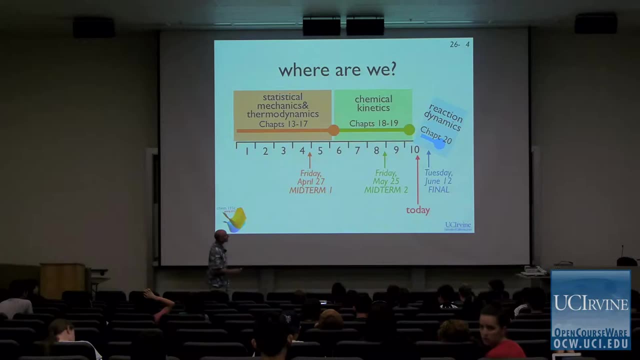 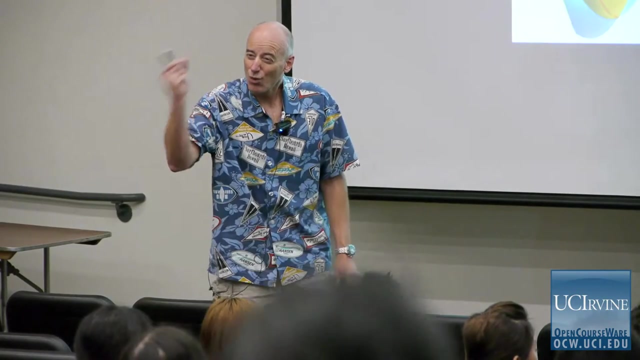 from Professor Martin, And I know you know a lot about quantum mechanics and spectroscopy, and that's good, But everything else is important too, and so this subject is actually very, very important to us, and so I've tried to pick out the one thing that I cannot allow. 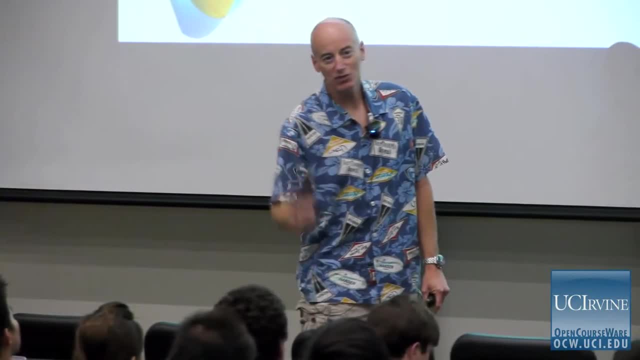 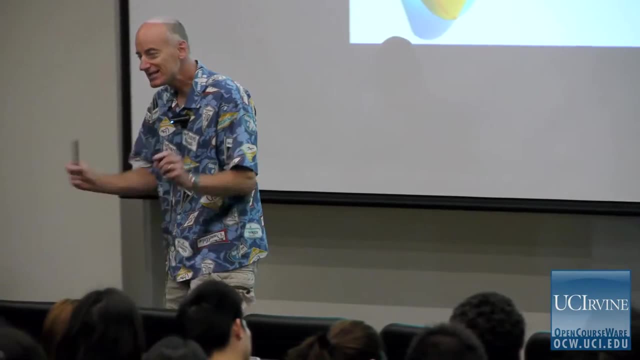 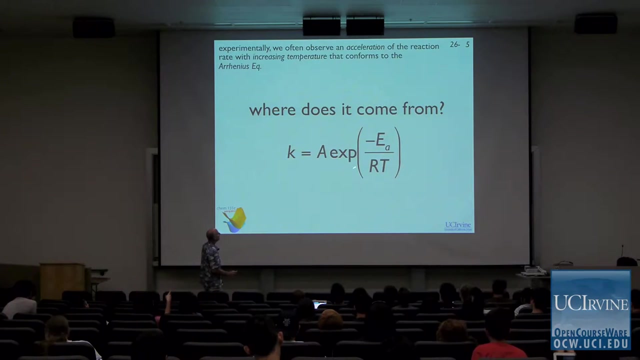 you to leave this class without knowing. I've tried to pull the one thing out of reaction dynamics that you've gotta know about. This is the one thing. this lecture, all right, I'm going to tell it to you. Basically, what we want to understand is: where does the Arrhenius equation come from? When we look? 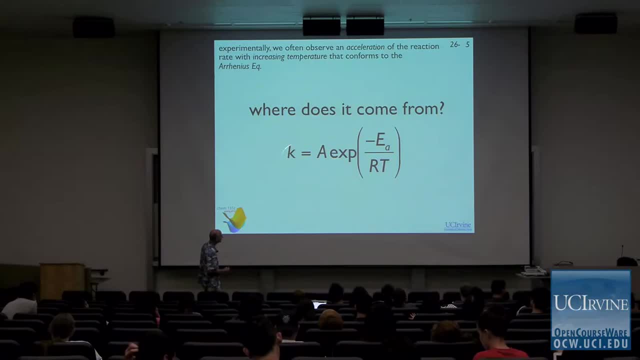 We measure the temperature dependence of reactions. This is the reaction rate. Most of the time we find out that it conforms to this equation. right. We make a plot of log of the reaction rate versus 1 over T. We get a straight line. 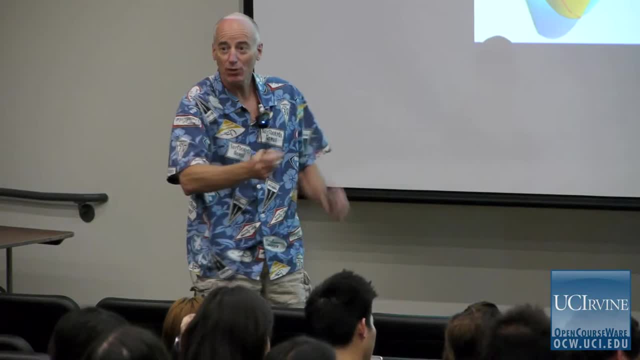 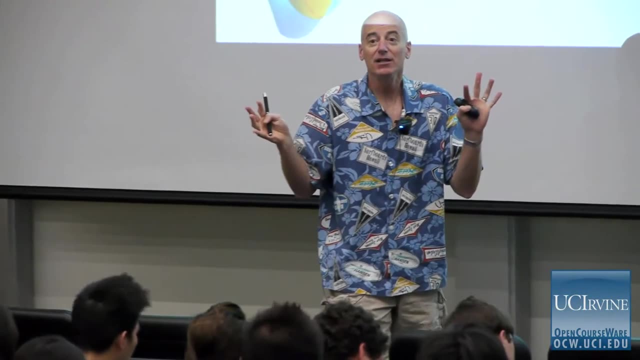 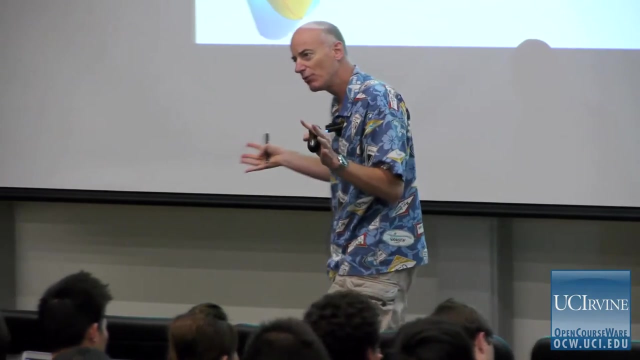 We get the activation energy of the reaction from that straight line and we report that and we think about that. that guides a lot of what we do as physical chemists, But we have never explained where this equation comes from. In some ways, this is the most important equation. 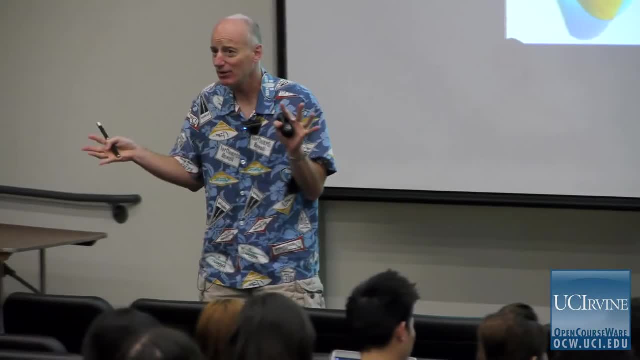 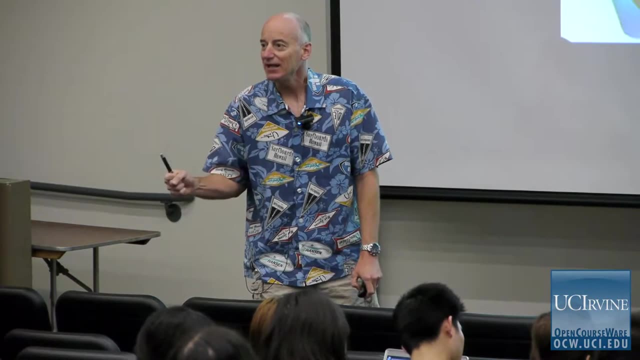 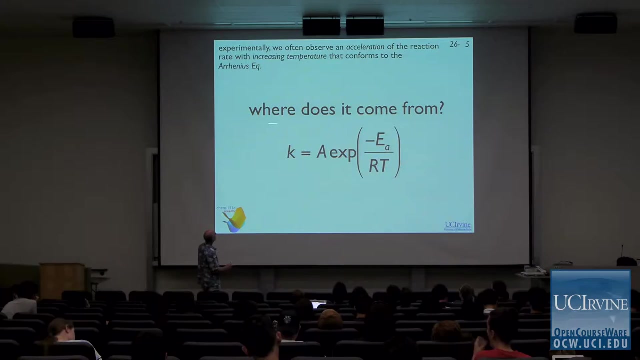 in chemical kinetics, but we haven't talked about what its origin is, Fundamentally, where does this equation come from? So we're going to do that today. I can do that in one lecture. It reminds me, of course. this statement is grammatically incorrect. 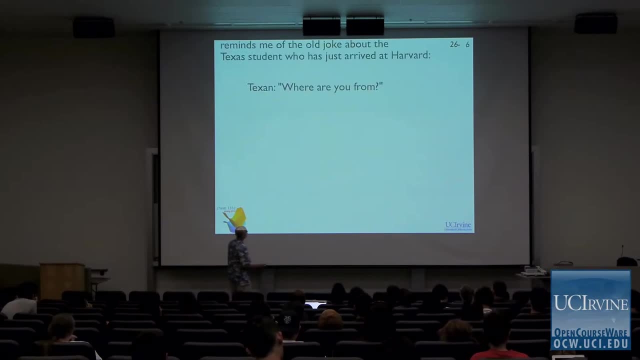 It's a dangling preposition. It reminds me of one of my favorite jokes. The Texas student goes to Harvard and he asks a Harvard student: where are you from? The Harvard graduate says: well, I come from a place where we do not end our sentences with propositions. 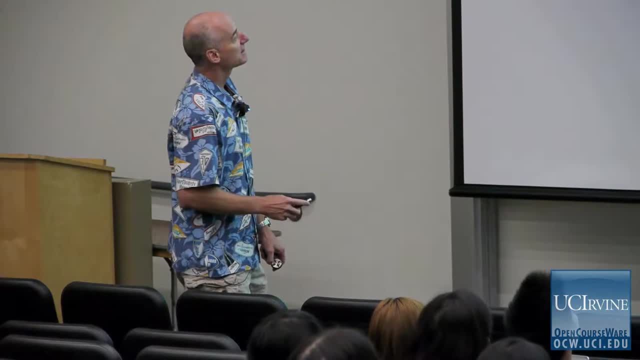 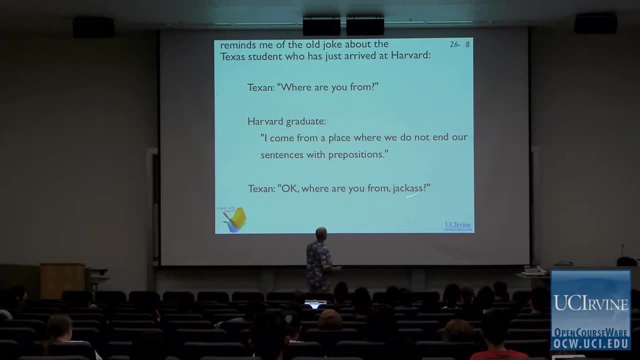 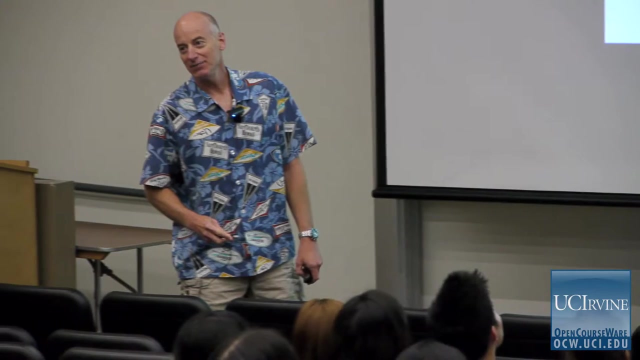 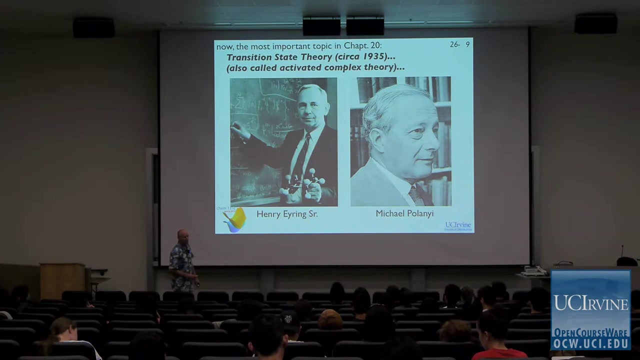 So the Texas says, okay, where are you from? Other words are sometimes substituted Okay. So I would love to spend 10 minutes talking to you about these two guys. Henry Ehring worked at the University of Utah for most of his career. one of the great American physical chemists. 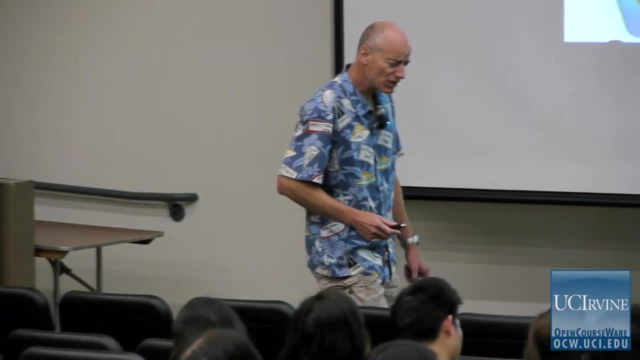 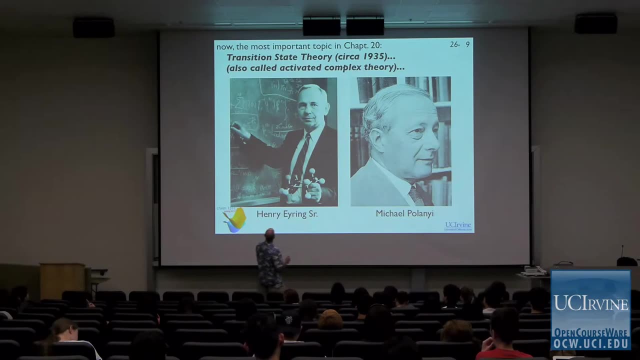 of the 20th century. Michael Polanyi, Nobel Prize winning physical chemist. All right, both of these guys are responsible for what we're going to be talking about today: transition state theory. They worked it out in the 1930's. 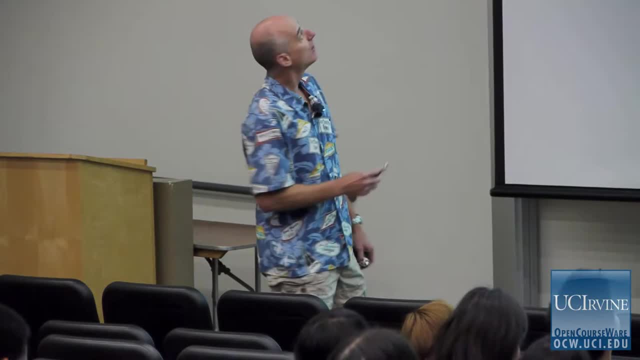 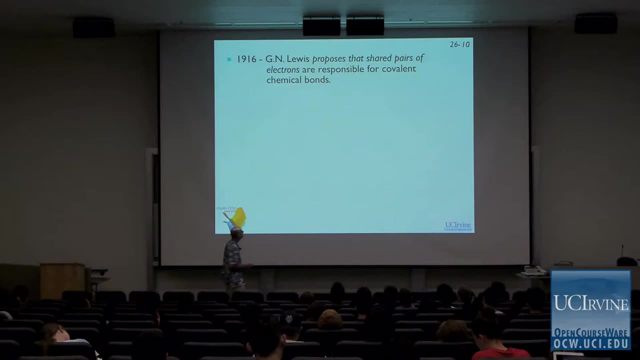 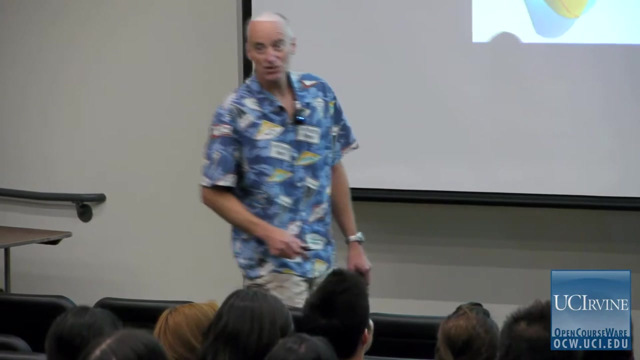 So here's the short version of the history that matters here. Way back in 1916, GN Lewis, the first great American physical chemist, worked out Lewis dot structures. All right, there was no quantum mechanics in 1916. It wasn't invented until 1924.. He came up with, I don't know, A very compelling model for chemical bonding involving pairs of electrons. that turned out to be correct and much of what it predicted, way before the fundamental underpinnings of quantum mechanics were described. He figured all that out. 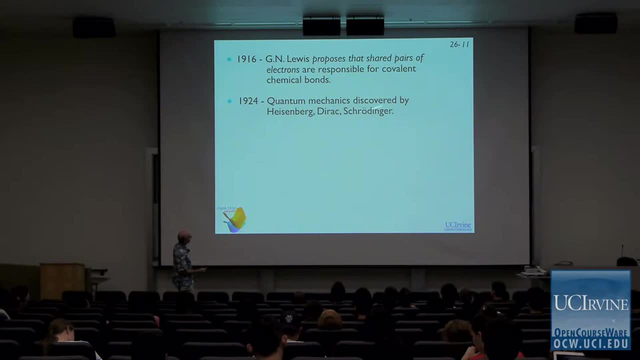 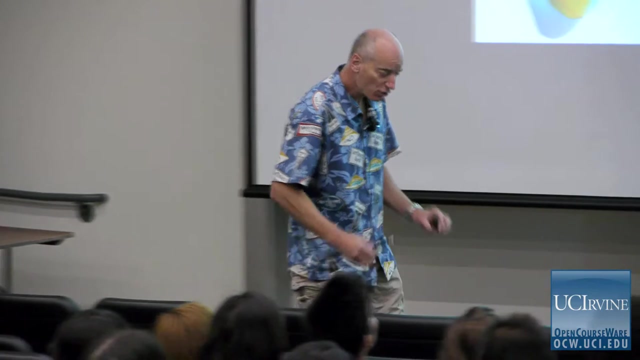 He was a genius. Heisenberg, Dirac and Schrodinger discovered quantum mechanics in 1924. A bunch of Germans- Heitler and Frit Heitler and London rather- Took quantum mechanics and applied it to bonding for the first time. 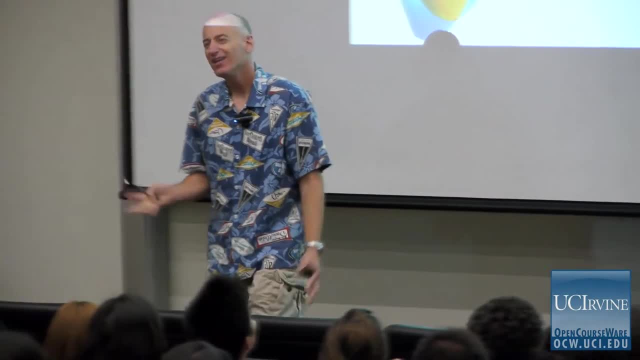 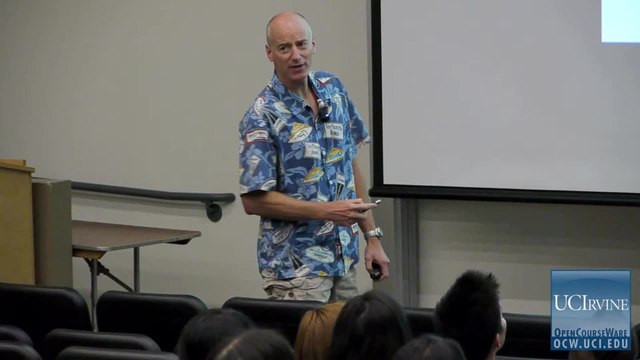 They did the first quantitative description of chemical bonding. Their names are usually lost. We hardly even mention it. Sometimes we talk about London's dispersion forces. You guys remember that? Vanderwall's forces. This is the guy, Fritz London. He's the guy who figured that out. 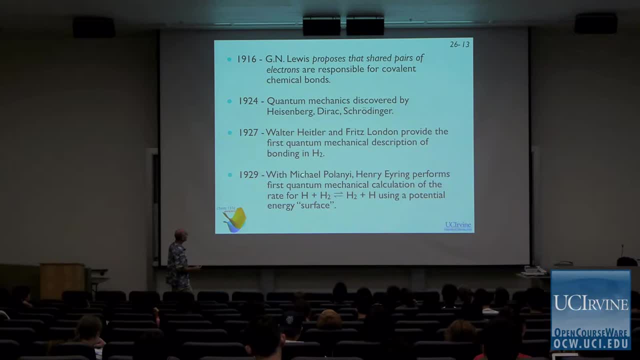 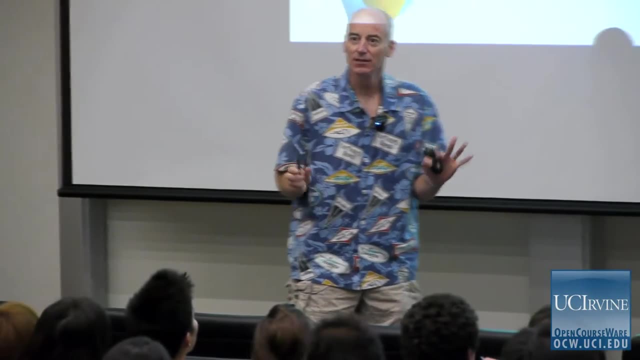 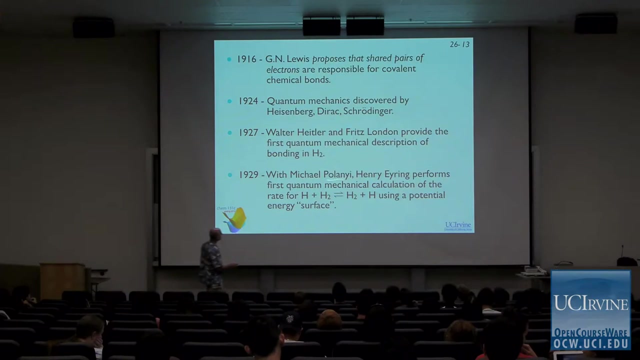 All right. 1929, five years after quantum mechanics, These guys developed a quantum mechanical way to think about reaction rates. All right, these guys figured out a quantum mechanical way to think about bonding. That's pretty important, All right. but Polanyi and Ehring figured out how to think. 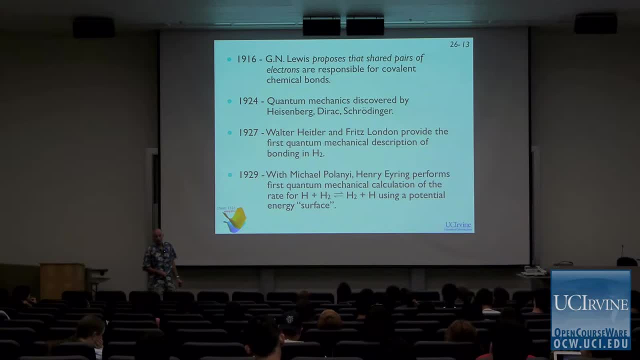 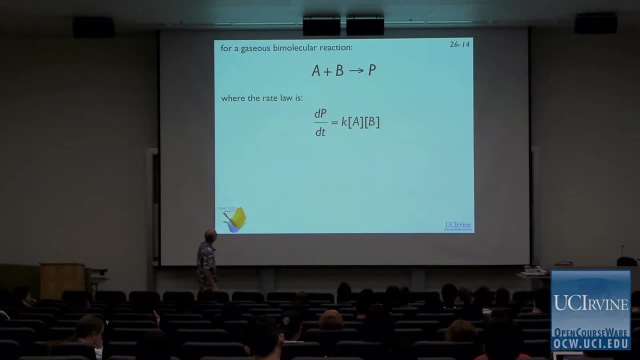 about reaction rates from a quantum mechanical perspective. All right, so we're going to zoom through what they taught us today. Here's the basic idea: A plus 1.. A plus 1.. A plus B goes to products. We're just going to talk about this generic reaction today. 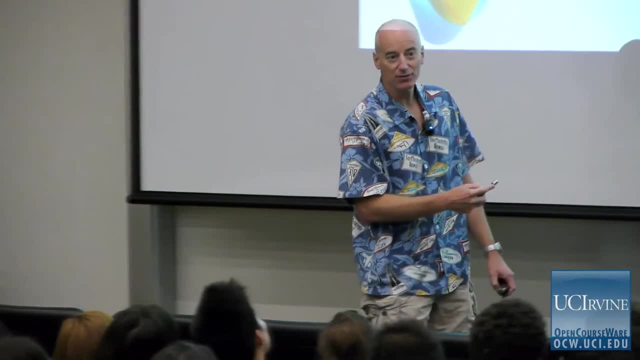 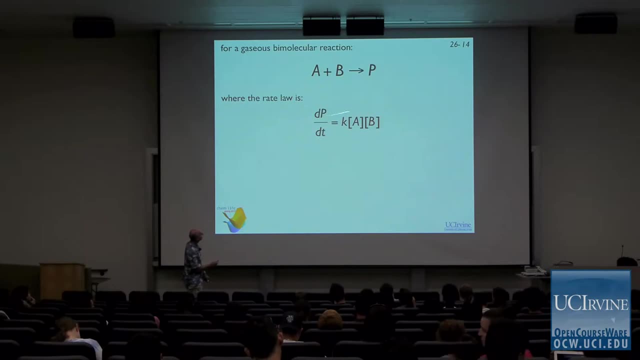 All right, we've stripped down this lecture so that we've taken everything else out. It should be three weeks worth of lectures. We know the rate law. is this? All right, the rate constant times, the concentration of A times the concentration of B- These can be pressures. 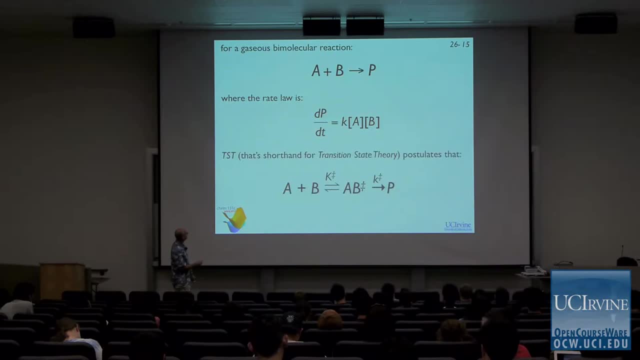 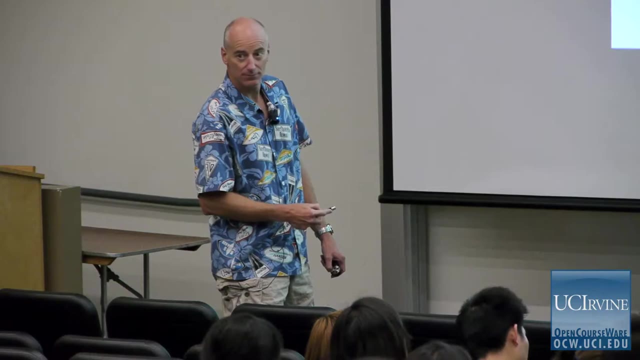 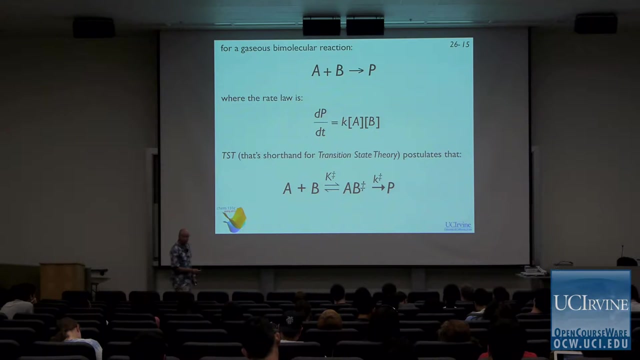 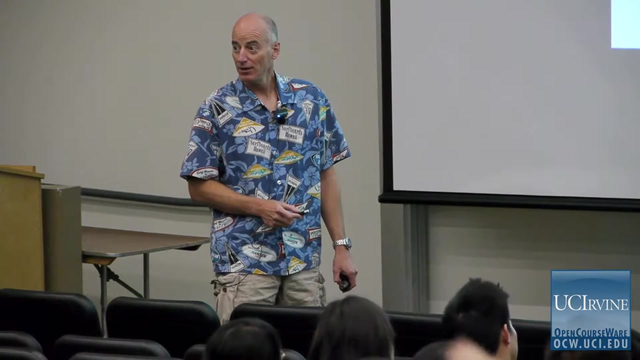 or concentrations. Transition state theory says that this reaction actually occurs through this mechanism. All right, A plus B are in equilibrium with something called AB double dagger and that reacts in a unimolecular fashion to give us products. All right. transition state theory basically takes all. 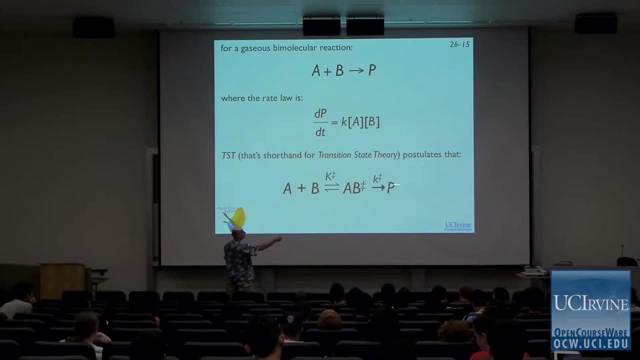 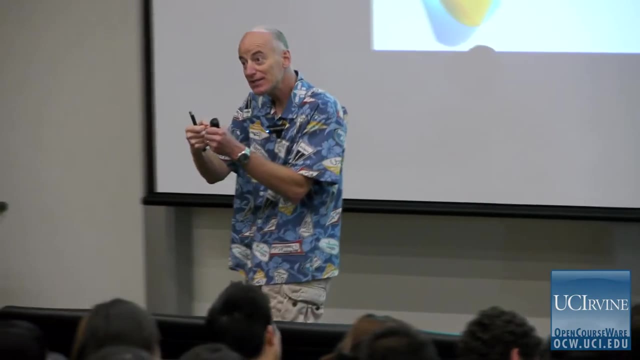 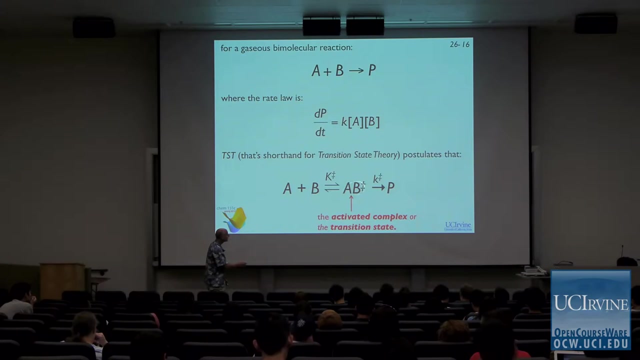 of the reactants puts them on one side, All of the products puts them on the other side, and in between it constructs something called an activated reaction, activated complex or a transition state. That's why it's called transition state theory. This thing here is the transition state. 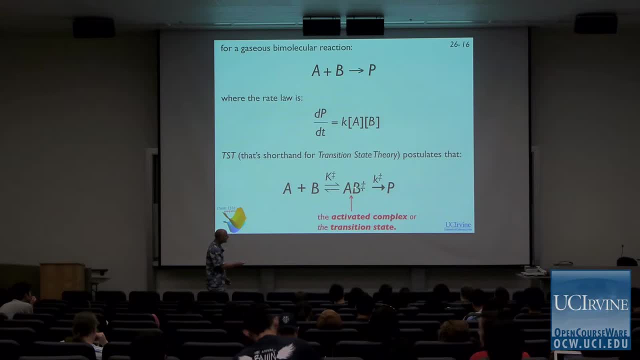 It's an entity that is intermediate between the reactants and the products. If bonds exist in the products that don't form in the reactants, they exist partially in a weak form in the activated complex or in the transition state. If bonds are broken here, they're partially broken. 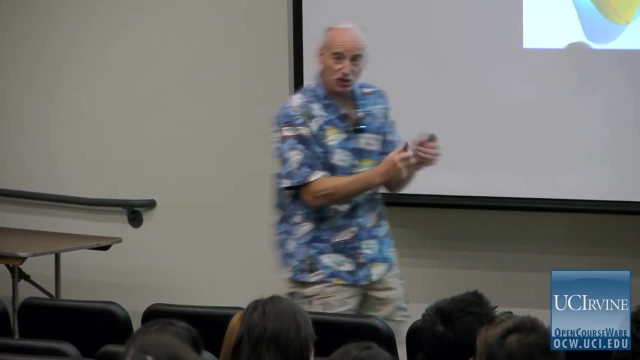 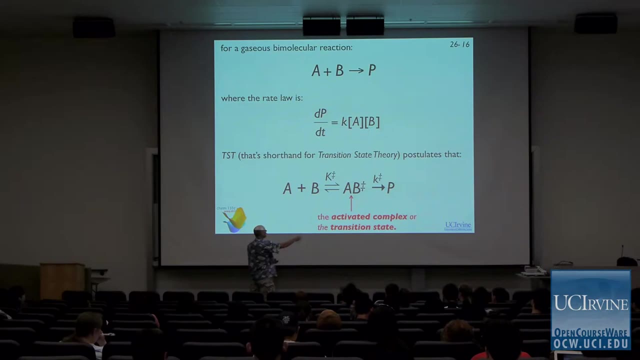 in the transition state. So the transition state has structural attributes, bond lengths and so on that are intermediate between the reactants and the products. One of the key points about transition state theory is that it postulates that an equilibrium exists between this transition state and these reactants. 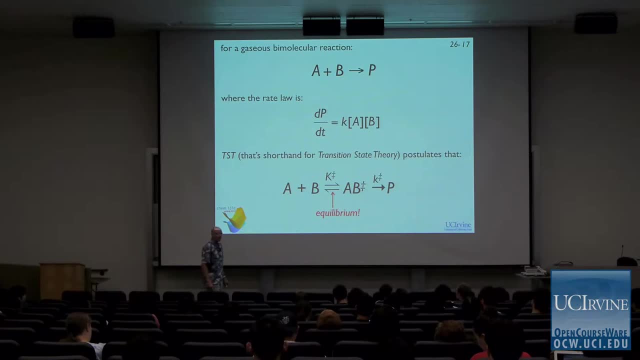 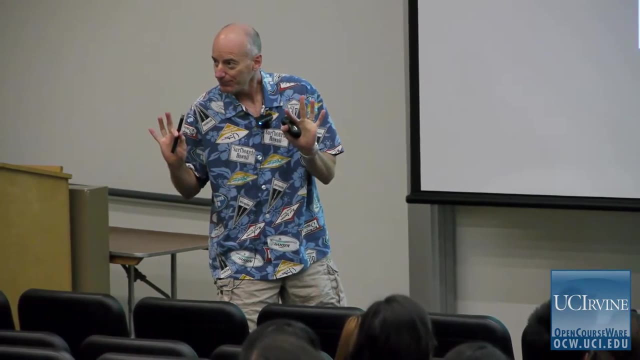 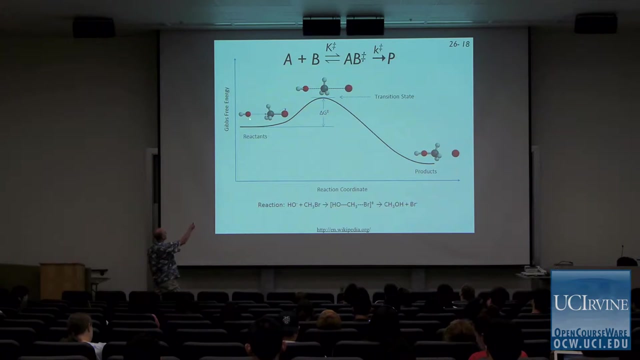 So here's the picture in terms of energy that you've seen a million times. but what we're presenting here now, the notation applies specifically to transition state theory. You've got reactants. that's represented here by these two molecules. This looks like it could be an OH, that's CH3, that's CH3BR. 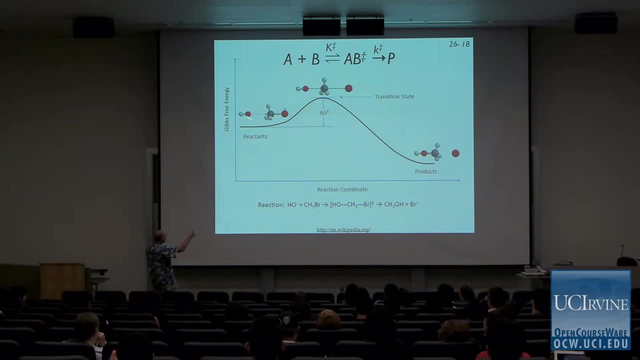 apparently OH minus CH3BR. that's the transition state and here are the products. Notice that in this reaction a new bond is formed between this oxygen and this carbon and this bond here between this carbon and this bromine is broken. So in the transition state notice. 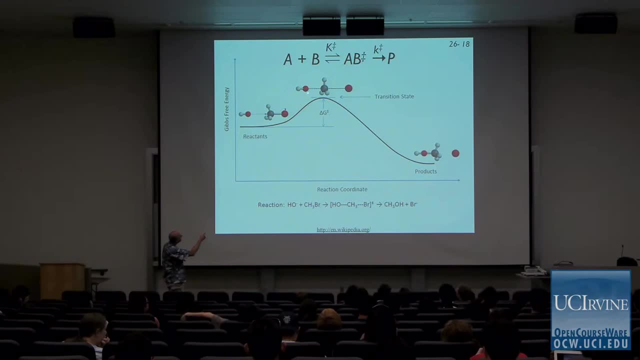 that the transition state. what we're depicting here is this bond is partially formed. You see how long it is. It's a long weak bond. and that bond is partially broken. See how long it is. It's a long weak bond also. 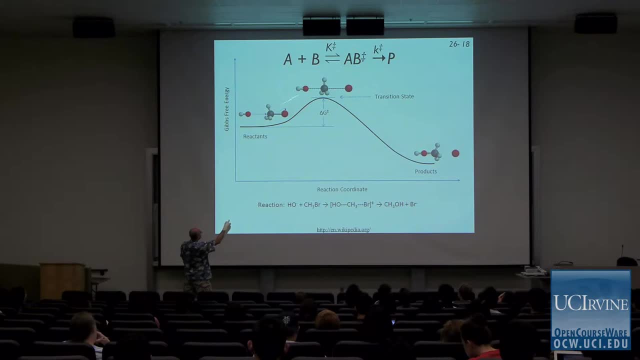 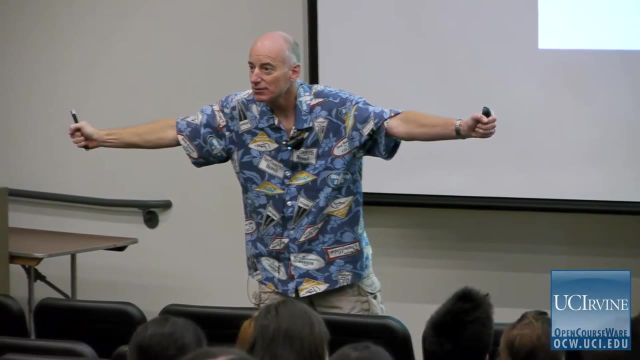 That bond is going to be broken in the product state. That bond doesn't even exist in the reactant state. so the transition state contains all of the bonds that are present in the reactants and in the products, but the bonds that are involved in the formation. 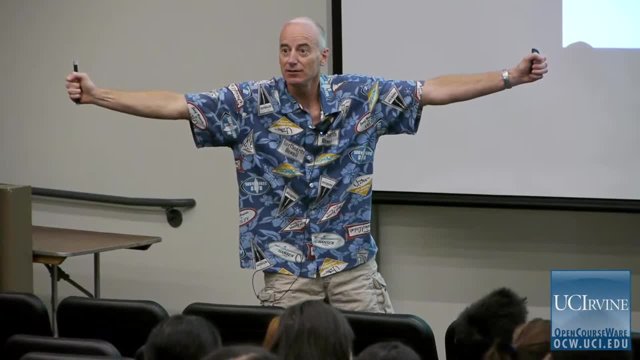 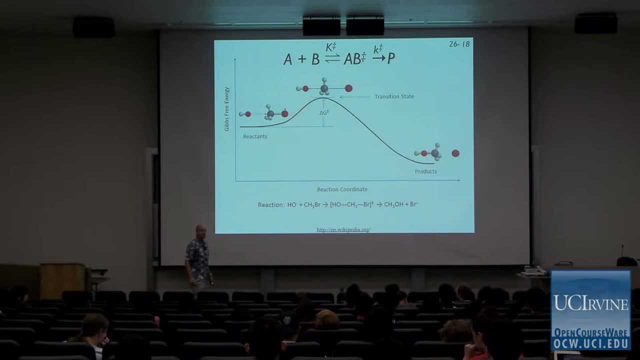 the formation of the products from the reactants are weakened. See how long that is. see how long that bond is. These are two super weak bonds. So we can construct a transition state by thinking about what the products look like, what the reactants look like: products, reactants. 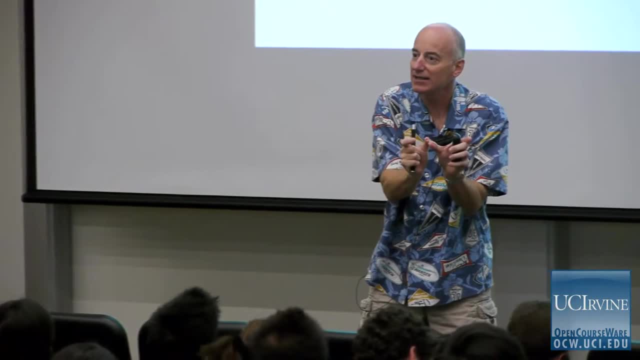 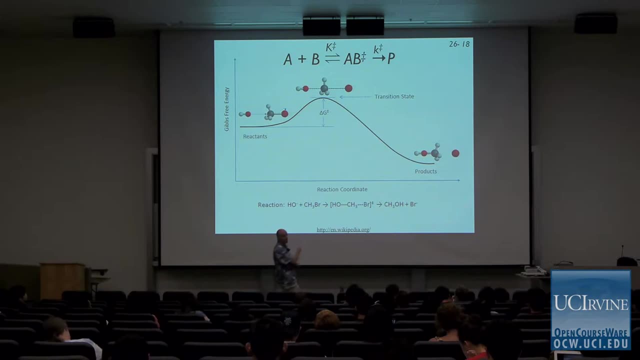 and then thinking about how the products are formed from the reactants geometrically. How does that happen? This shows that the reactants are formed from the reactants. This shows an attack in a particular geometric orientation of the OH minus to the CH3BR. 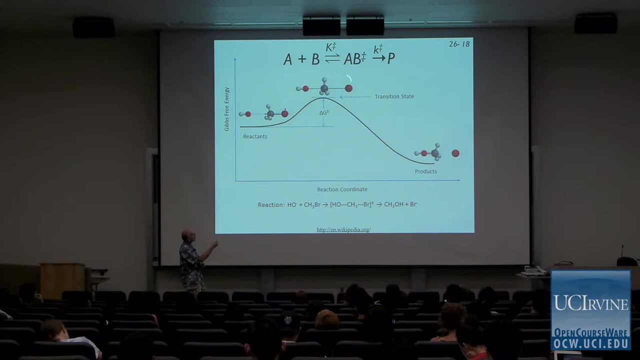 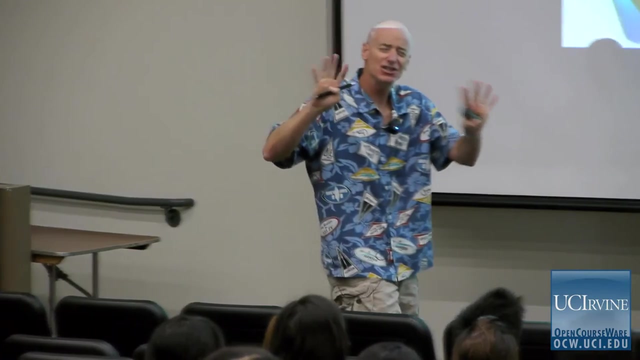 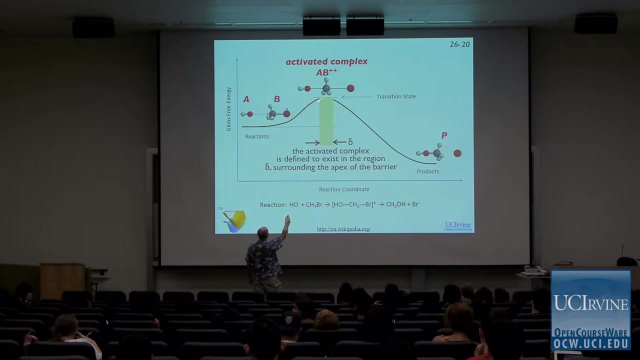 Thinking about this and thinking about this, we can construct what this transition state should look like using a few simple rules. Okay, now it turns out that transition state and activated complex should not technically be used interchangeably. There's a nuance. The activated complex actually exists over a range. 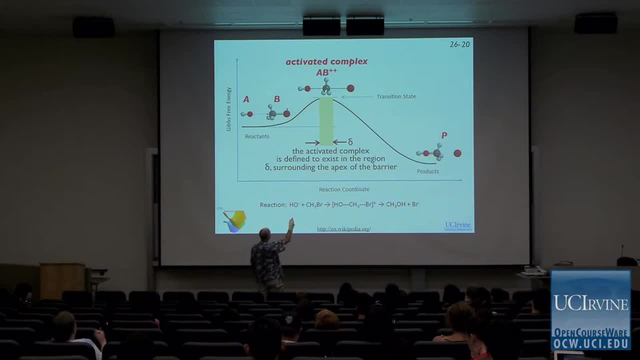 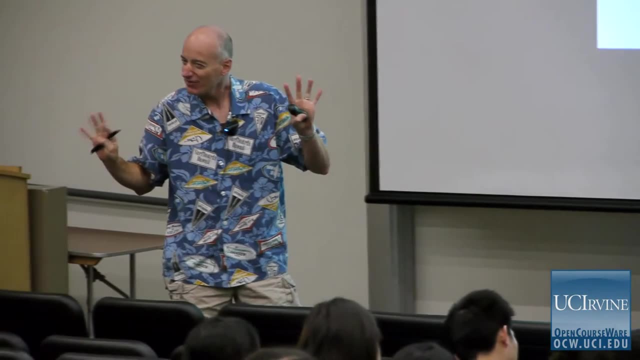 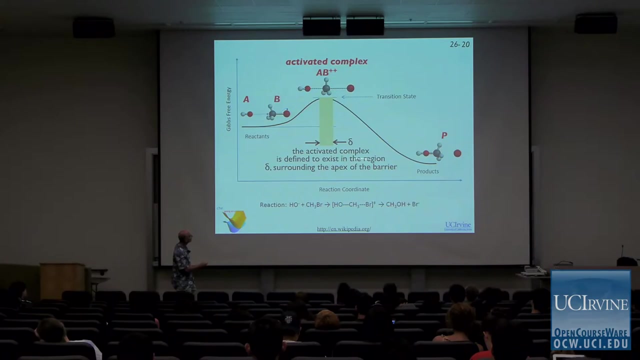 of this reaction coordinate, whereas the transition state in principle exists only at a particular point in time. We're not going to bother ourselves with that distinction today. There's a fine point there that you should know. These are not identical, They are not interchangeable. to say, activated complex. 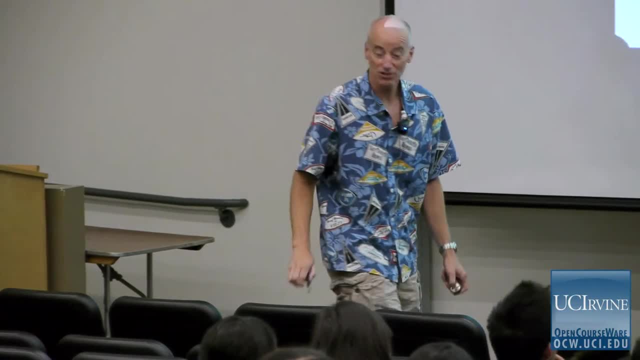 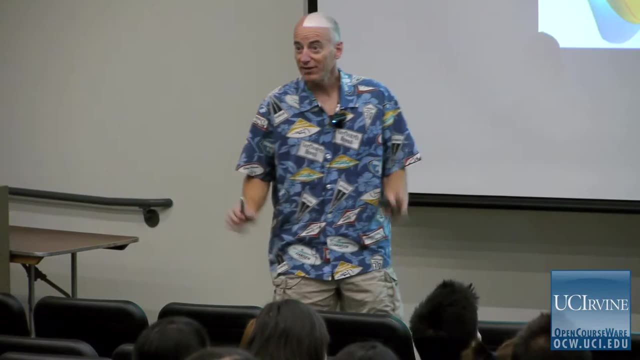 and transition state, but today we're just going to use those two terms interchangeably. Okay, Now we're going to look at the reaction state. Now, with that as a premise, let's see if we can work out what the reaction rate is. 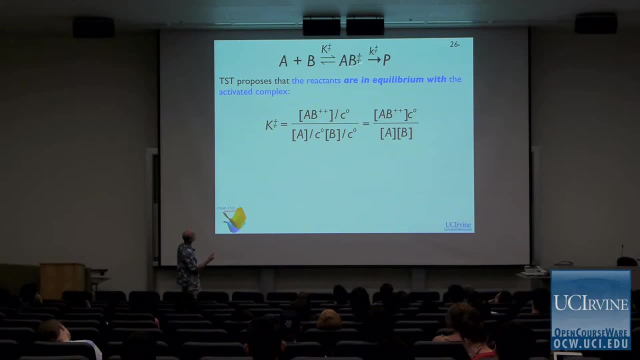 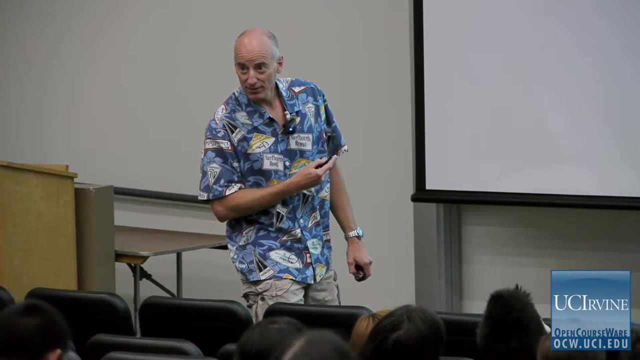 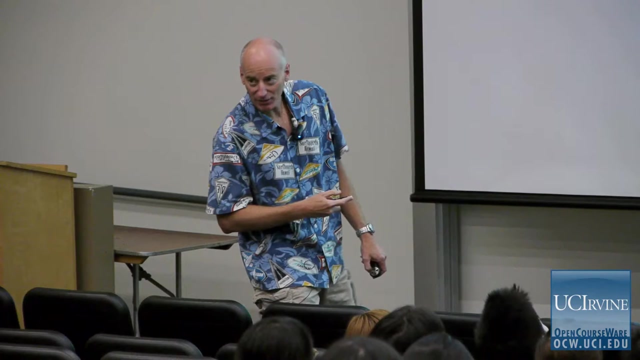 Here's our mechanism, our transition state theory mechanism for this reaction Transition state. yes, so we can write an expression for this equilibrium constant. What is it? Product over reactants. Notice that I'm normalizing and being very careful here to write activities. 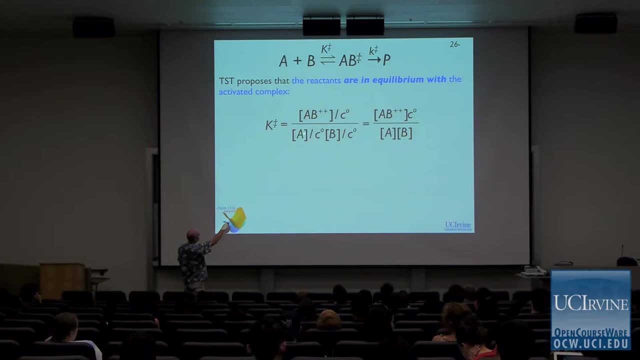 The activity of the transition state, the activity of A, the activity of B, because I'm dividing by the standard concentration here. Okay, and so when we're done canceling these C zeroes, I end up with an extra factor of C zero in the numerator. 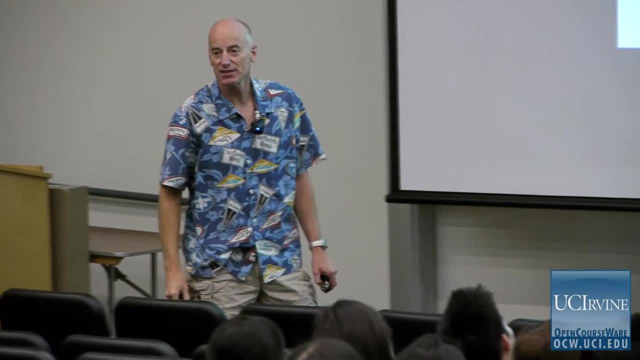 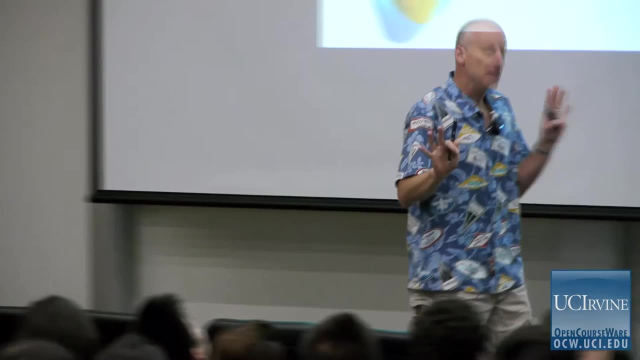 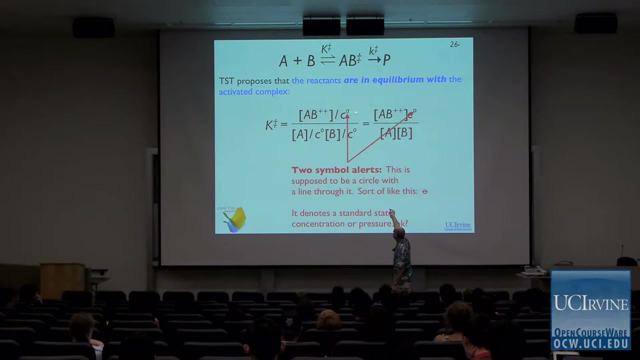 That ensures that the equilibrium constant is dimensionless, doesn't it All right? Now, unfortunately, I used the Microsoft Word equation editor to write a lot of these equations. It does not allow me to write a zero with a line through it. 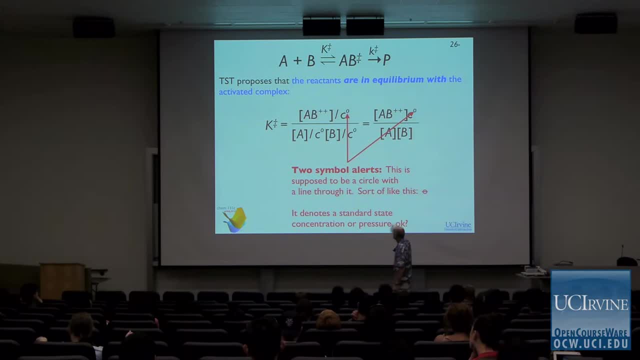 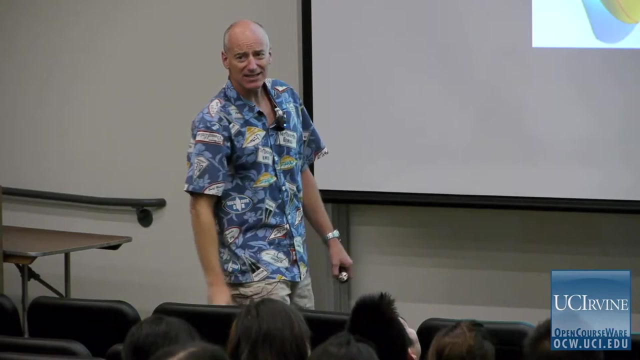 All right, That is the symbol for the standard concentration, one molar, for example, but I'm just going to call it C zero. All right, there's another issue. See this double X here. this double plus Microsoft equation editor doesn't contain a diesis. 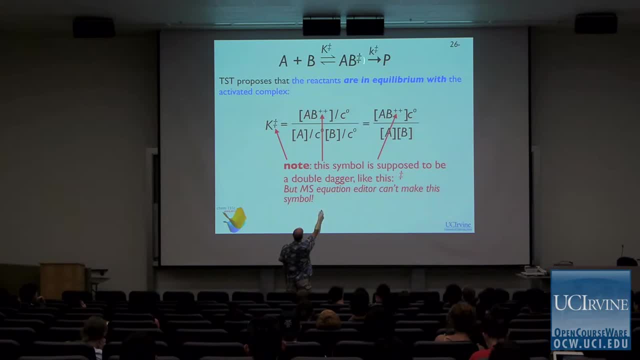 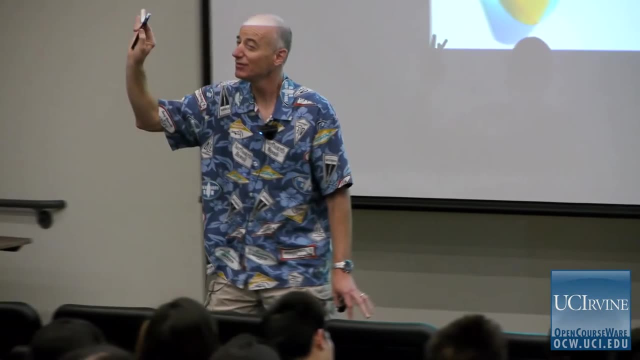 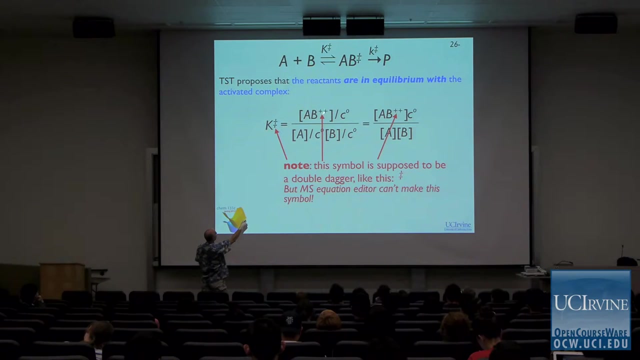 What's a diesis? It's that thing. the double dagger. The double dagger is the same thing as the diesis. So when I write two pluses, I'm just indicating the transition state. Okay, So that refers to the transition state. 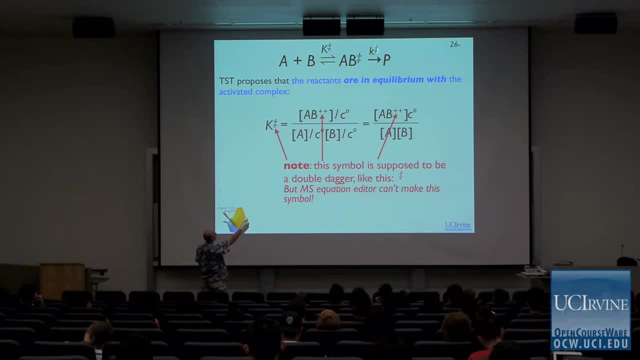 That's the equilibrium constant. that involves the transition state. That's the unimolecular reaction rate constant. that involves the transition state. You see how I'm going to write that as that. If you see the double plus, that's the transition state. 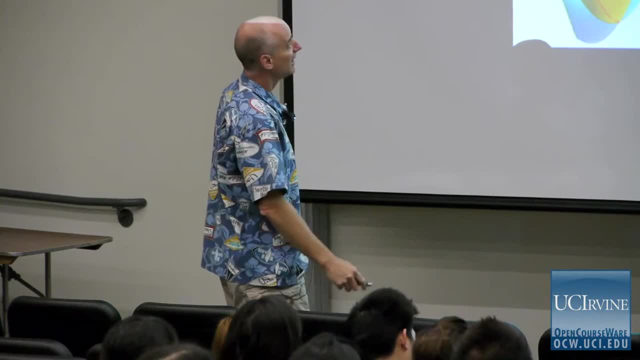 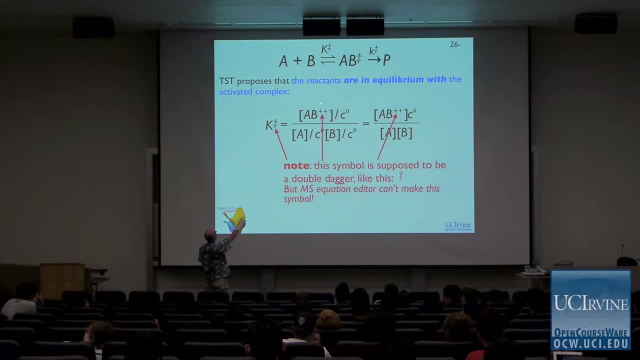 If you see the plus, it's just the diesis. If you can, if anybody knows a work around for that, I would. that would help me out a lot. If I, how do I write a diesis in Microsoft equation editor? 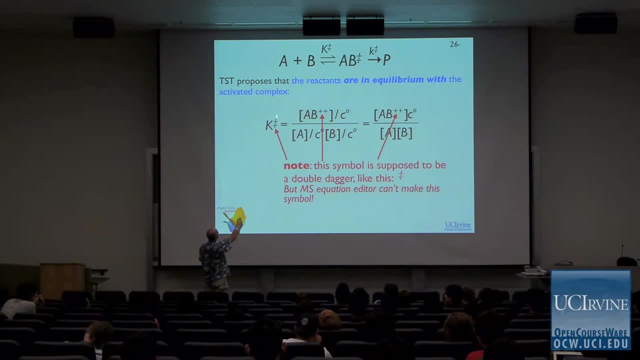 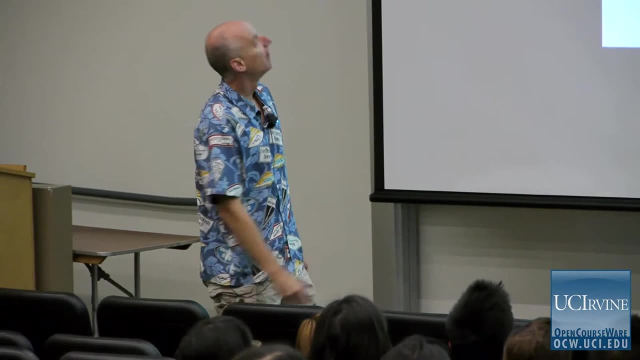 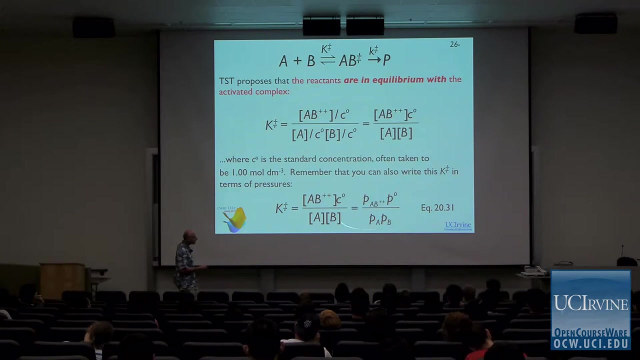 Here I cheated, I put a white square here and I pasted this on top and I thought I can't do that. There's like 106 slides in this presentation. Okay, Now it says yes. yes, We could write this in terms of pressures, if we want to. 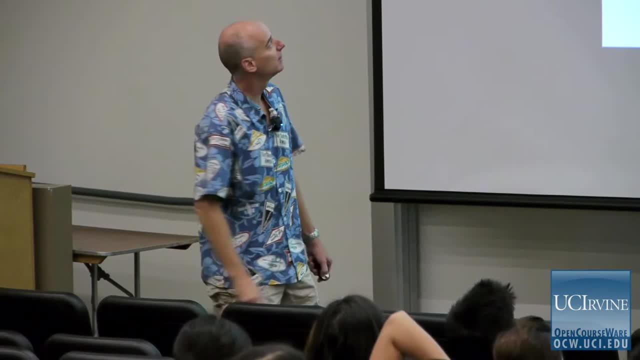 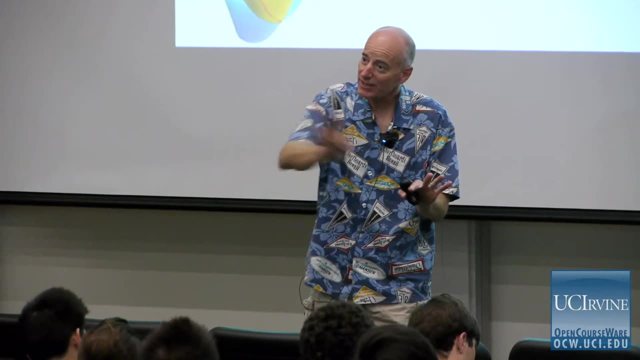 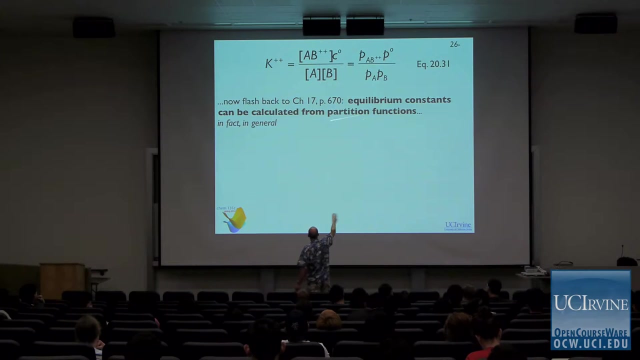 All right, Here's the concentration, Here's pressures, No difference. Now, if we flashback, we're talking right now about chapter 20.. If we flashback to chapter 17, it turns out we can calculate equilibrium constants from partition functions. 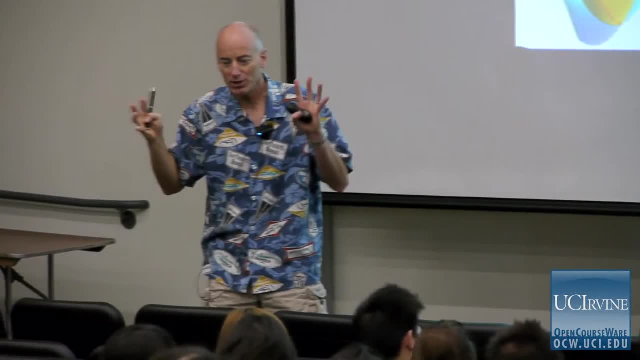 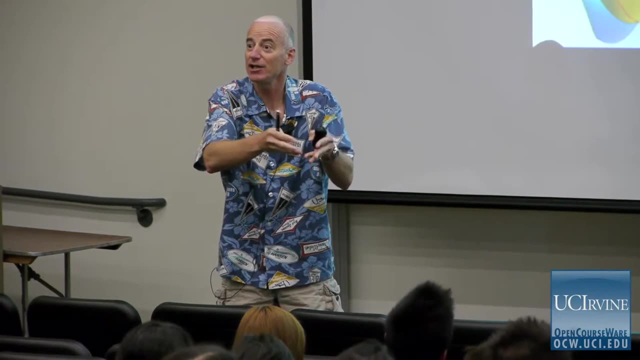 All right And recall. partition functions are very important to us because they allow us to make a connection between statistical mechanics and thermodynamics. Partition functions contain information about the actual molecule. We can look at a molecule If we know something about its state distribution. 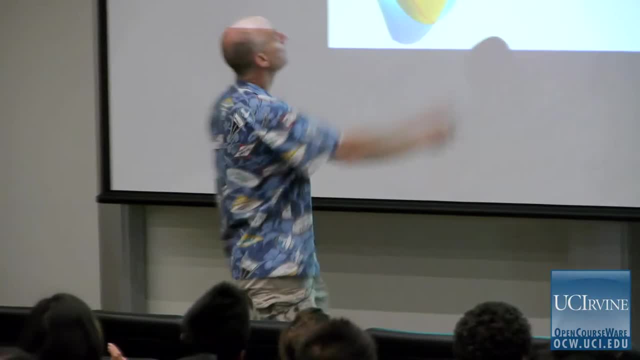 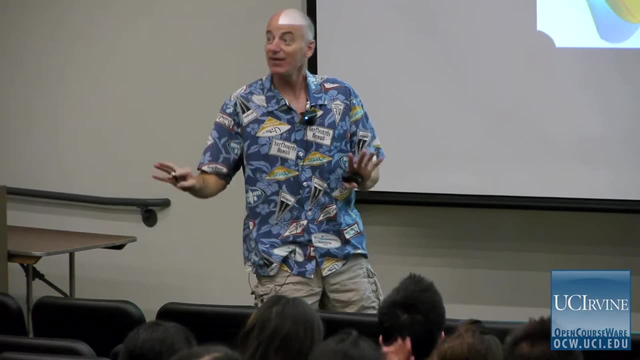 we can write its partition function. All right. What we learn in chapter 17, what we didn't have time to talk about in the class this quarter is the fact that you can also use these partition functions to calculate equilibrium constants. If you want to read more about that, it's on page 670.. 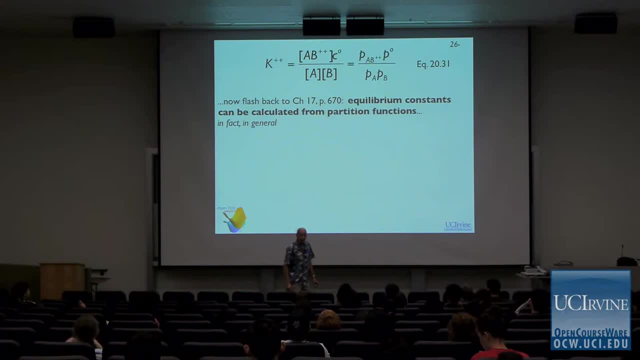 Turns out to be a sort of an important thing that we left out. Okay, So let's look at this. Here's what's there. all right, Here's some generic reaction: A moles of A. B moles of B. 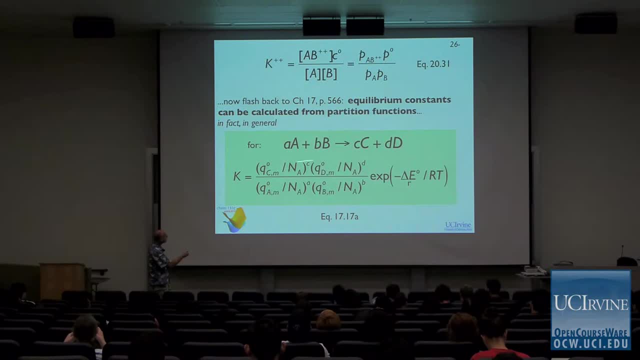 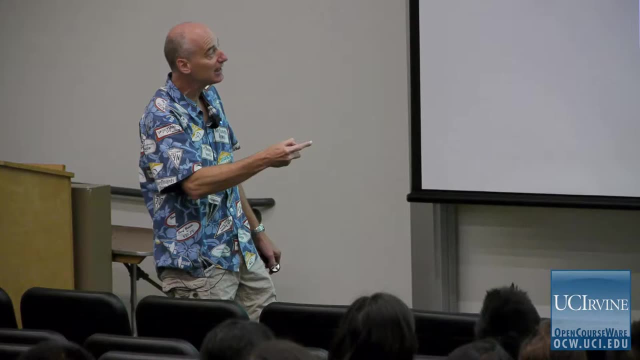 C moles of C, D moles of D. Here's what the equilibrium constant expression looks like, written out in terms of the standard molar partition functions for A, B, C and D. All right, So if I can calculate these partition functions for all, 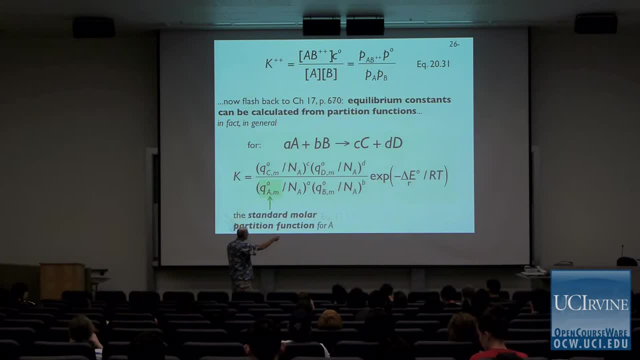 of these guys, and I know that. so what is this? This is the standard Molar partition. M means molar A is species A. What's that? That's Avogadro's number. That's not a misprint. 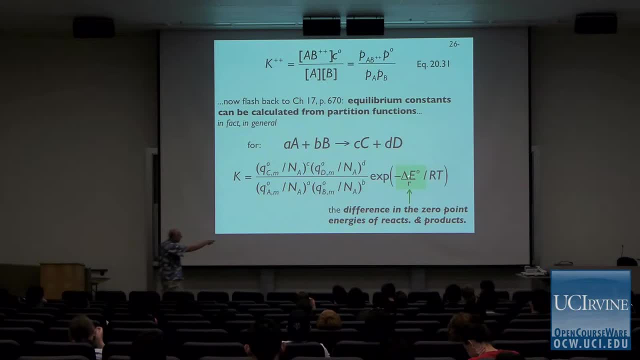 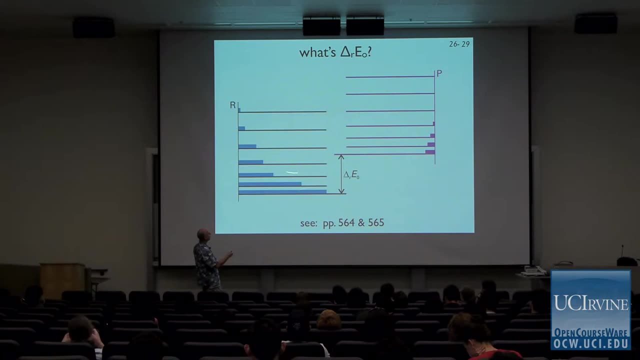 All right, It's Avogadro's number. in every single case, That is the difference in the zero point energies between reactants and products. So if this is your generic reactant, here here are vibrational energy levels. Here are vibrational energy levels of the product. 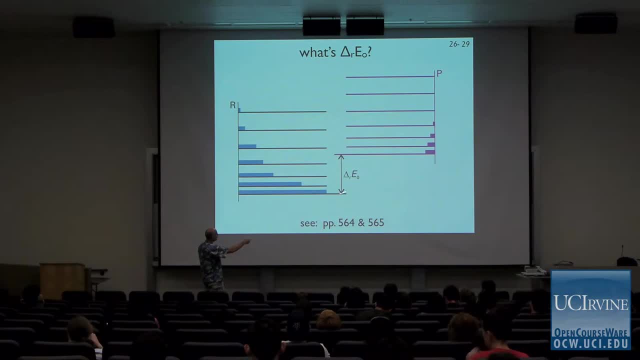 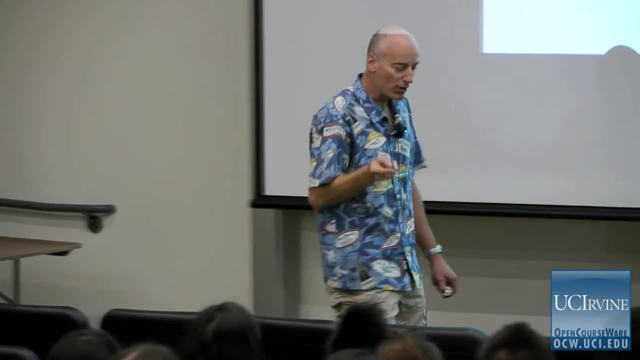 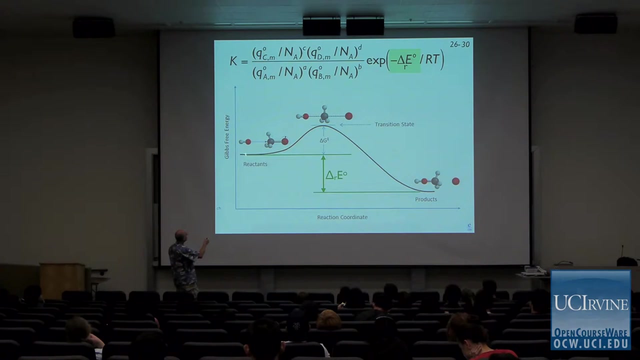 All right, That's the ground vibrational energy level. That's the ground vibrational energy level. That's delta, R E, zero. All right, The difference between the ground, the zero point energies of the reactants and the products. Okay, So here's our Gibbs: free energy as a function. 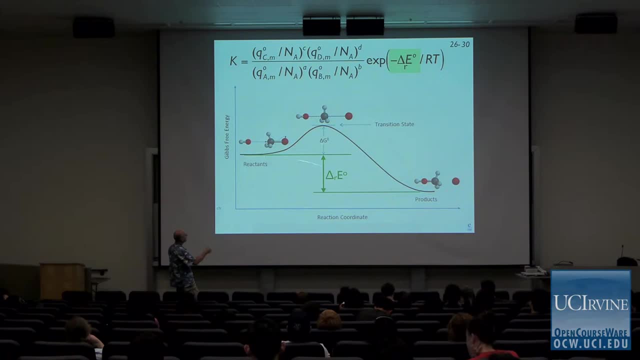 of reaction coordinate. All right, The delta R, E zero is closely related to this green quantity that I'm indicating here. All right, If this thing was in its ground vibrational energy level, and this thing was in its ground vibrational energy level. 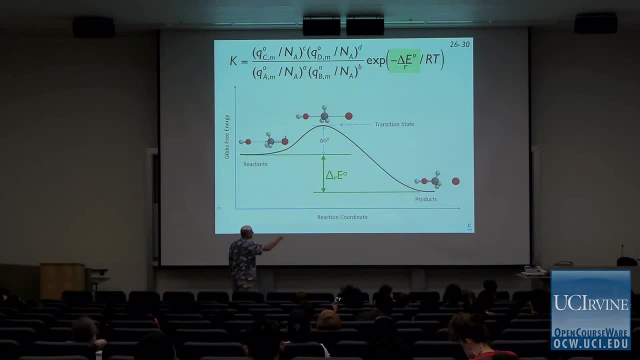 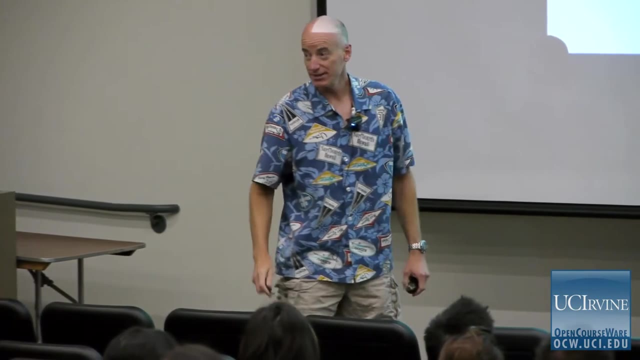 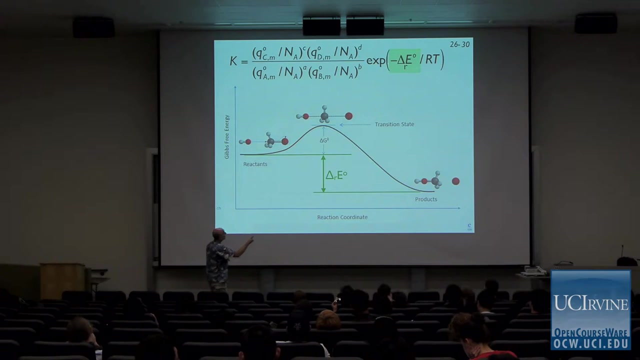 both of these guys and both of these guys, then this would be delta, R E zero. All right, Because we're always talking about the zero point, energies And we could say something about this equilibrium constant. We could calculate it using this equation, right here: 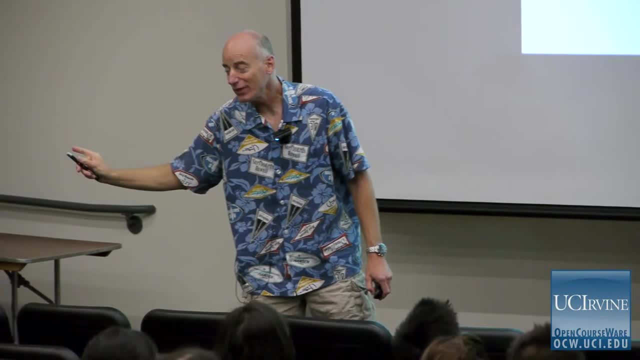 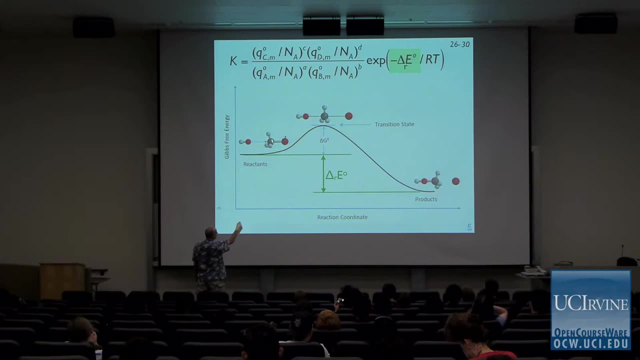 Now, in transition state theory, that's not the equilibrium constant We care about. What we say in transition state theory is: this is an equilibrium with this. All right, I don't care about the equilibrium of this with this. That's going to give me the normal equilibrium constant. 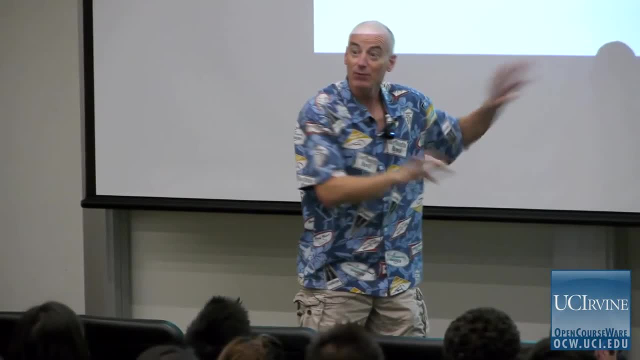 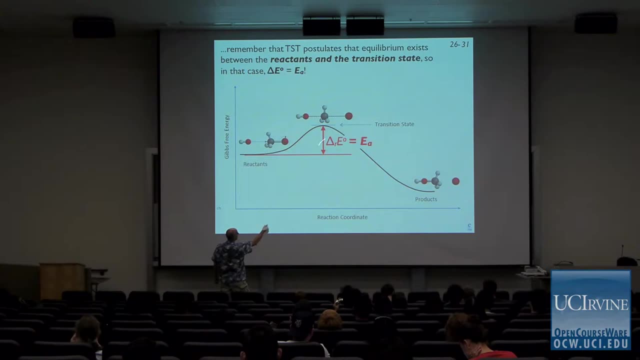 that I can learn about in chapter 17.. All right, But what transition state theory says is: these two guys are in equilibrium with one another. So what matters is this: delta, R E, zero here. All right, This thing that we normally call the activation energy. 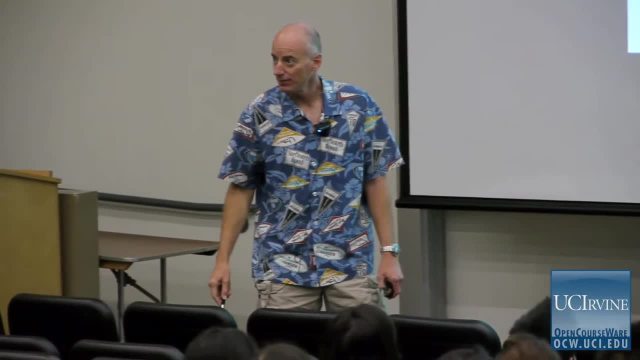 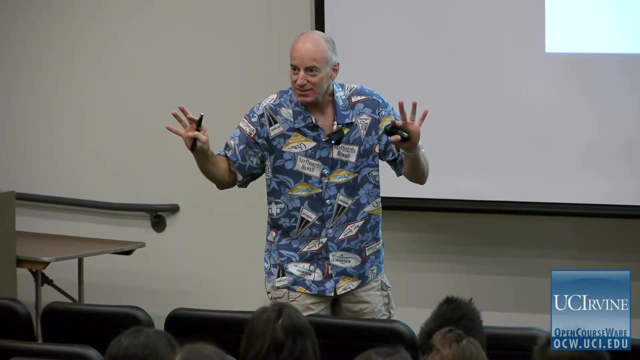 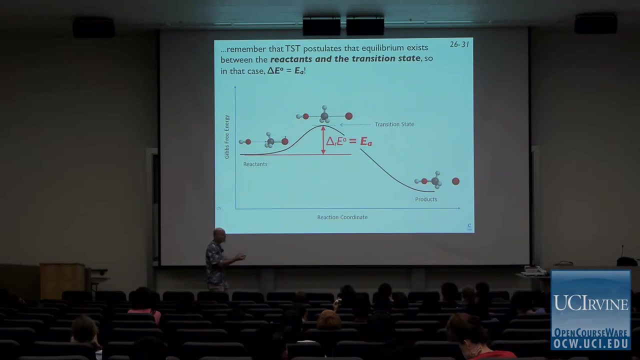 It's the activation energy from the Arrhenius equation. All right, So we want to calculate that imaginary equilibrium constant. All right, Because these things may actually be in equilibrium, but this thing is not really observable except using some exotic spectroscopic: nanosecond, picosecond spectroscopy. 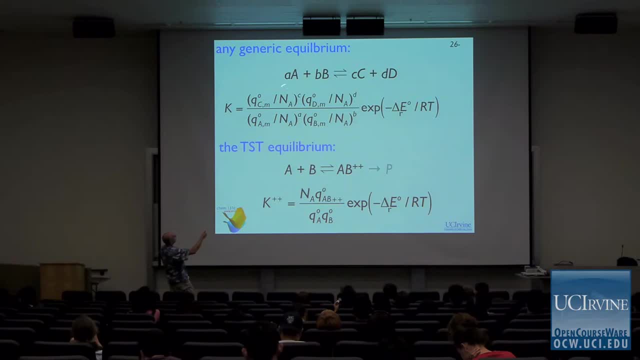 Okay, So a normal equilibrium applied to this generic reaction. right here I could calculate the equilibrium constant using this equation. So now I'm going to apply that same thinking to the transition state theory. Here's the transition state equilibrium we care about. 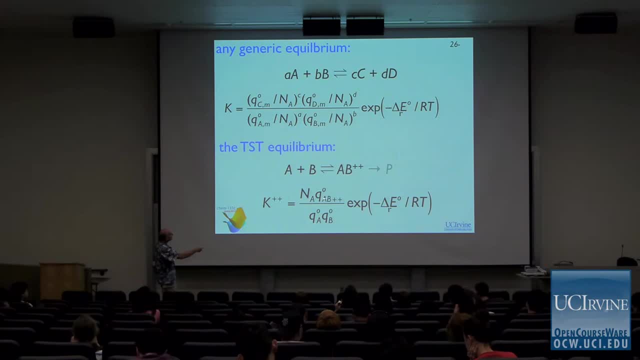 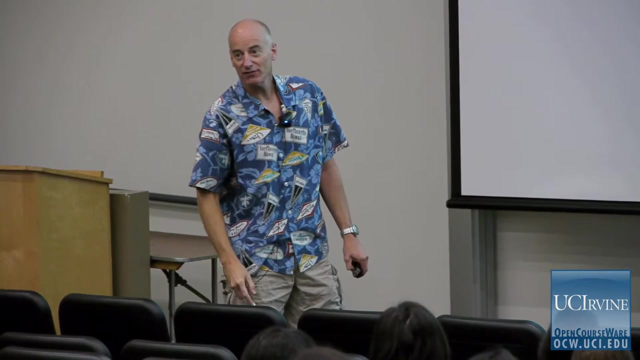 A reacts with B to give this transition state. And so now, what do I want? I want to put the partition function for that guy in the numerator, for these guys in the denominator, and then that's Avogadro's number. That's just left over from. that's an extra factor. 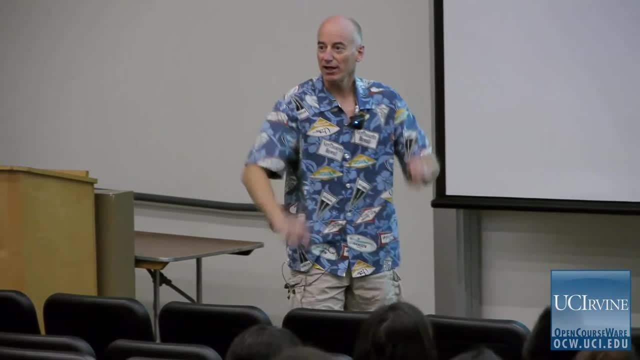 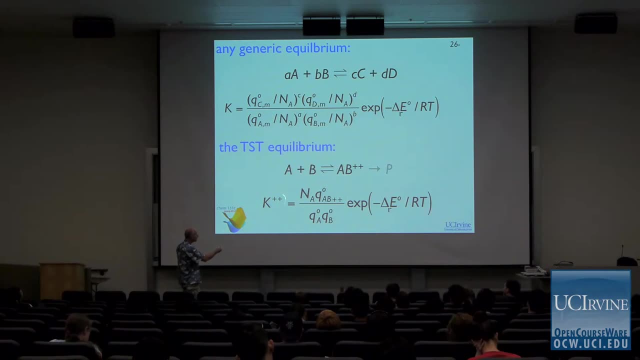 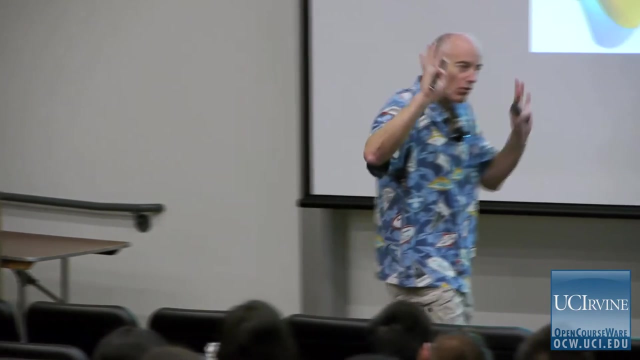 of Avogadro's number, because I've got two reactants in one product. Okay, So I can calculate this equilibrium constant that applies to the formation of the transition state. All right, Now keep in mind: everything we're talking about here is kinetics. 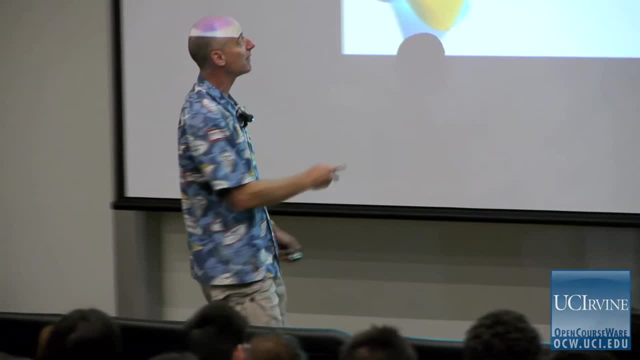 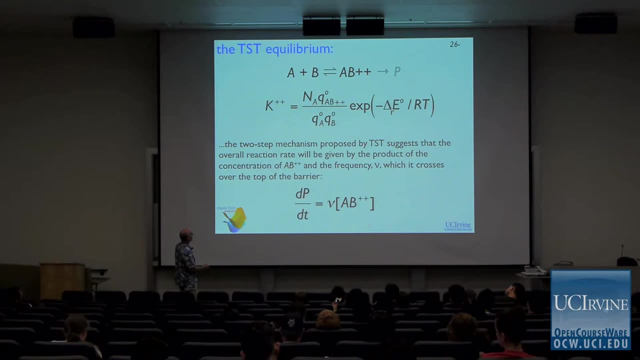 All right, We're sort of mixing thermodynamics with kinetics. They took a thermodynamic concept- equilibrium constant- and applied that to transition state theory. Okay, So you with me. so far We've got an equilibrium constant here. We can calculate it using statistical math. Okay, So we've got an equilibrium constant here. We can calculate it using statistical math. Okay So, we've got an equilibrium constant here, We can calculate it using statistical math. Okay So, we've got an equilibrium constant here. We can calculate it using statistical math. 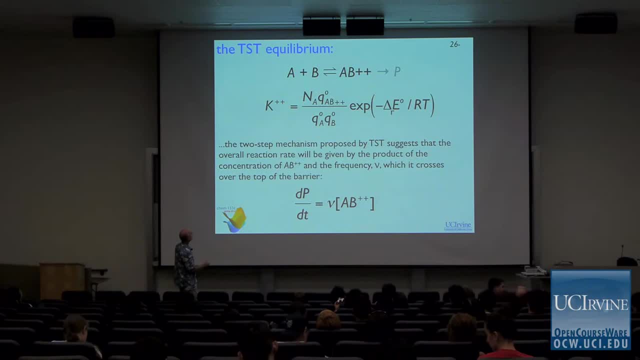 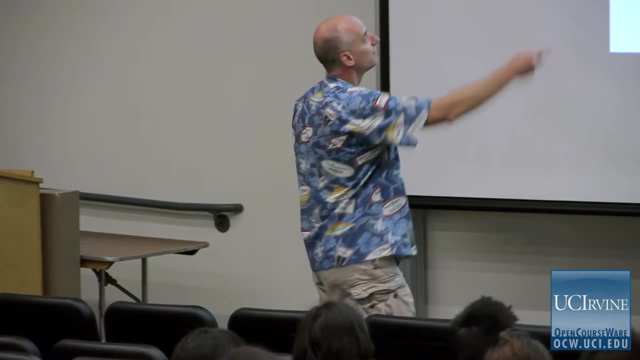 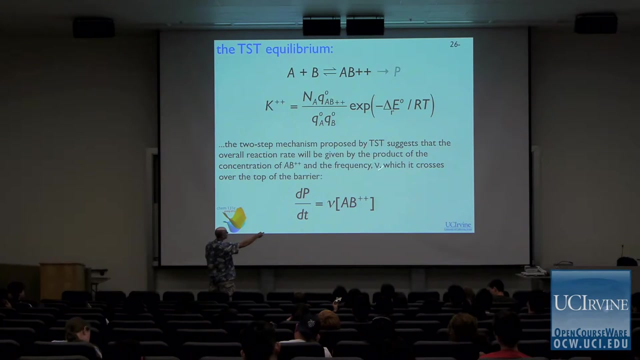 Two-step mechanism. Okay, That's the first thing to understand. Okay, That's the first thing to understand, Right? The second thing to understand is that this rate right here, shown in gray, that's going to be approximately equal to the frequency. 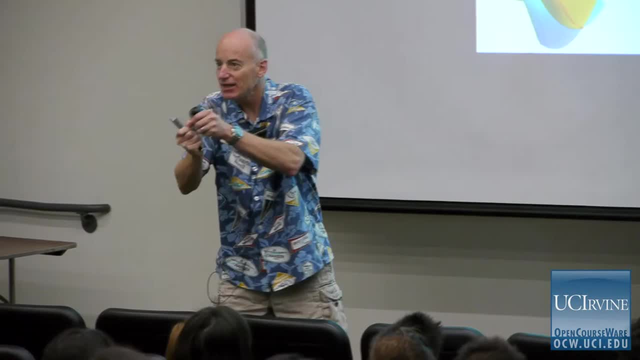 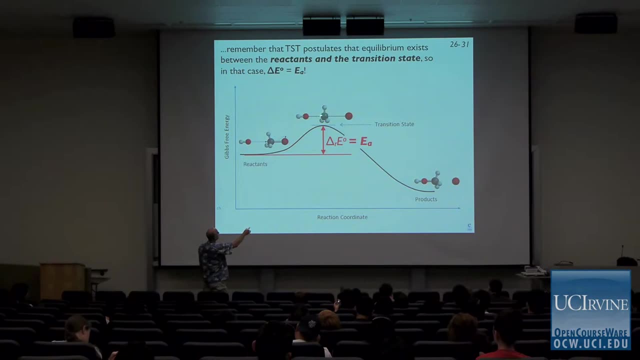 with which the transition state crosses over the top of the barrier. We've got a barrier here. We've got a transition state, This we are moving along, this reaction coordinate from reactants to products, The frequency with which this thing moves across the top. 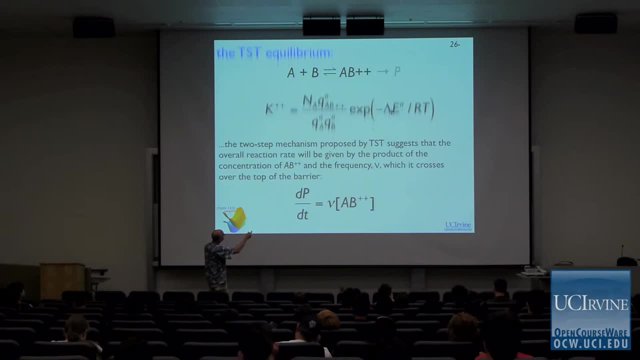 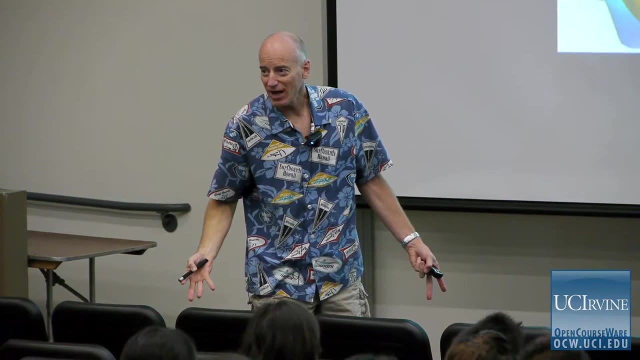 of this barrier that's going to closely approximate this rate Right, The rate at which products are formed. That seems to be a statement of the obvious. All right, Obviously, as you cross over this barrier from reactants to products, the frequency that that happens, 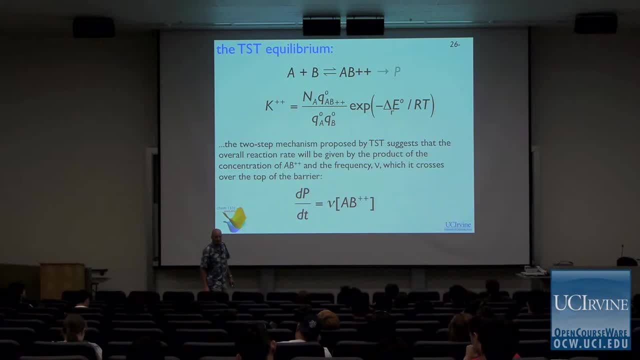 that's the rate of this reaction. I mean, it's totally obvious, Totally obvious to say that. Okay, So the reaction rate I can write as this frequency times whatever the concentration of this transition state is All right, We're going to talk about this frequency. 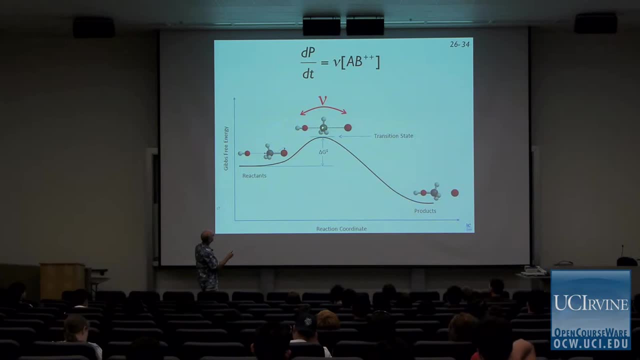 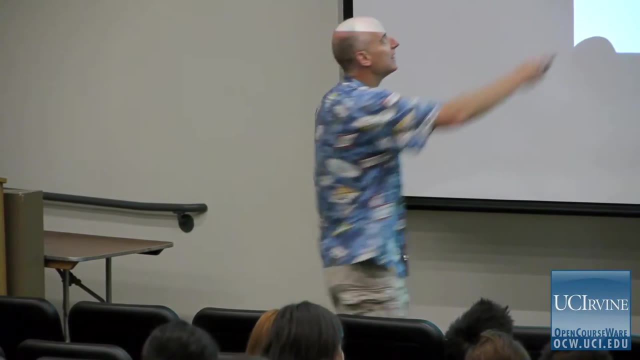 All right, It's the frequency with which- if you think about this as being a molecule, all right, there's a vibration that has to happen here. All right, This guy moves back and forth between these two, These two guys. All right. 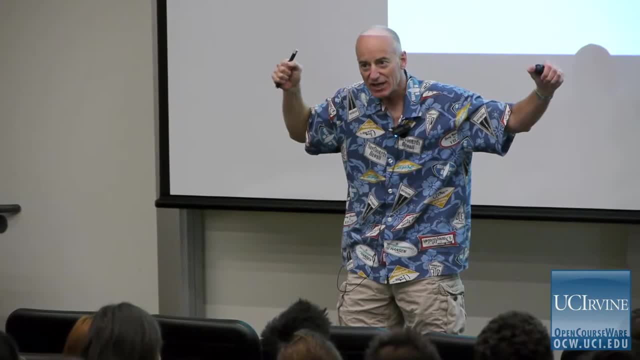 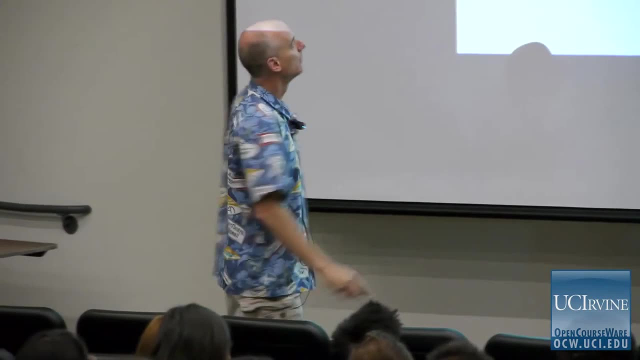 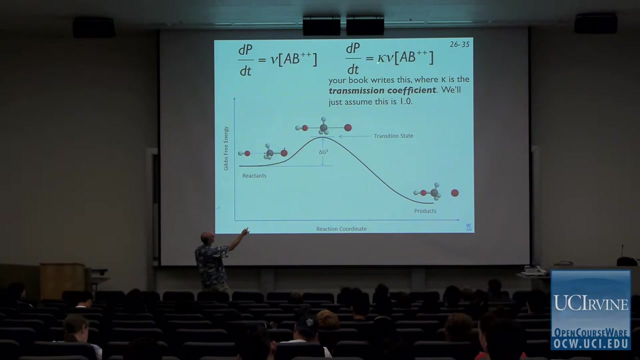 We get a symmetric vibration of this transition state. The frequency that characterizes that mode is the frequency that we care about Now. your book includes something called a transmission coefficient. We're just going to assume that's one. See that Kappa right there. 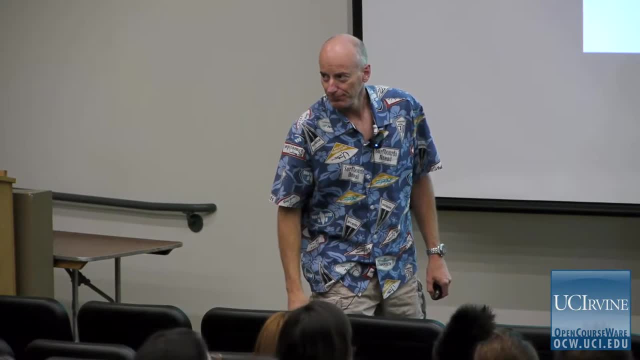 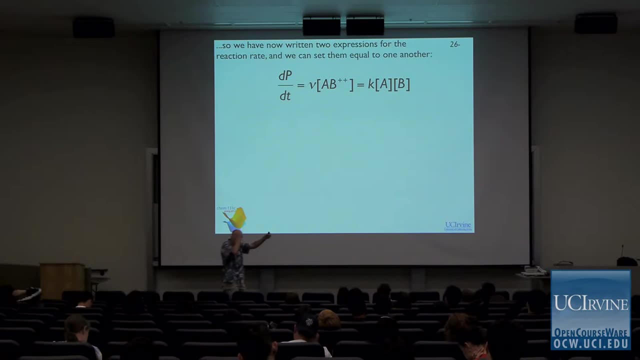 Just forget about it, It's one. Okay. So the rate of the reactions given by this special frequency. that applies to the reaction coordinate times, the concentration of the transition state. but we know we can also write the rate in the normal way with a rate constant times A, times B. 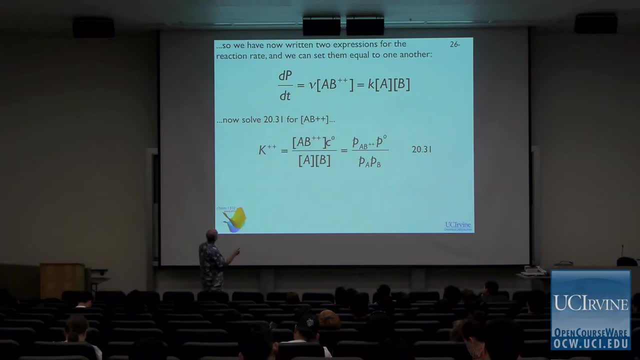 Right, It's what we've been saying all along, So we can. here was our equilibrium constant expression for the transition state, and if I just solve for AB in this expression, right here I get this and I can plug that in to AB there. 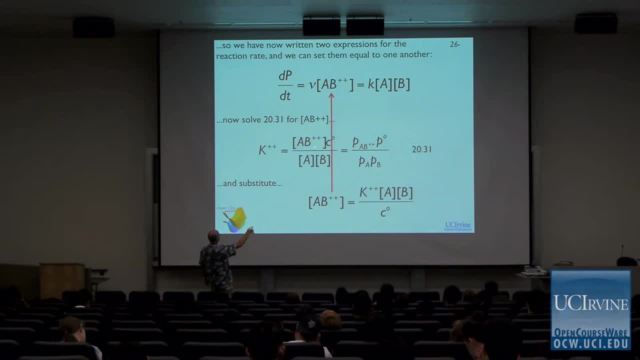 All right, So I've just solved for the concentration of the transition state from here. Okay, And now I'm going to plug that in to this equation right here, and so I'm going to put all of this into here, and so there it is. 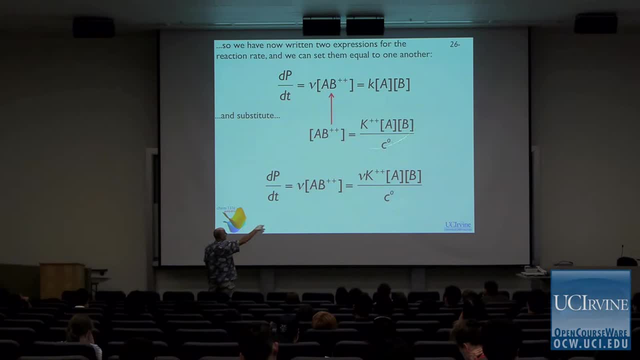 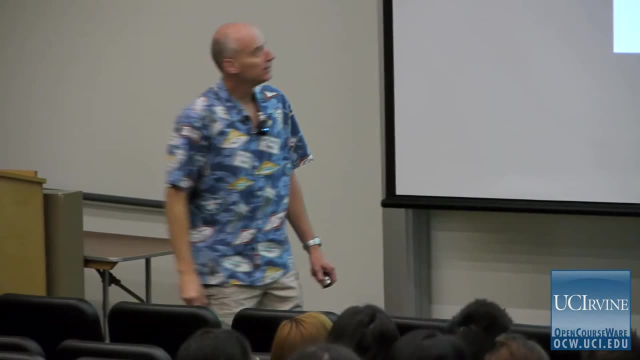 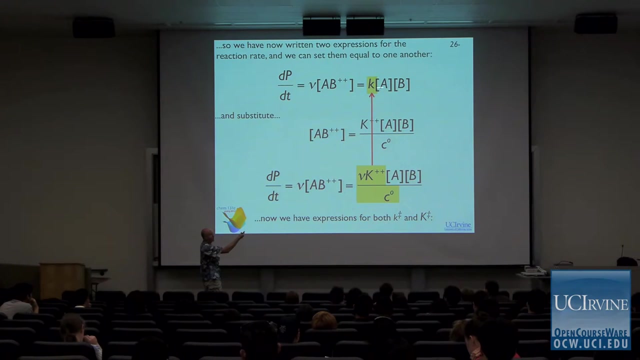 There's the V, There's the frequency, the special frequency, here's all the rest of that. All right, That's our reaction rate. So, in essence, this is the phenomenological rate expression that we would normally write for this reaction. 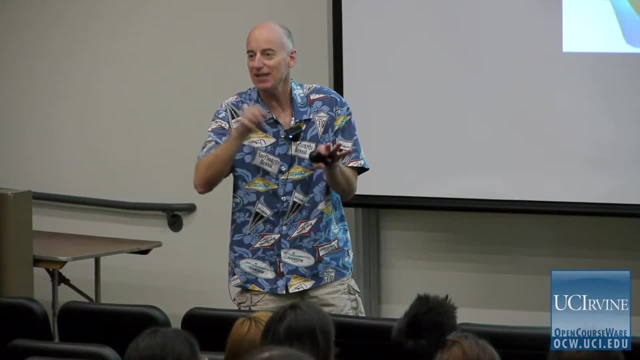 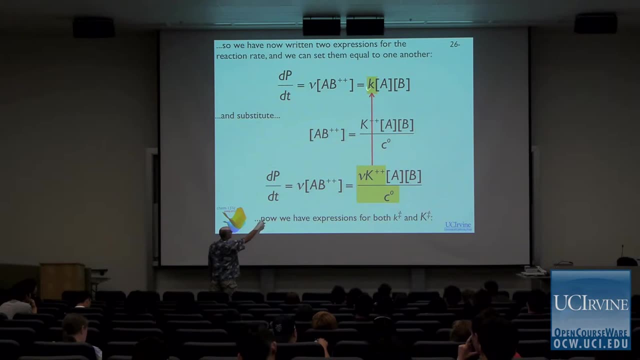 A plus B goes to products. We know that the reaction rate is K times A times B for it. as long as that's an elementary reaction, Right, All right. And what we've said is: look that rate constant is given by this expression, right here. 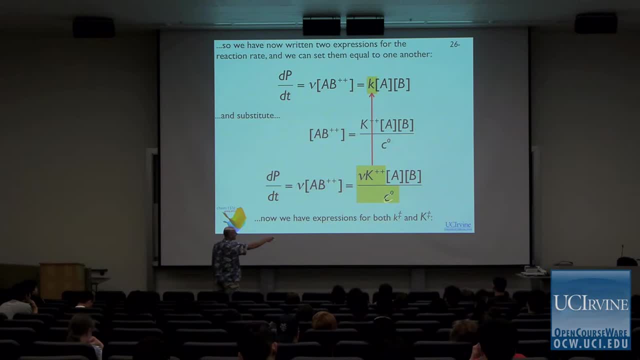 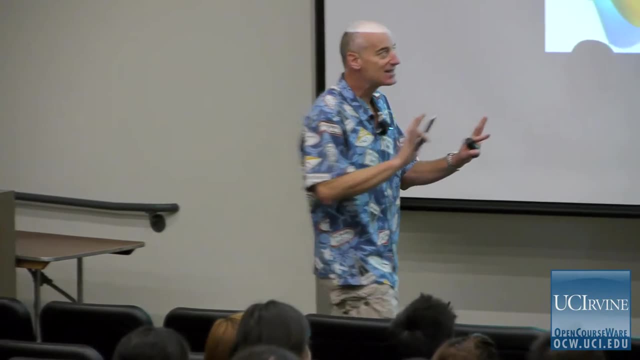 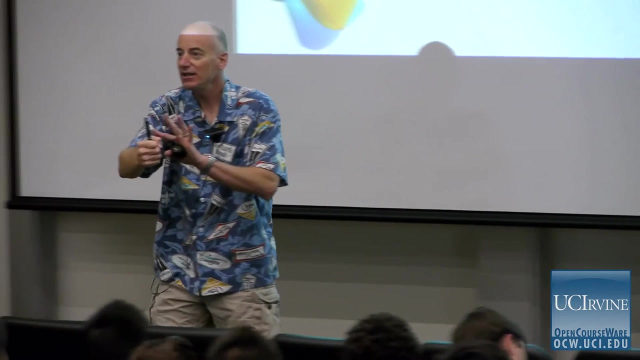 That frequency times, that equilibrium constant divided by this concentration term, just to keep the units right, All right. So transition state theory has already- and the important thing is, these two parameters here relate directly to physical parameters of the transition state that we can think about calculating- 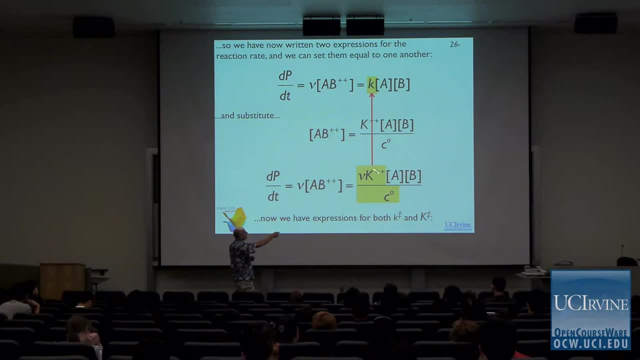 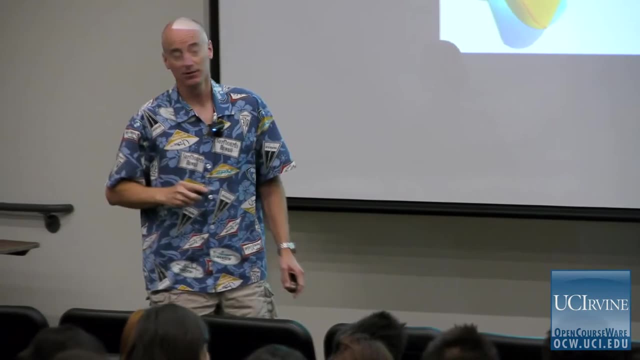 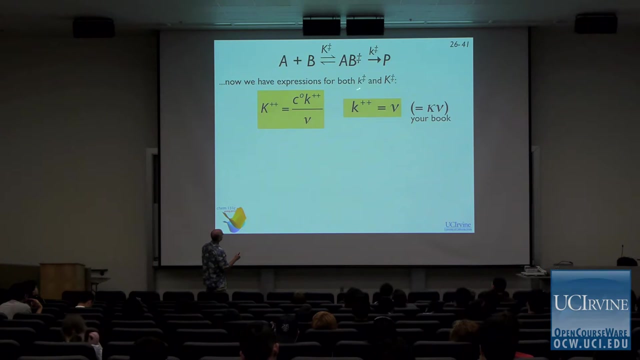 In other words, we can calculate this rate constant from fundamental properties of the transition state, because we know enough physical chemistry to do that already. Okay, So here's our transition. So we have the key point is, we have expressions for this equilibrium constant. 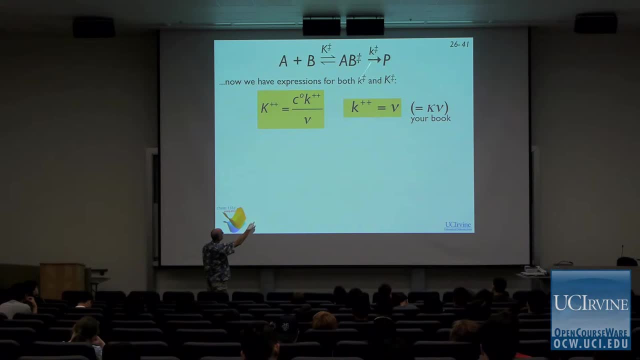 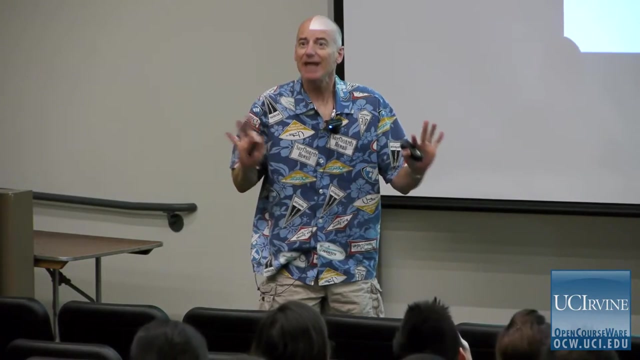 and for this rate constant right here We said that's just equal to V. This guy is equal to C zero times K, double dagger divided by V. Okay, And so let's say that we actually do want to calculate now what the rate constant is. 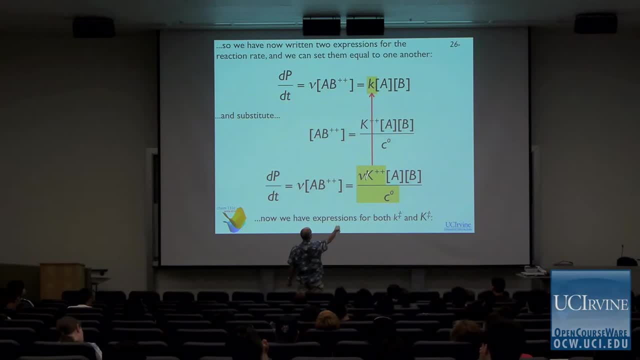 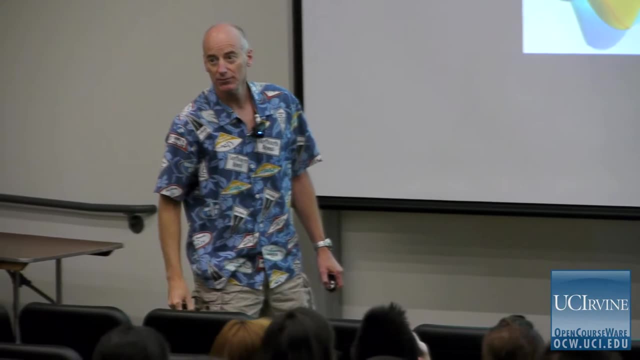 Let's say that we actually want to calculate that K right there. We have to be able to calculate big K double dagger and we've got to be able to calculate little K double dagger, which is just equal to V. How are we going to do that? 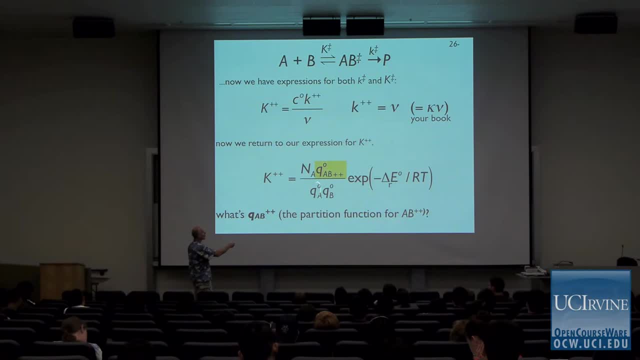 Well, here's the expression for big K, double dagger. We know what the partition function of A and B are. We know how to calculate that already. We've done that. How do we calculate the partition function of the transition state? How do we calculate that partition function? 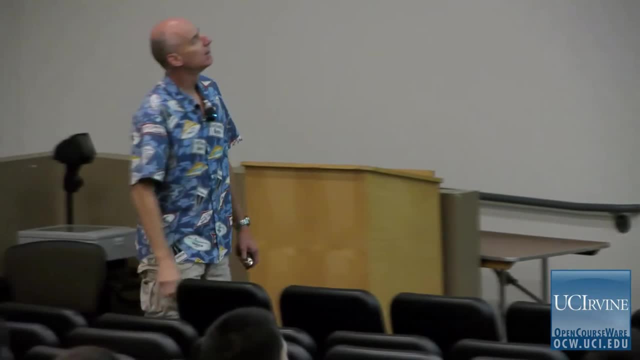 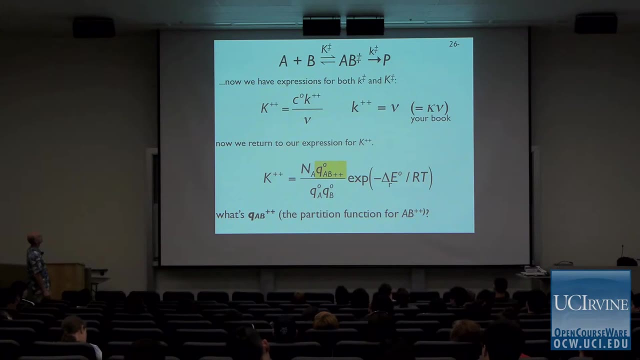 I'm just confused on your K double dagger expression. Which rate constant should we be using there? because that goes up with the rate constant delta. that is equal to the frequency. That's the same as that. That's the same as that. Well, that's a little confusing, isn't it. 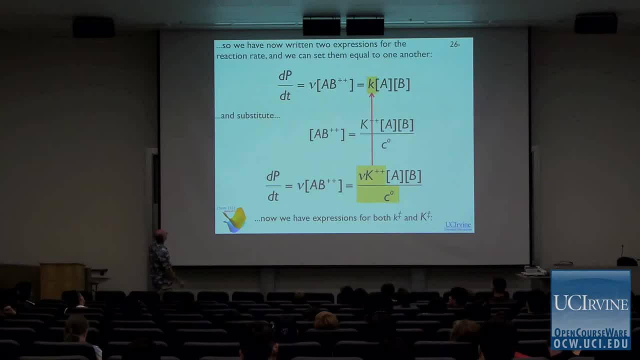 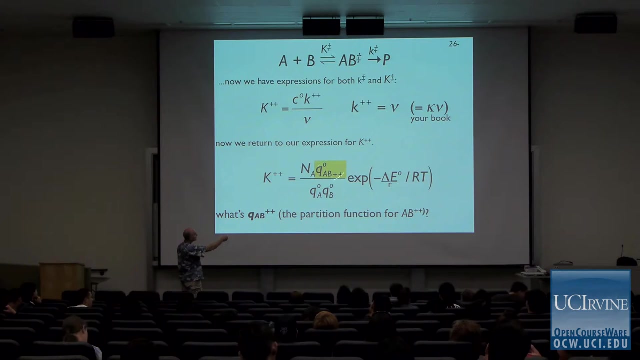 Okay, What the heck did I? That's supposed to be K sorry, that shouldn't be K double dagger, That should just be K sorry. you're right, Those that double dagger shouldn't be there. Thank you, Okay. How do we calculate that transition state? 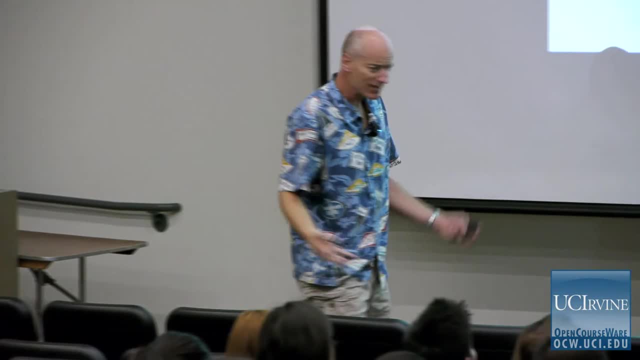 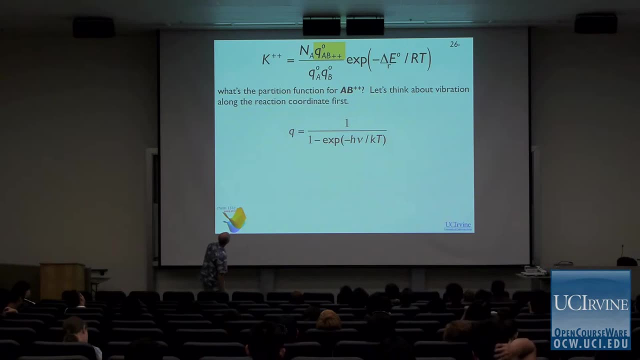 I mean, how do we calculate that partition function? It's a transition state, for goodness sakes. What is it? This is the question that these guys wrestled with when they worked out transition state theory. If we think about the vibrational partition function, 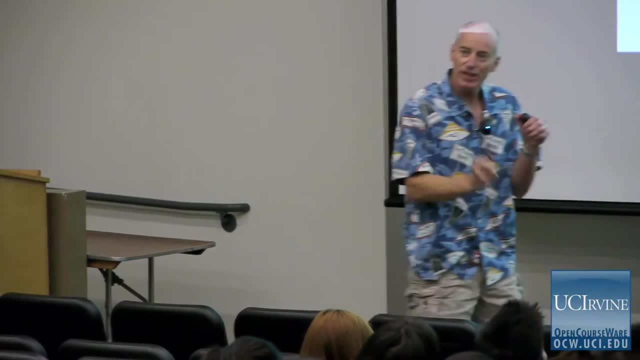 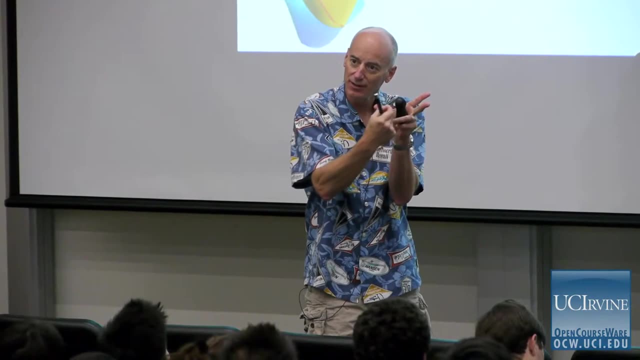 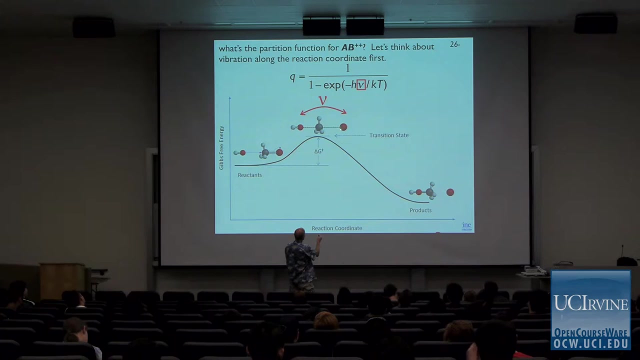 first, it's the vibrational partition function that we really care about here. Essentially, the transition state is undergoing a vibration. How do I think about that? I mean, this bond is going to be a constant. This bond is getting longer. This bond is getting shorter. all right, 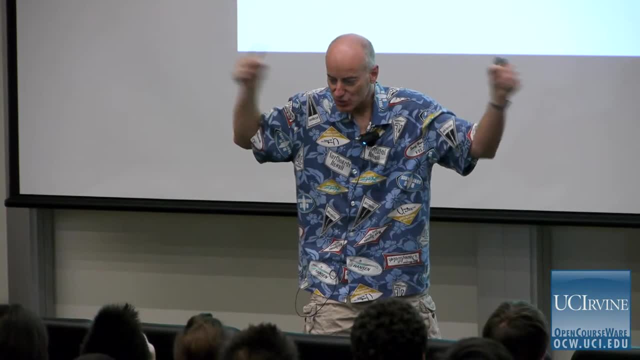 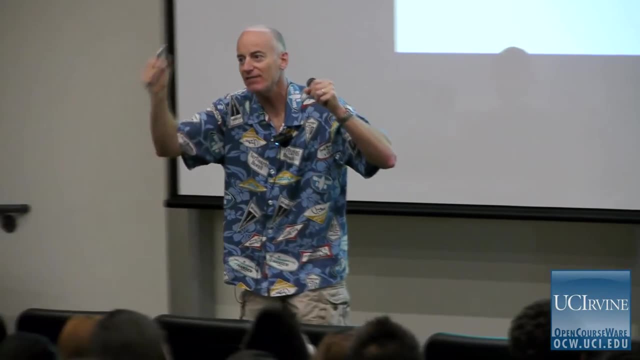 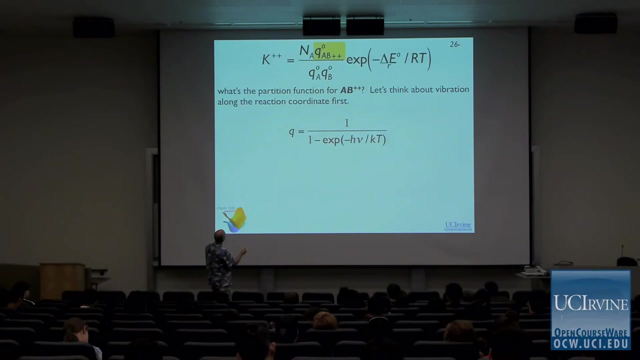 It's like an asymmetric stretch of the transition state. That's the mode that we care about. So if we could calculate the partition function for that vibrational mode, that's critical to understanding what the reaction rate is going to be, All right. 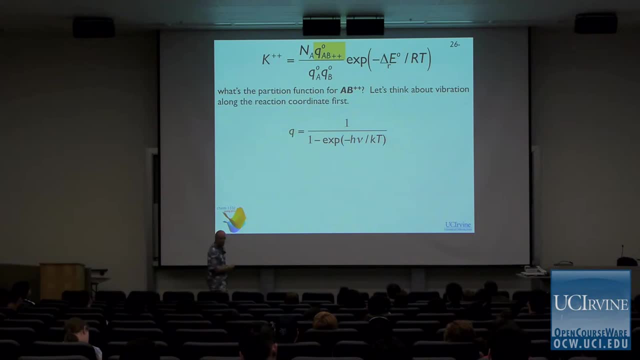 So here's the generic expression for the vibrational partition function: right For some mode, For some mode that has a natural frequency or a natural energy- h new and a natural frequency, nu. all. right, Now, what can we say about this magic mode that we care about? 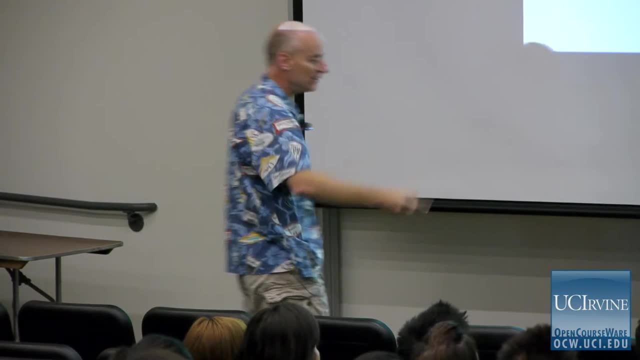 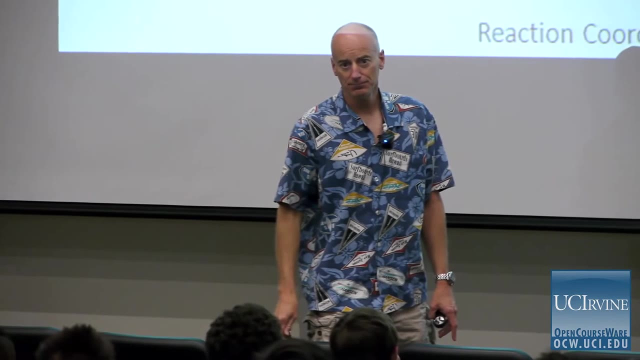 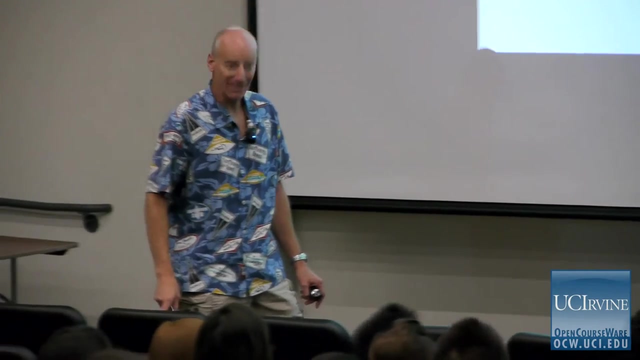 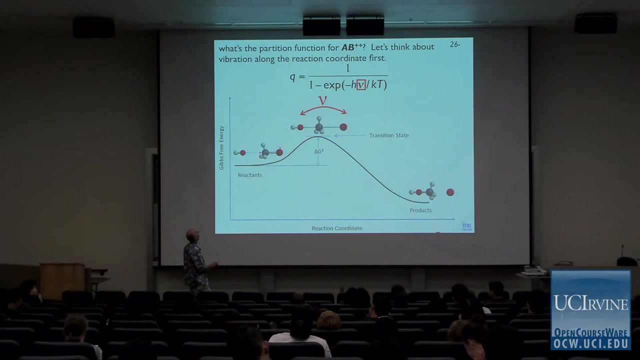 This asymmetric vibration along this axis. Is that going to be a high frequency mode, a low frequency mode? What do you guys think? High, High frequency, Yes, Low. So tell me, these are weak bonds here, right? Do weak bonds have high frequencies or low frequencies? 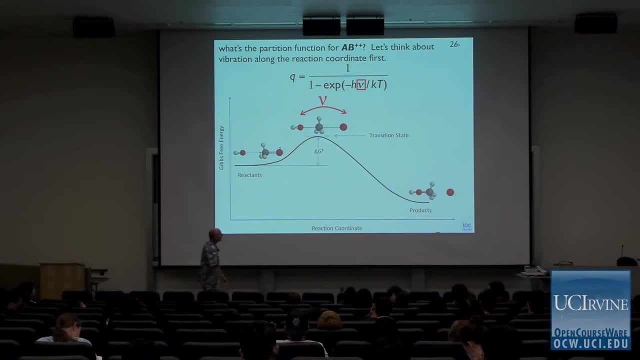 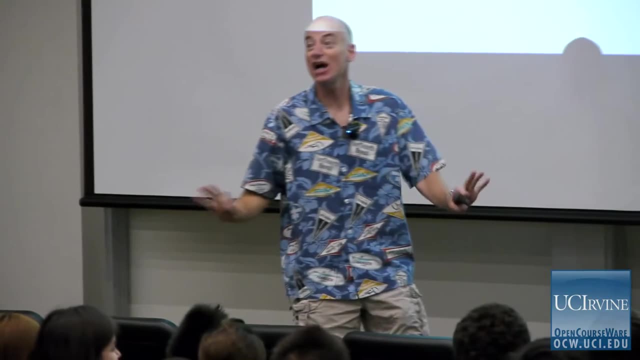 Low, Low. Thank you. All right, so we're going to expect this to be a weak bond. We're going to expect this to be a very low frequency mode. We call these soft modes. All right, here's a picture from your chapter. 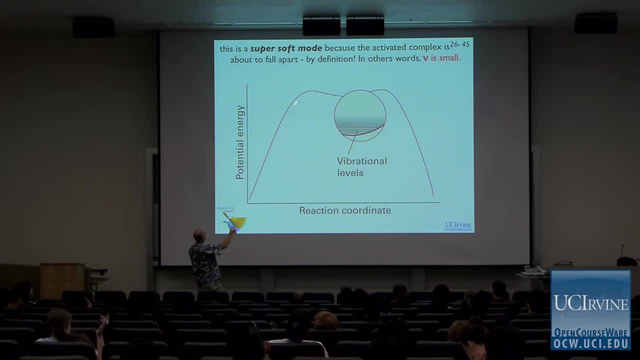 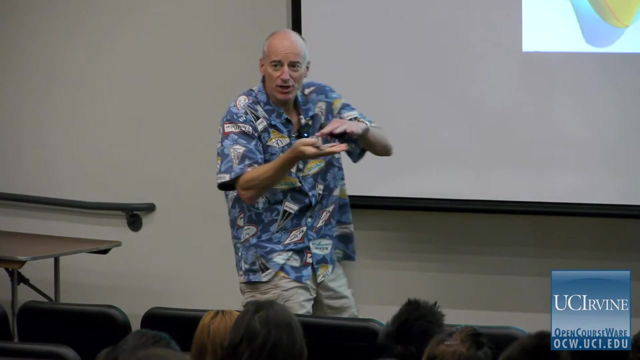 that, I think, is somewhat non-intuitive. All right, here's the transition state up here. What this picture is trying to convey is that the transition state has a very shallow vibrational energy. well, with very with vibrational energy levels that are very 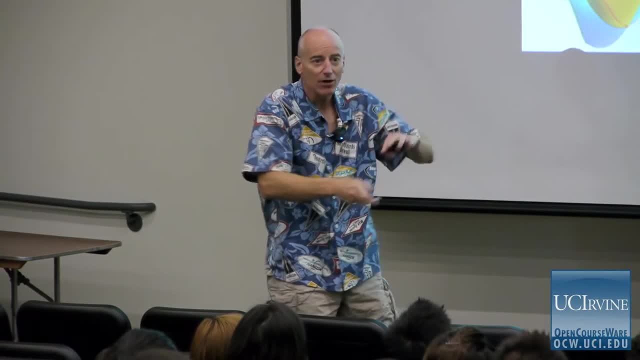 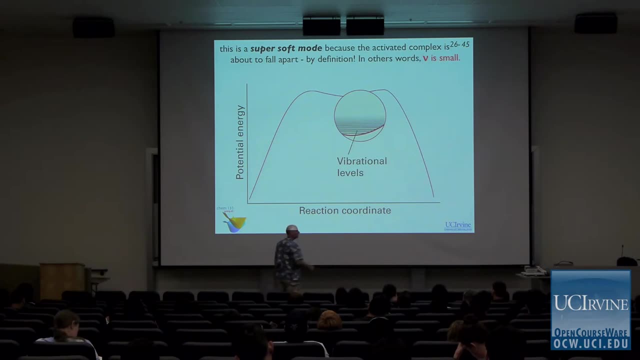 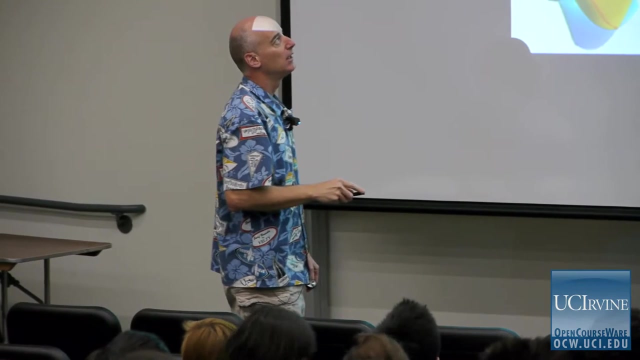 very close together, All right, in other words, the frequency. you know, to go from here to here, that H? nu is tiny, All right, So it's easy to change the Yes, but the key point is that the frequency. 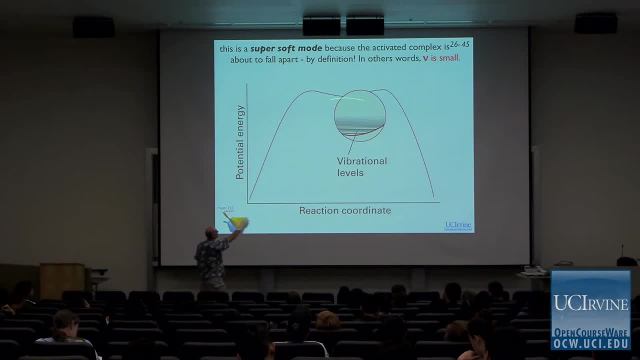 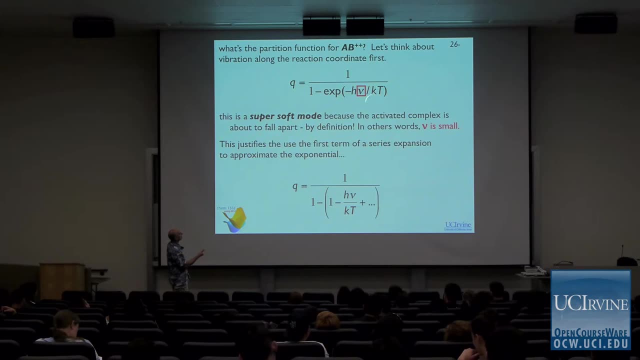 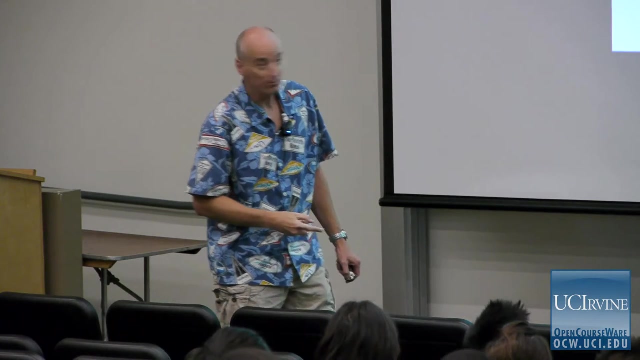 that characterizes these transitions in the transition state along this direction right here is very small. So what that allows us to do is simplify this equation. We can write this exponential as a series and we can truncate it at the first term, and when we do that, we just get KT over H? nu. 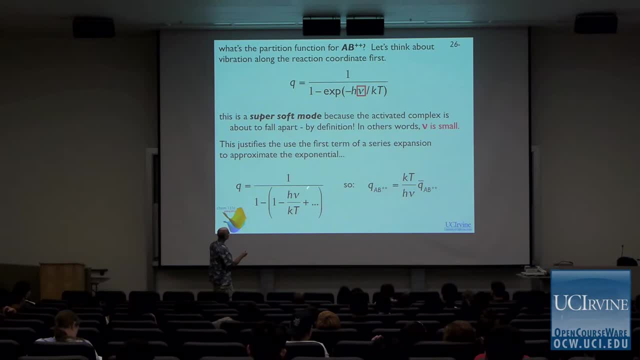 All right, we take this normal expression for the partition function, we truncate it, we write it as a series: expansion, the exponential, and we truncate it at the first term and we just get KT over H nu. This is a special nu. 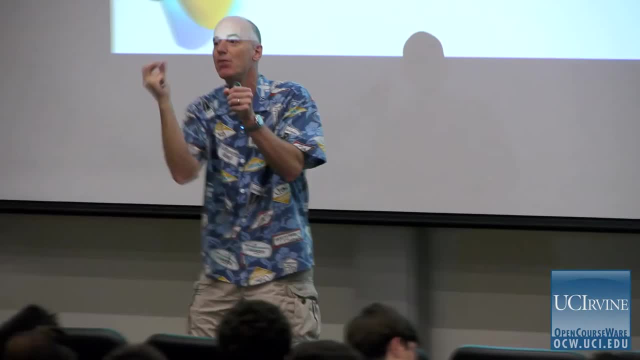 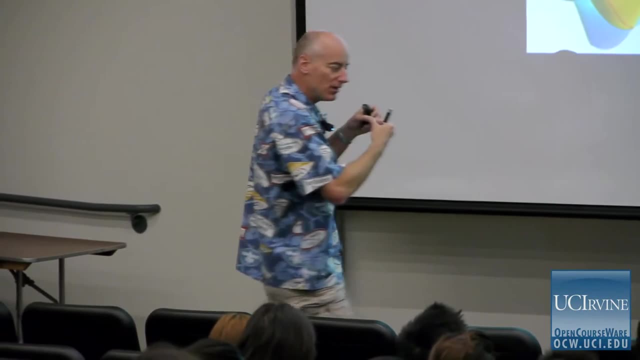 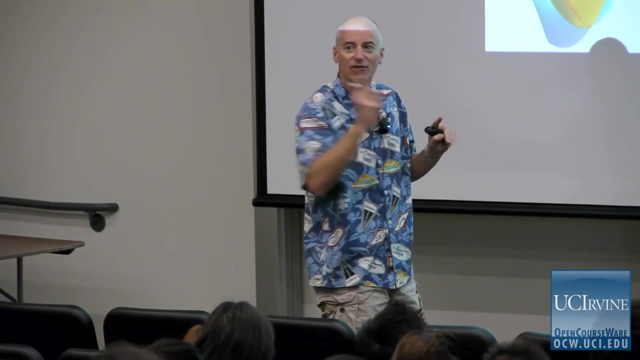 This is the frequency that describes motion over the barrier. all right, Whatever that is for, whatever the transition state is, whatever mode- the product bonds are getting formed, reactant bonds are getting consumed. we can think about that process as involving a single vibration. 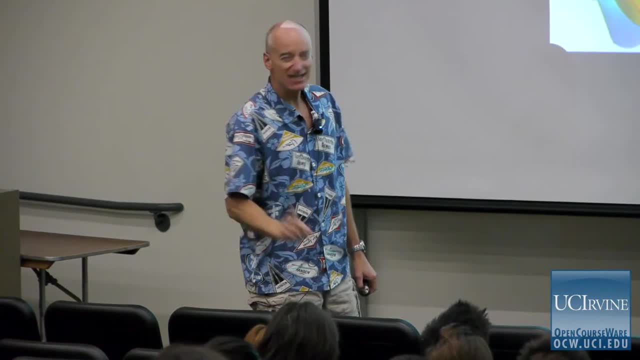 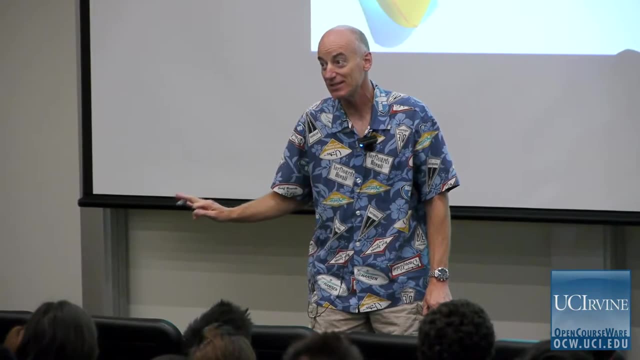 that has a very low frequency in general. That's what they realized Conceptually. this is not obvious. I think everybody in this room would agree. none of this stuff that I'm talking about in the last five minutes is obvious. This was the conceptual leap that Polanyi made. 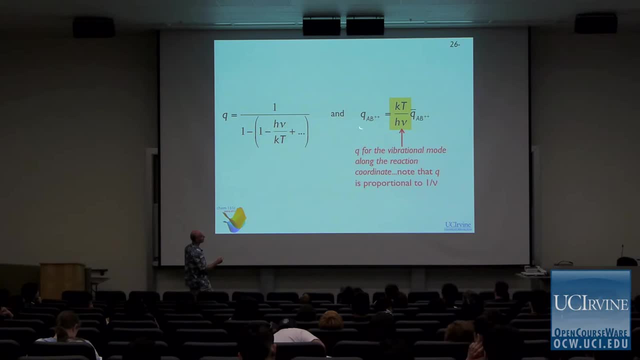 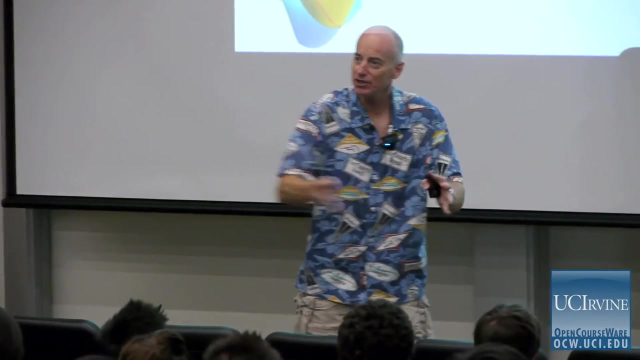 Okay, so I can write the whole partition function for the transition state as the partition function for this low frequency mode and then the whole rest of the partition function. All right, notice that there's going to be a rotational, an electronic, a translational. the partition function contains: 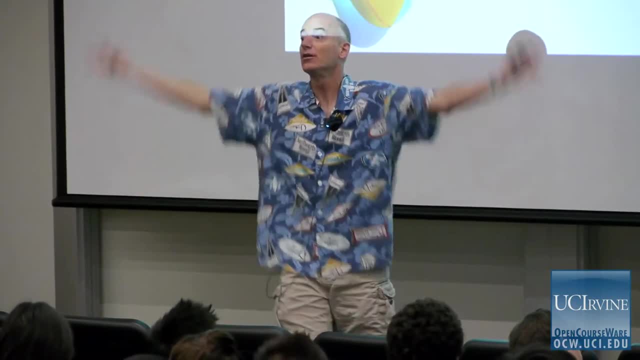 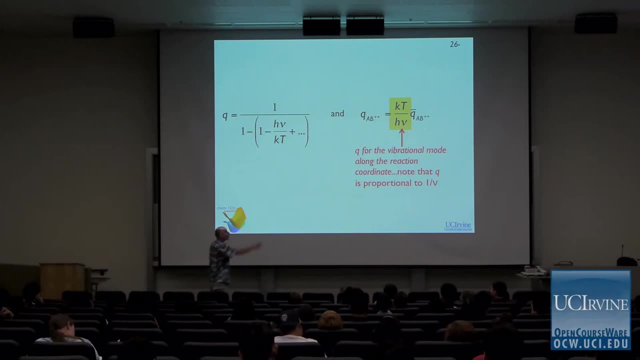 many other manifolds And other vibrational modes as well for the molecule that are orthogonal right to this special mode. All right, we're going to roll that all into this guy over here. This is just the partition function for the magic mode. 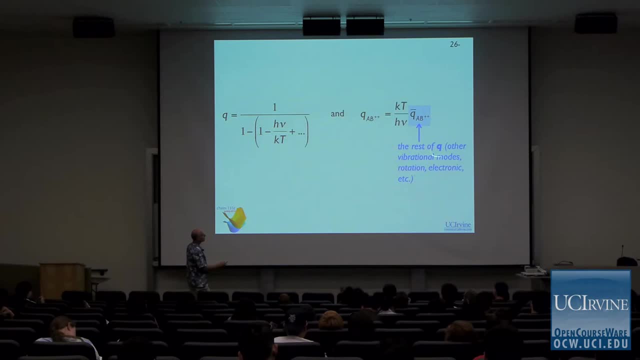 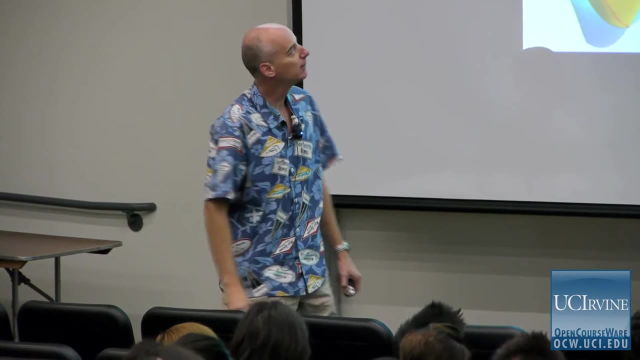 that corresponds to the reaction. This is the rest of Q, All the rest of the partition function for all the other modes, manifolds and so on. Okay, So that's the partition function. I'm going to just plug that in then. 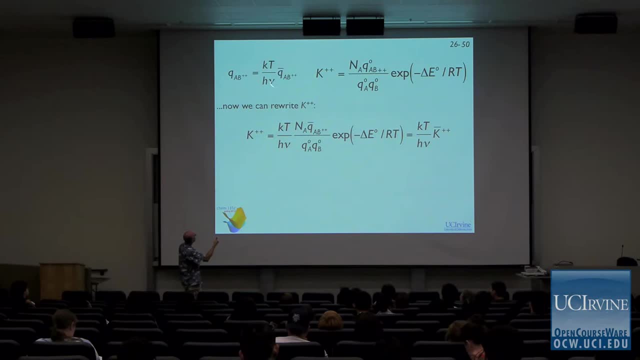 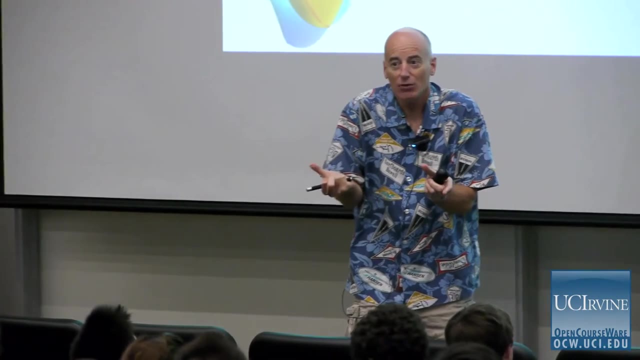 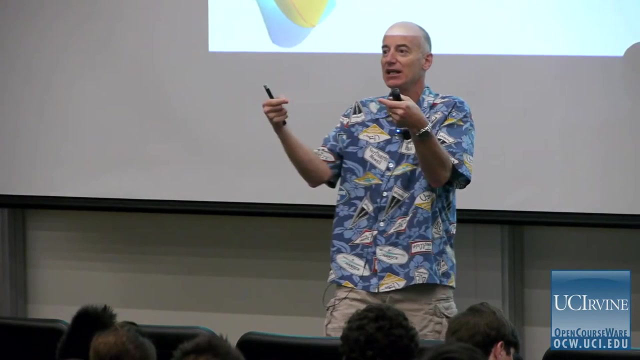 Here's the partition function that we were wondering about. Here's the expression we now have for it. Notice that the rest of this partition function involves things that we can already calculate, because they're things that are not perturbed in the molecule. What's perturbed in the transition state is product. 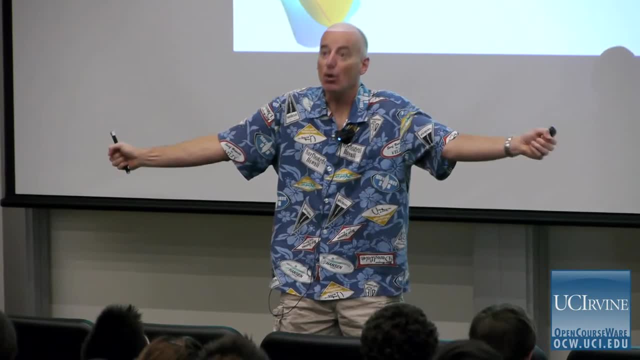 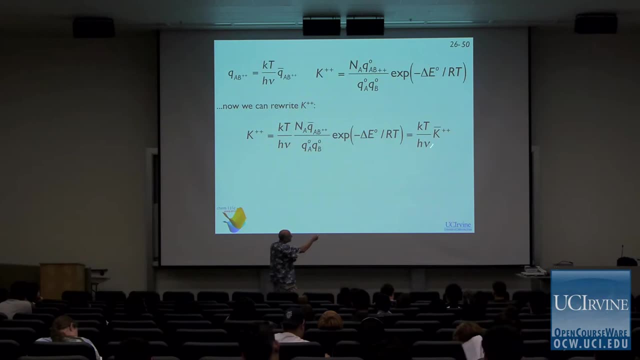 bonds are getting formed, Reactant bonds are getting broken- All right, and we can describe that. We can roll that process all into our. We're going to have to figure out what that frequency is, All right, but all the rest of this stuff we can just roll in. 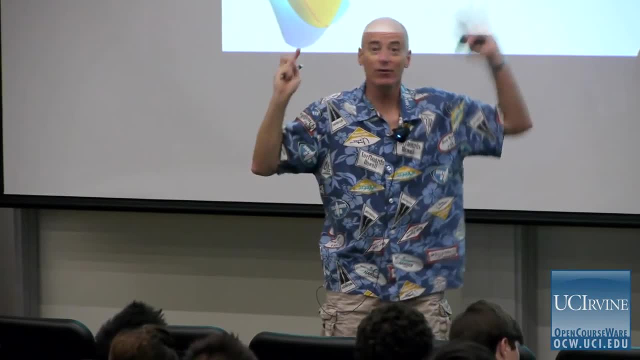 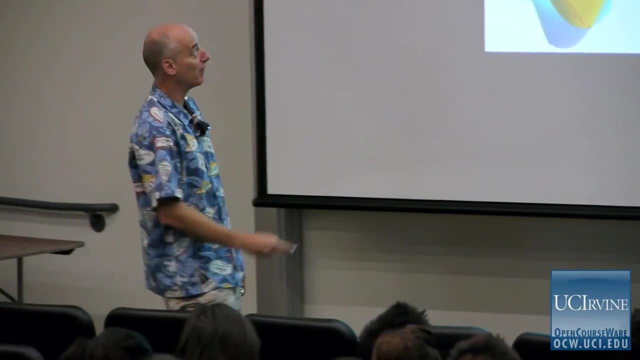 All right, bonds that are orthogonal to the reaction rate. we can just calculate their vibrational partition function, their rotational partition function, all of that stuff, using the conventional methods that we already know about. Okay, so now I rewrite this in terms of this guy right here: 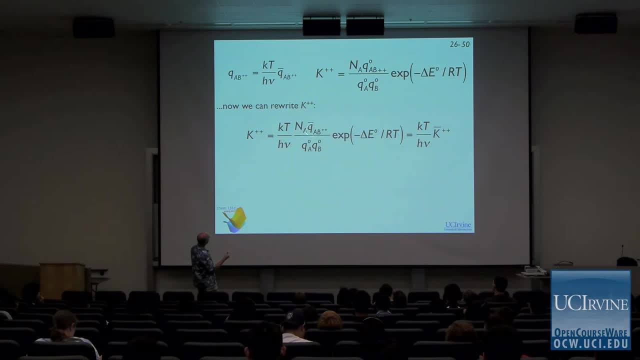 Look at this: KT over H. nu. Now, that's right here. It's right there. Here's the rest of the partition function, this Q with a line over it here. All right, and I'm getting close to being able to calculate this guy. 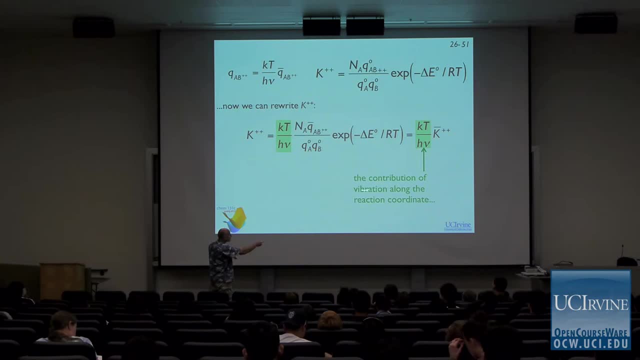 This is the contribution along the reaction coordinate. only Yes, yes, this is all the rest of it. Yes, Okay. so our expression for the rate constant becomes this: and we're just plugging now this expression in: for the rate constant. All right, so we're going to have to figure out what's going on. 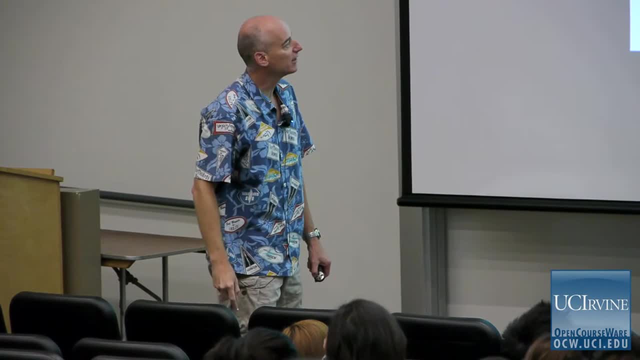 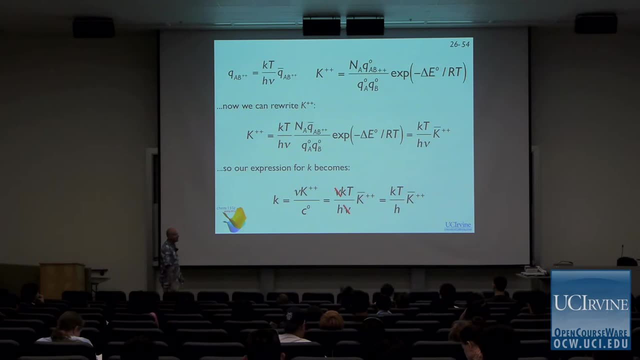 All right. so we're going to have to figure out what's going on, This equilibrium constant with the double dagger on it. All right, and so we can. actually, when we do that, we can cancel this frequency. Hey, turns out, we don't need to know what it is. 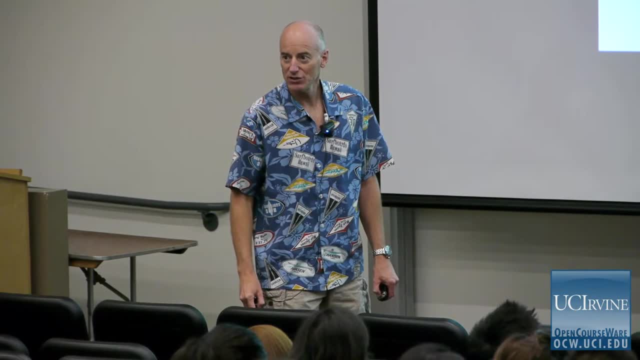 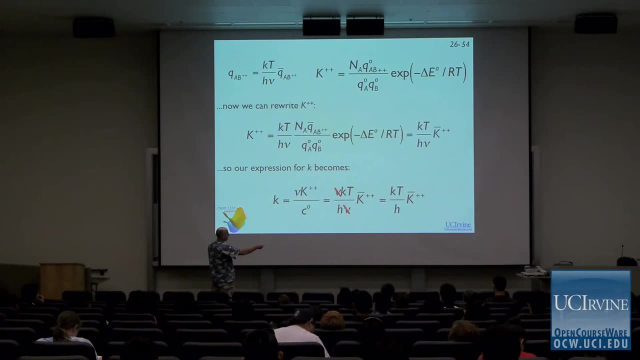 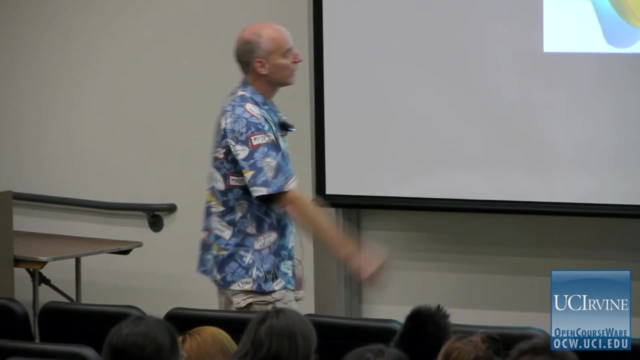 It cancels, for gosh sakes. All right, we don't have to measure it. All right, we get this expression right here and this is the famous airing equation. All right, we derived it going way too fast, In about 20 minutes. 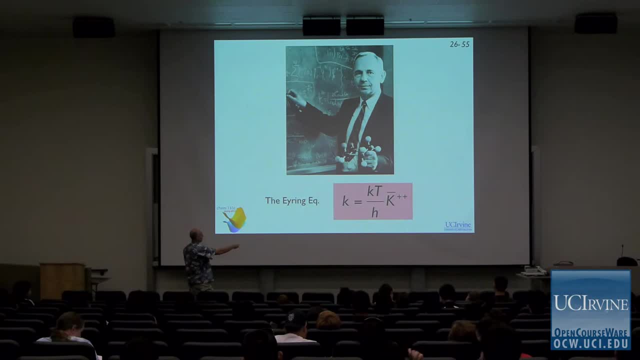 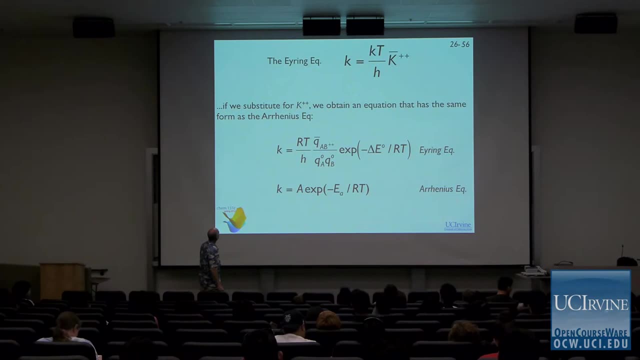 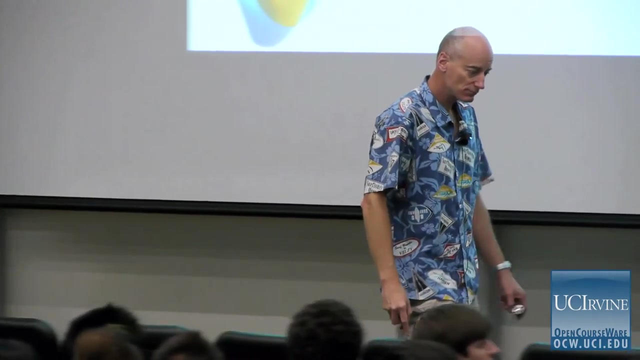 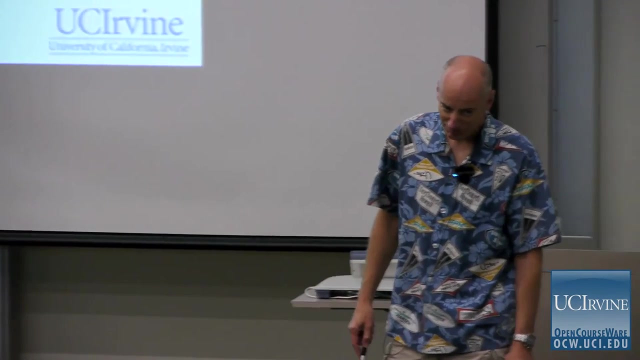 All right, here's. this is a very important equation. Now, why is it so important, Professor? Yeah, How do we find K using K? How do we find K using K? 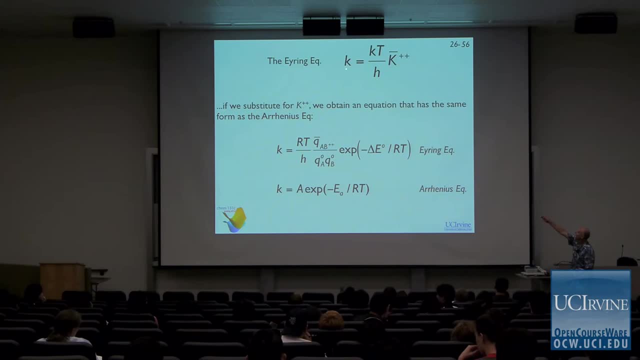 How do we find that K using that K? No, the little K within the equation. 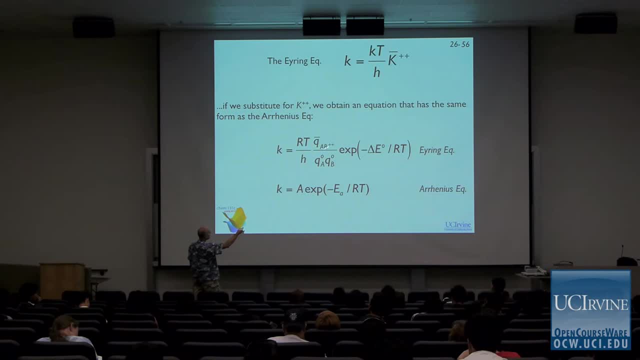 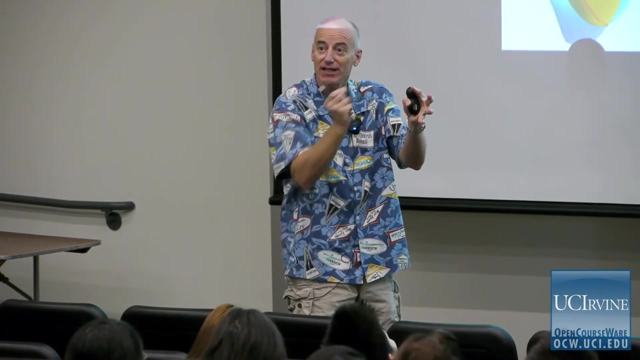 of variables. right here R T over H times this guy. what's left over from the partition function, We strip out from the normal partition function. for the transition state, we strip out the part of it that pertains to the vibration along the reaction coordinate. 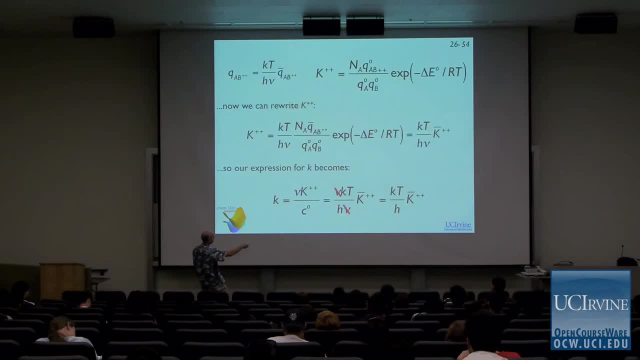 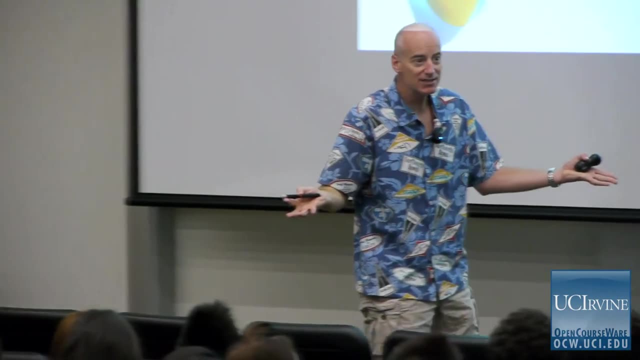 and that's what's left over, because remember that frequency just cancelled for us. We don't need to know it. That's a good thing, because who knows what it is Okay. How would you measure it? You'd have to have some exotic spectroscopic method to do that. 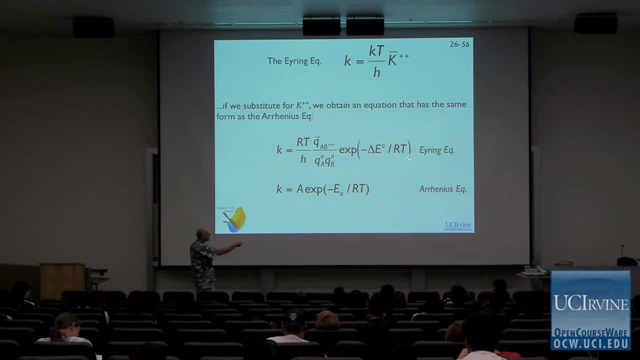 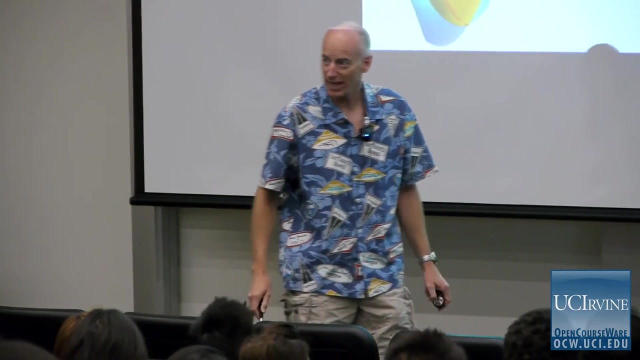 Okay, So the Arrhenius equation is a special case of the erroring equation, right, And we can calculate these things. and if you don't believe me, go to slide 101 and we go through and we do it laboriously for a particular reaction. 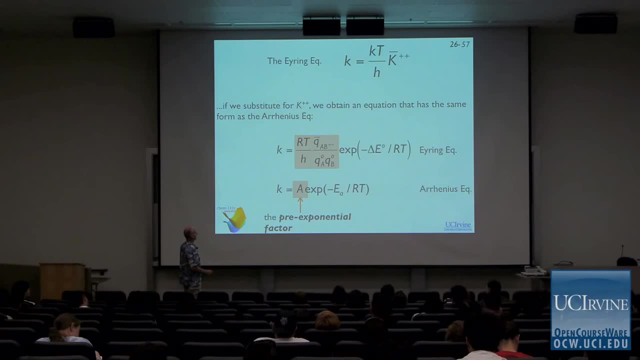 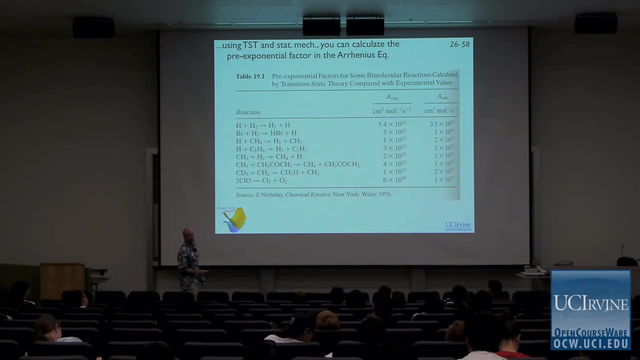 We're not going to say more about it, sadly. All right, here are pre-exponential factors. You can calculate this one. actually, it is calculated later in this lecture. All right, we can calculate these pre-exponential factors for the Arrhenius equation, knowing transition state theory. 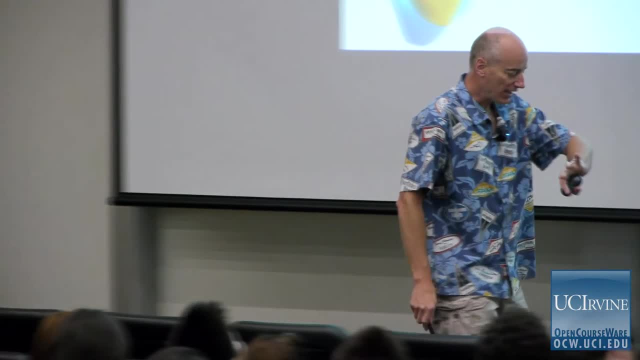 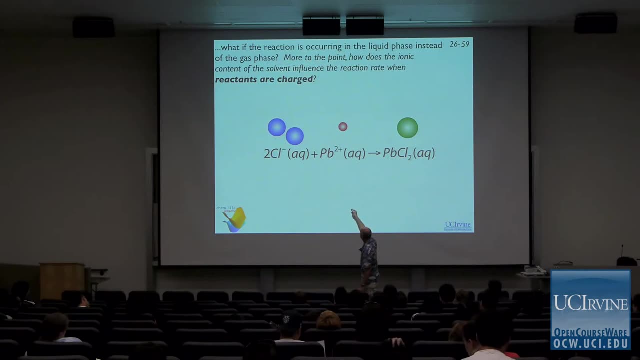 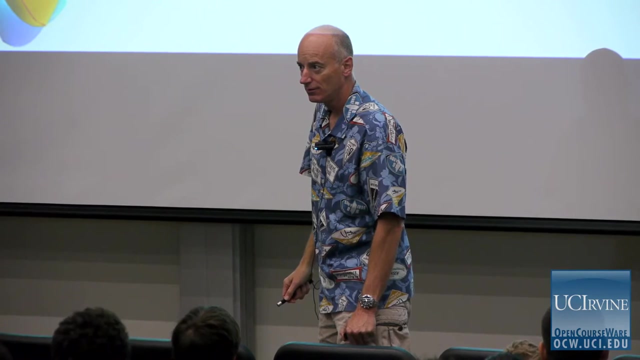 so it's very powerful. Okay, what can we do in the last 15 minutes? Something very important. All right, we want to apply the same thinking to a reaction that occurs in water. Okay, And the key point is that we want to think. 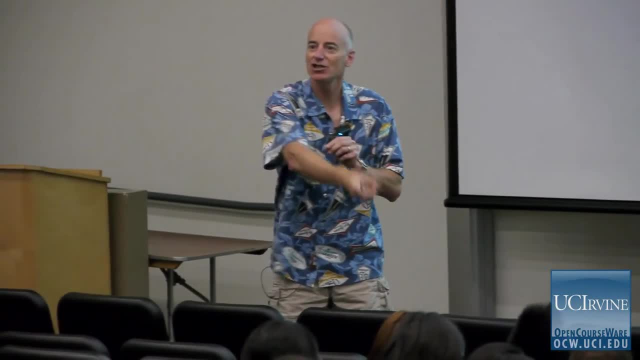 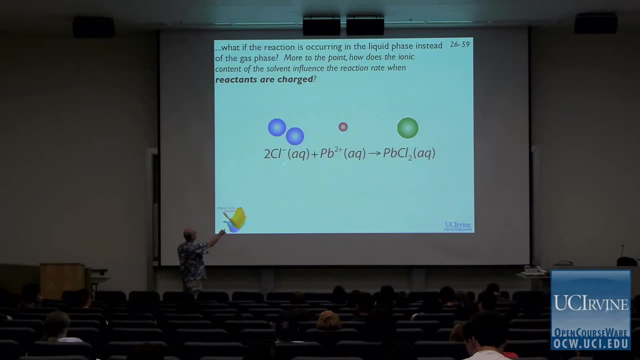 about what the influence of charge is on the reaction rate. It's not inconceivable that there could be a question like this. on the final, For example, two chlorides react with lead to give lead chloride. All of these things can be in solution, right? 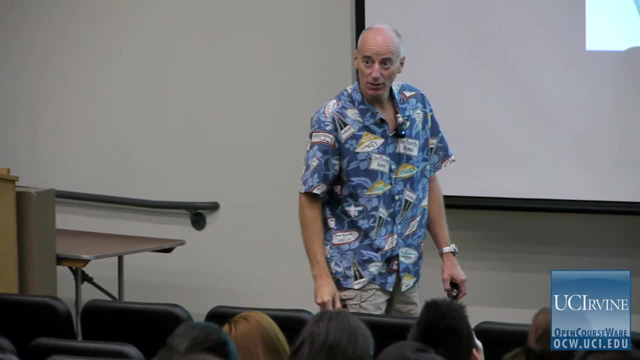 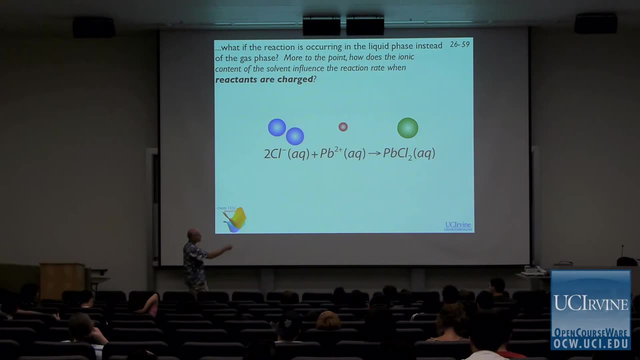 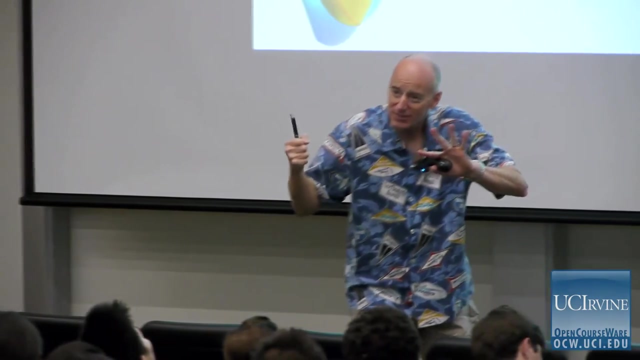 Lead chloride has some solubility in water- very low, All right. what rate would this reaction take? All right. what is the influence of the charge on the reaction rate? You might think naively: if the reactants and products are oppositely charged, they're going. 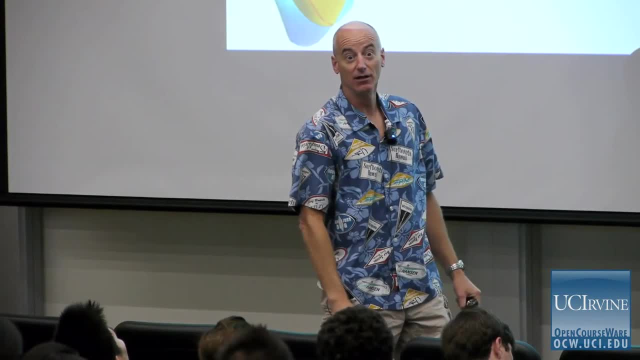 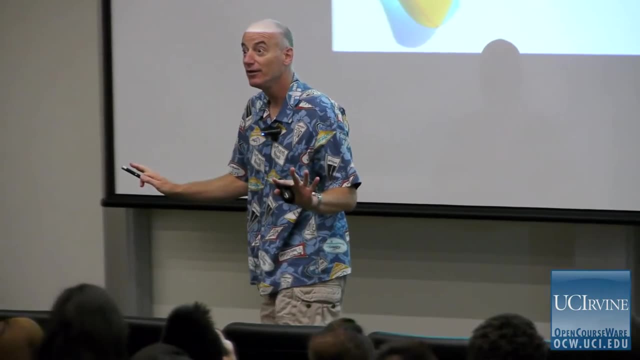 to be attractively attracted to one another and the reaction rate is going to be accelerated. All right, if you don't think about this too hard. even if you think about it hard, you might come to that conclusion, All right. negatively charged reactants. 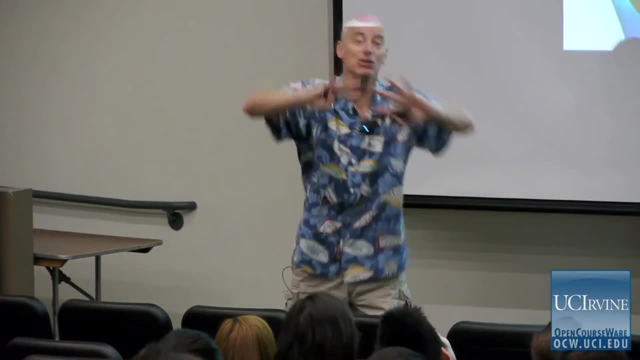 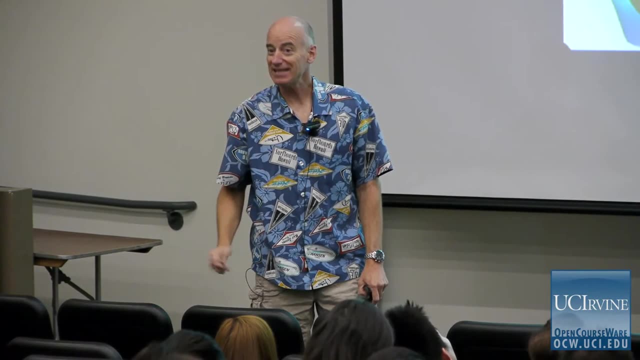 and positively charged reactants are going to be coulombically attracted and boom, they're going to react really fast. That's going to accelerate the reaction rate. All right, that turns out to be exactly wrong, and it's important to understand why. 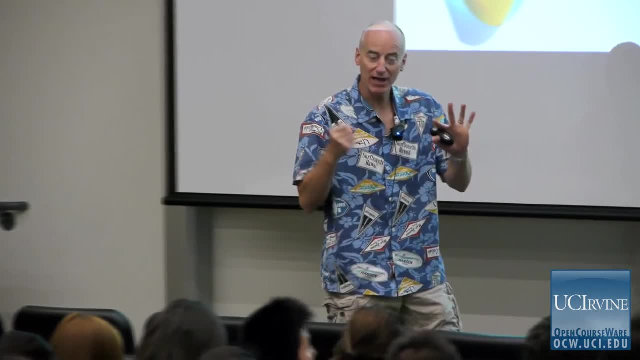 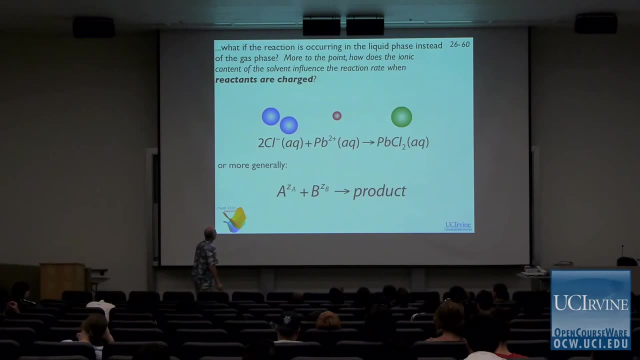 All right. it's great once in a while in chemistry when you encounter a concept that is completely counterintuitive at first and later on, hopefully intuitive, All right. so I've got to make this happen in like 12 minutes. Here's the idea. 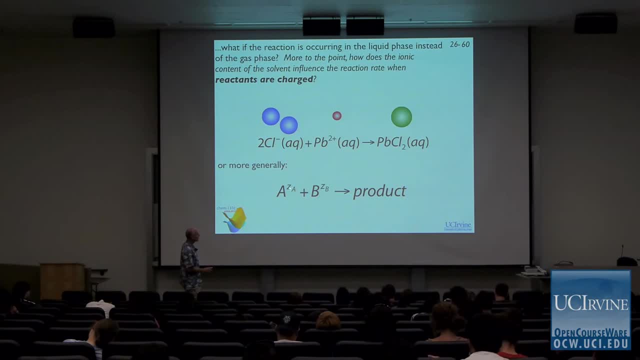 A reacts with B to give products. That's the charge on A and B, ZA and ZB. That's the charge. The key point here is: reactants are charged. So there's a version of transition state theory, but it's not strictly speaking transition state theory. 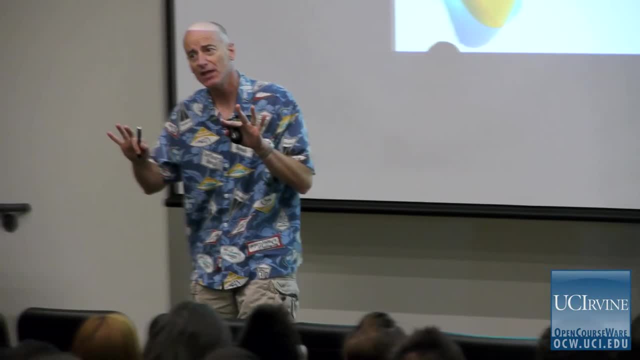 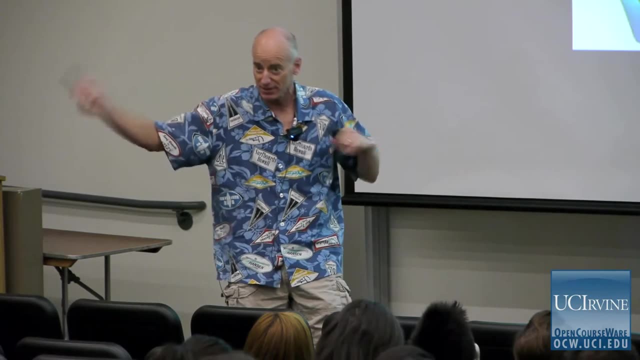 It's a thermodynamic version of it. You can't use transition state theory in its normal form to describe reactions and solution, because it doesn't account for reactions with solvent. All right, it doesn't. transition state theory in its normal form does not account. 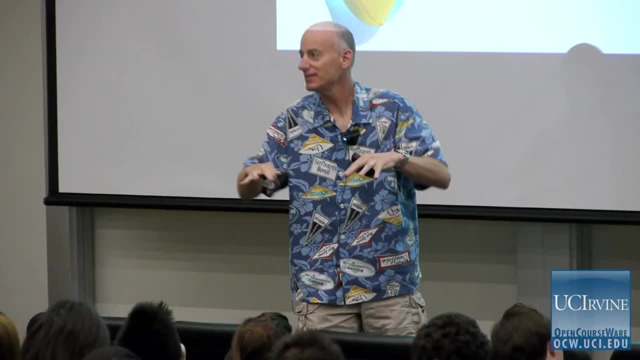 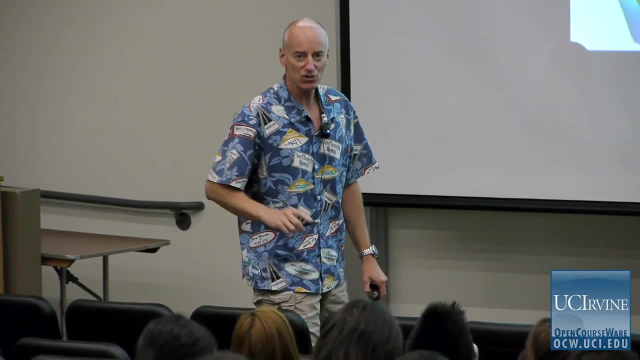 for the complexities imparted by having the solvent present in the reaction. All right, so this is a. this looks like transition state theory, but strictly speaking it's something that's related to it, not exactly the same thing. We're going to simplify this notation. 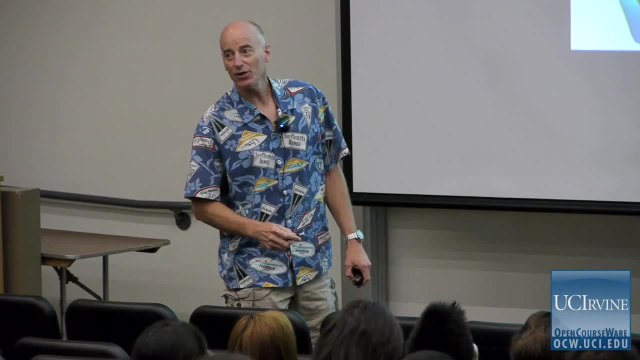 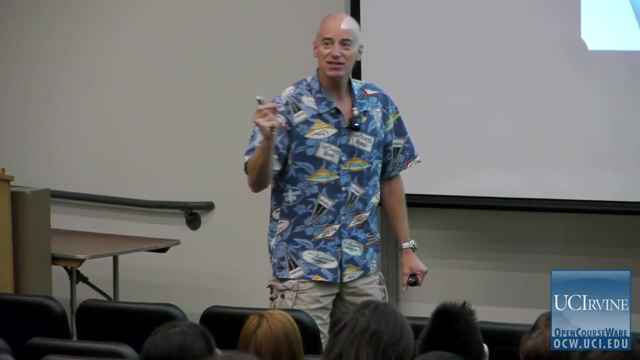 We're going to call this mess All right. so notice something: If we think about this in terms of transition state theory, when A reacts with B, if we form a transition state, the transition state will have a total charge equal to A plus B, right? 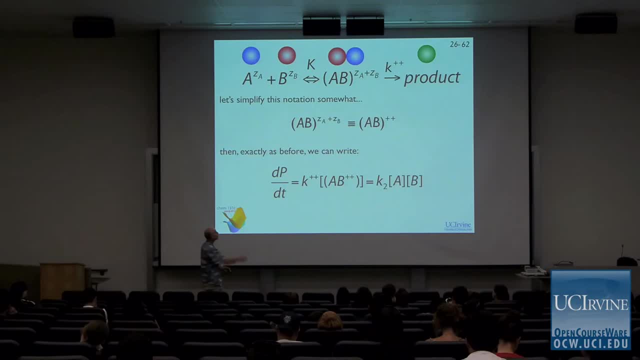 Right, the total charge of the transition state will be the sum of the charges on A and B, because charge has to be conserved here. that's a key point. Okay, so exactly, we can write the. this is the reaction rate. 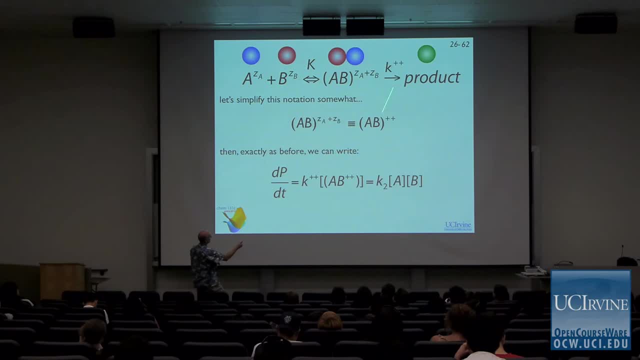 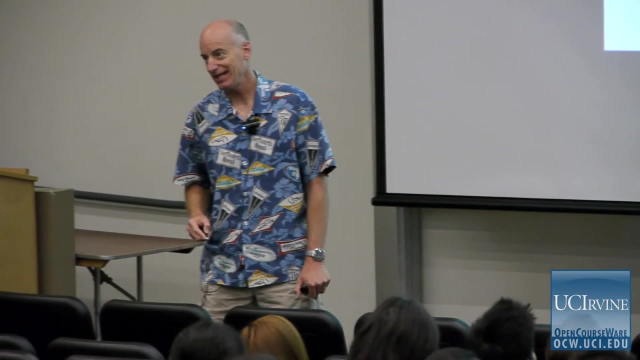 Now, in terms of this, is just that rate constant right there? This is the normal phenomenological rate that we would write for this reaction. Okay, so then we have to think back and remember something about activities. Activities are going to be the key. 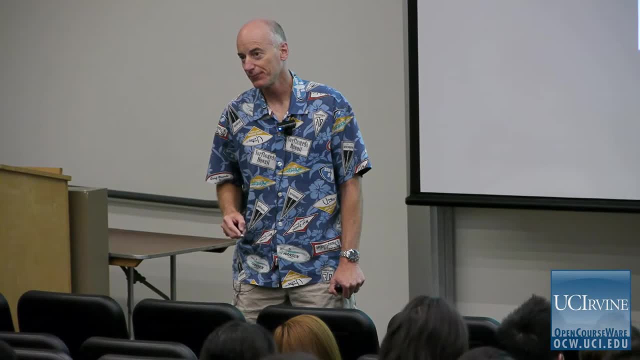 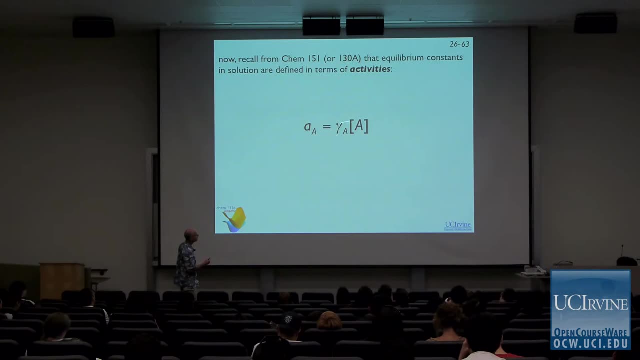 to understanding how this works. All right, the activity of some ion A is equal to its concentration times. some activity coefficient gamma sub A. All right, That's the activity of A, That's the activity coefficient. The activity coefficient for a neutral is one. 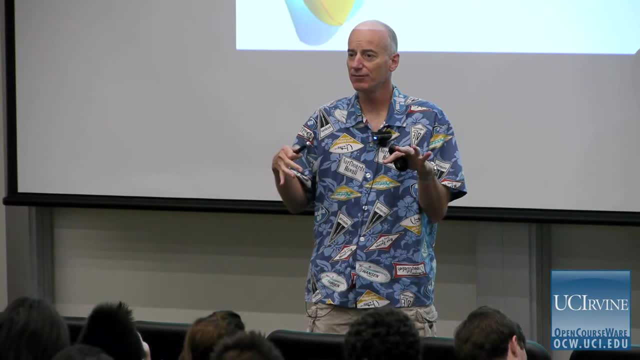 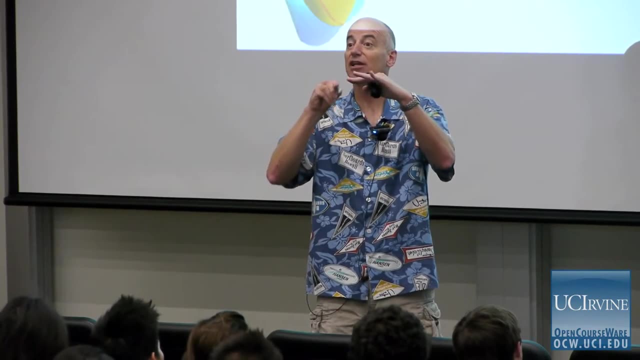 All right. the activity coefficient only deviates from one as a consequence of coulombic interactions with the solution. other ions in the solution: All right. if other ions are present in the solution, the activity coefficient will be less than one. The more ions, the lower the activity coefficient. 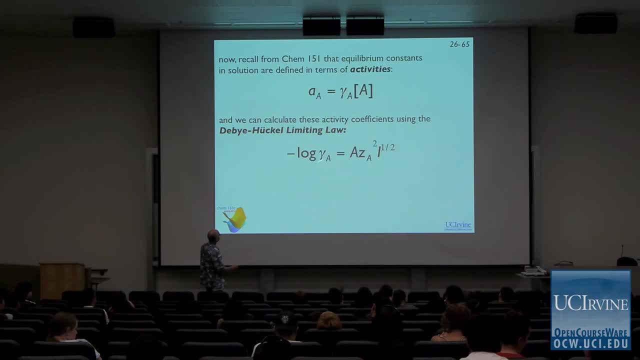 Okay, And there's a little bit of a difference here. There's something called the Debye-Hoeckle limiting law. That's the activity coefficient, That's the ionic strength, and the ionic strength is just given by this expression, where this is the concentration of the ion. 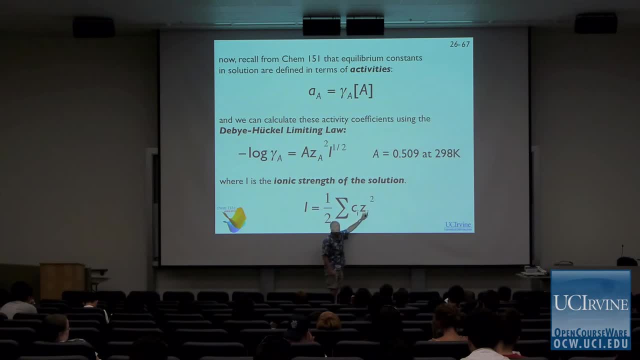 Sorry, this is the concentration of the ion and this is the charge on the ion for every ion in the solution. I add up all the ions in the solution, multiply by the square of their charge. take that times 1 half and I've got the ionic strength. 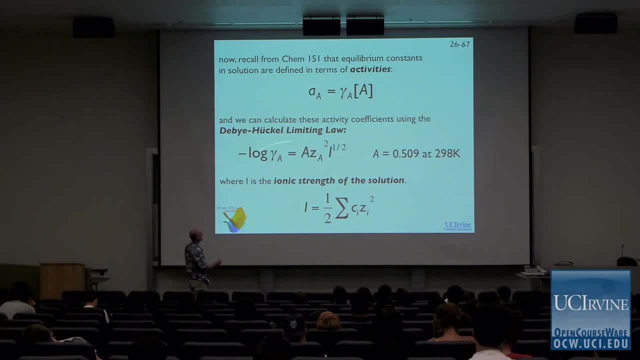 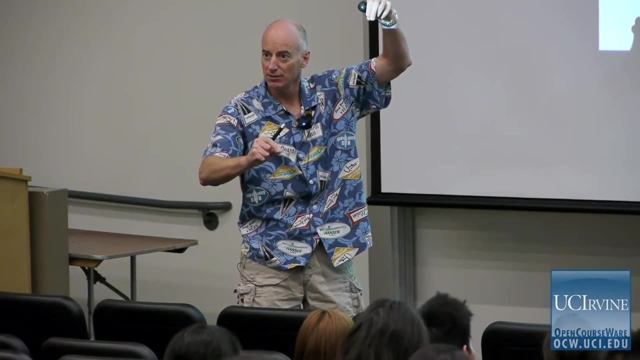 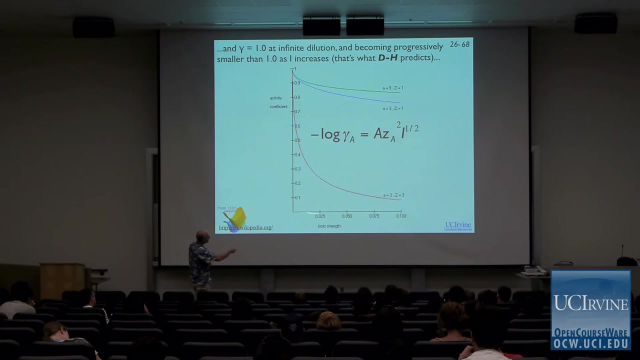 All right, the higher the ionic strength. it's never obvious to me when the equation has a log in it like this: The higher the ionic strength, the lower gamma becomes. All right, if I is zero, gamma is one. This is the ionic strength on this axis. 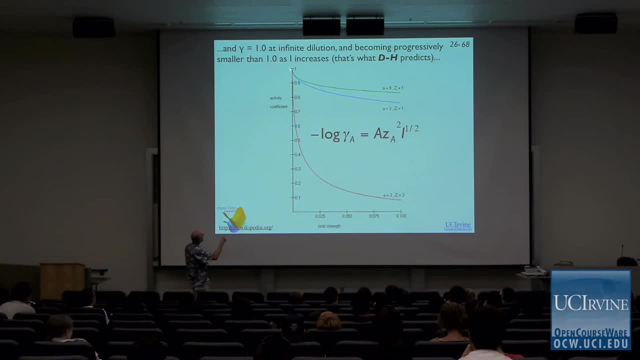 This is gamma on this axis. If ionic strength is zero, gamma is one and it deviates from one as the ionic strength goes up. That size of this deviation here depends on what the charge is on the ion of interest, ion A. All right, because here's its charge. 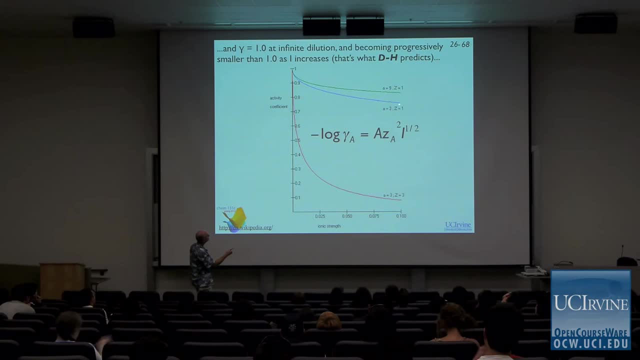 All right. so if it has a charge of one, there's a small deviation charge of all right. that's the size. If it's small, you get a little bigger deviation. If the charge goes up to three, you get a huge deviation. 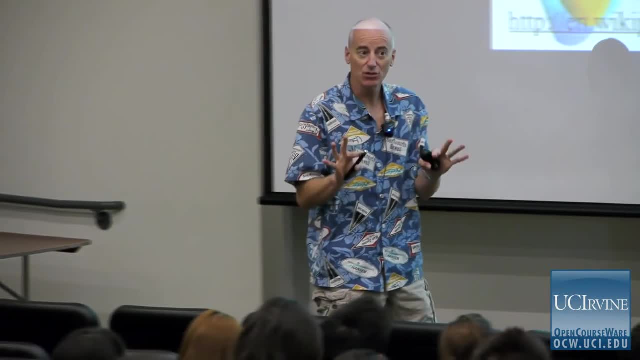 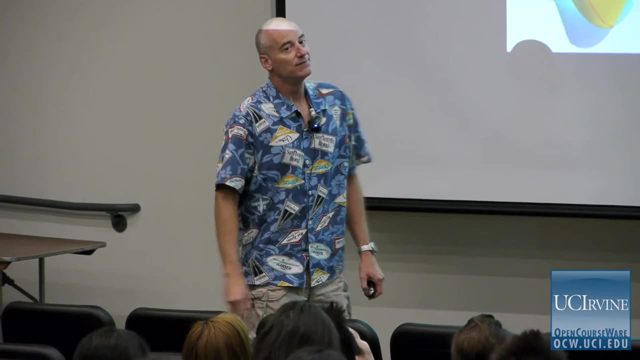 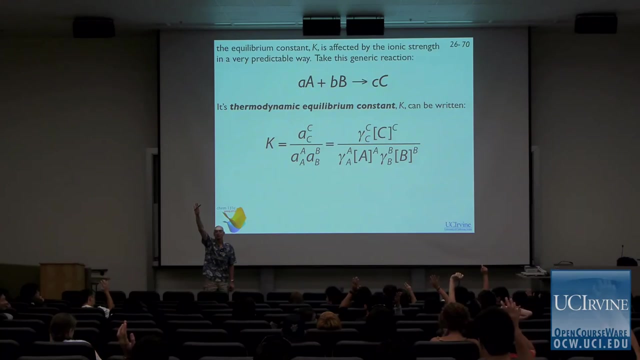 All right. so activity coefficient, Activity effects, have everything to do with charge. How many of you had 151? From me? Okay, so this is review for all you guys. Good. So when we write an equal, here's an equilibrium constant. 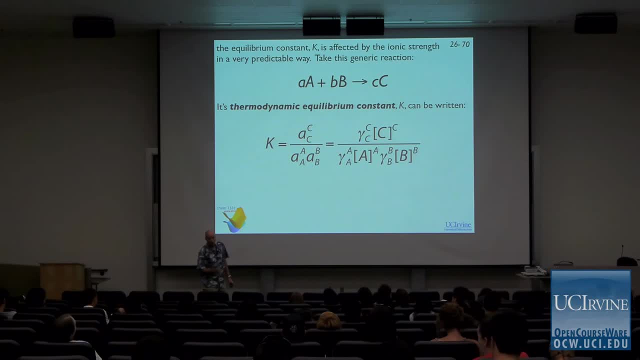 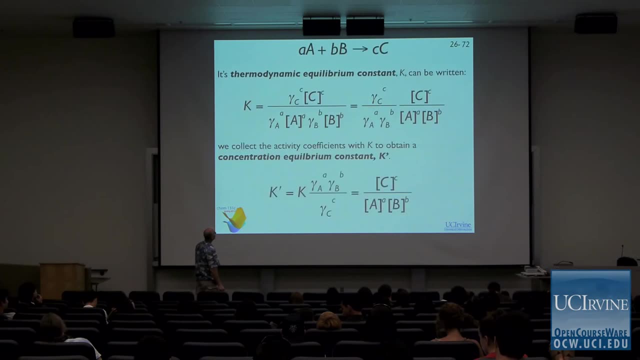 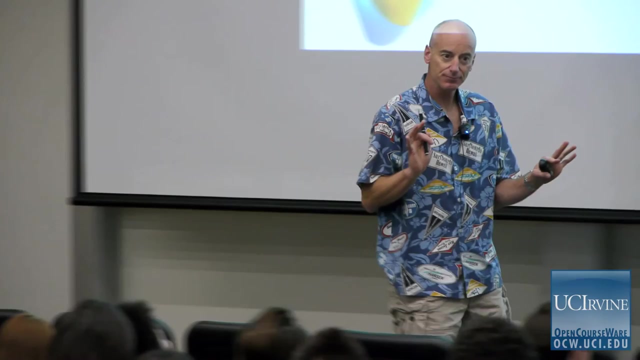 We write it in terms of activities. Every activity is an activity. coefficient times the concentration. You guys all know that And what's more important is, you have intuition about what the influence of ions are on equilibria. Here's an important piece of intuition. 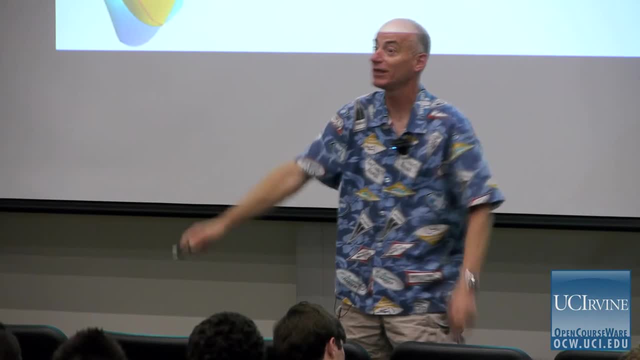 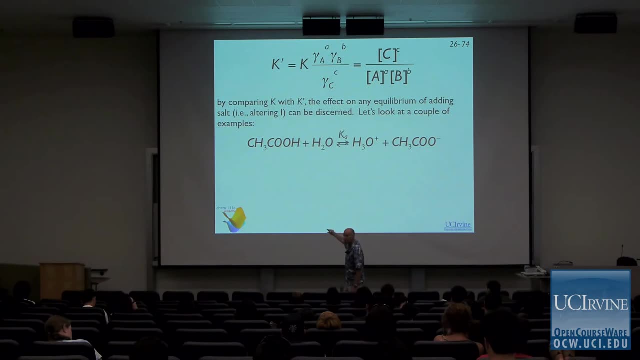 that everybody should have in the room, especially those of you who took my class. If you look at some equilibrium like this, all right, formic acid, acetic acid, Acetic acid. Acetic acid dissociates to give hydronium ion and acetate. 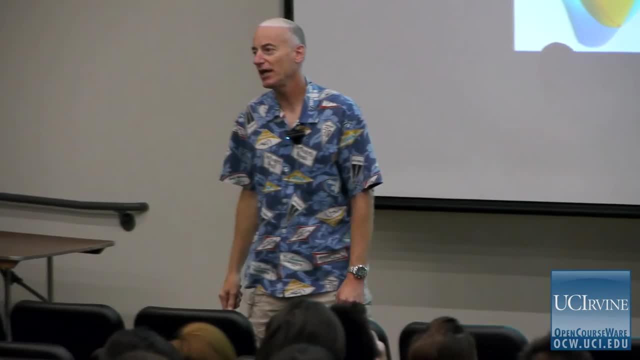 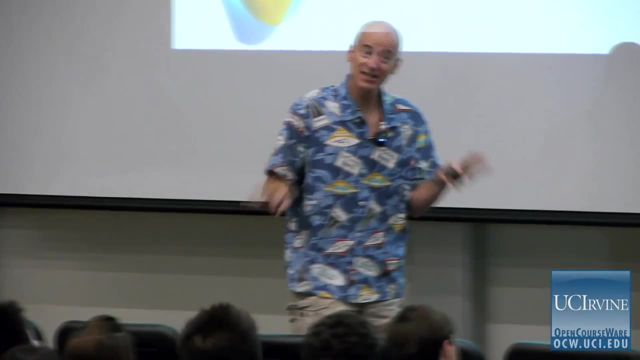 All right. if I dump sodium chloride into the solution, what's going to happen to the pH? Sodium chloride is an inert salt. Sodium chloride has no acidity or basicity of its own. All right, and yet the pH will change in a predictable way. 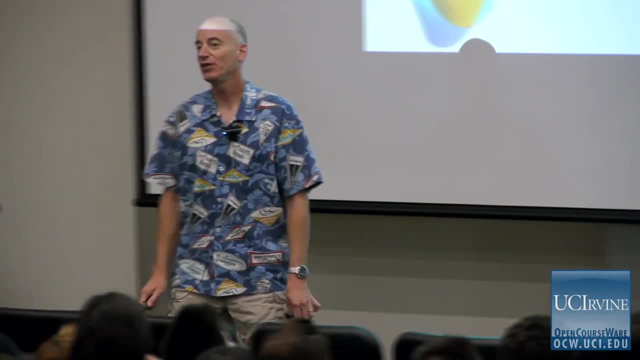 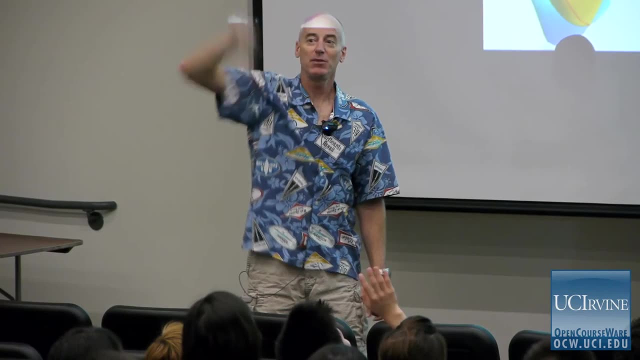 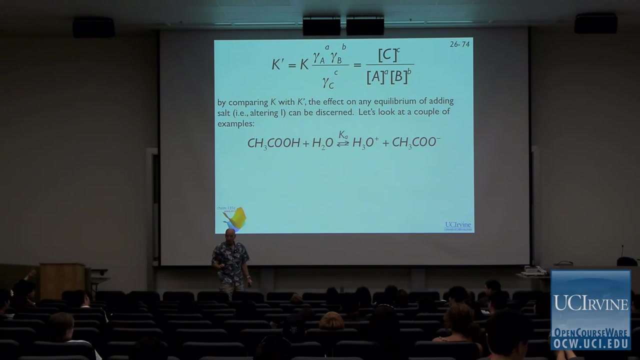 What will happen? How many people think the pH is going to go down? The solution is going to get more acidic. How many people think the pH is going to go up? It's going to get more basic. when I add salt, Get those hands way up there because I want to see. 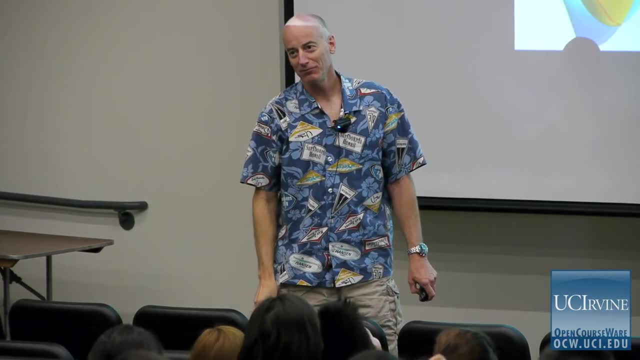 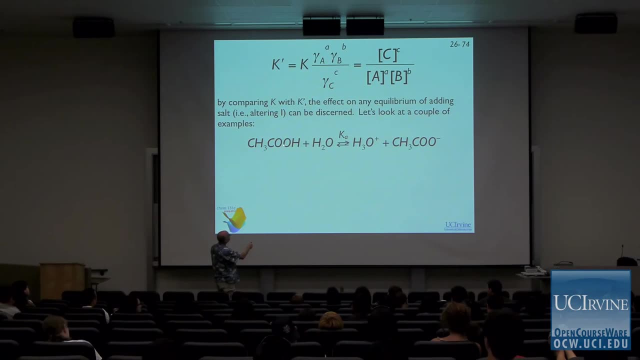 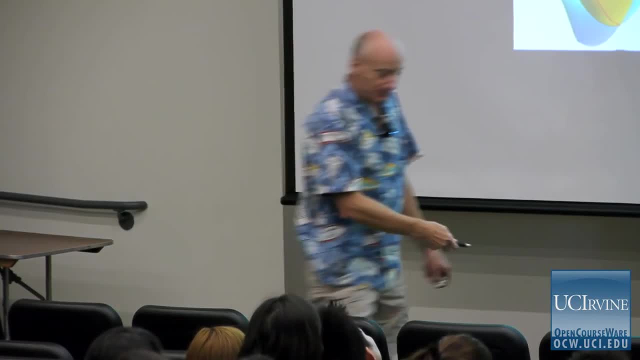 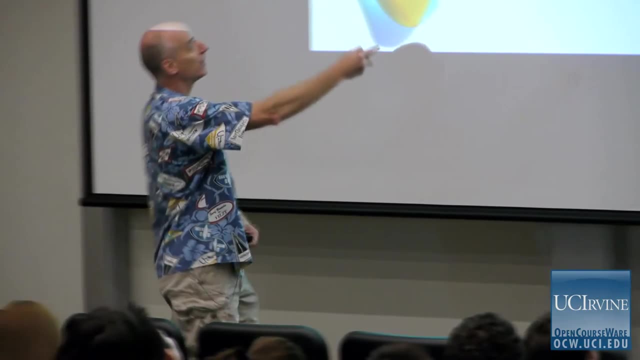 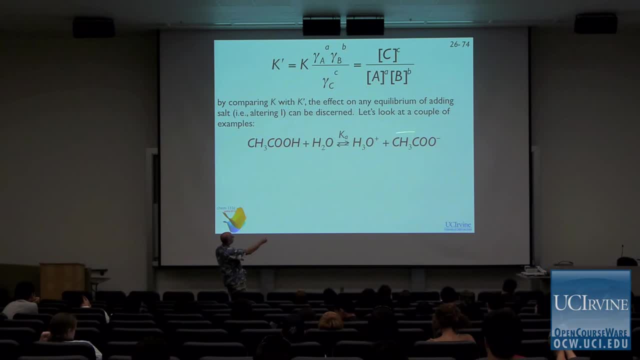 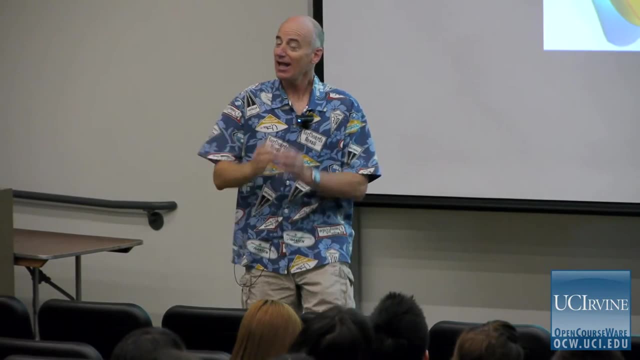 See how there's ions here and there are no ions here. All right, That's the most ionic state. If I add salt, the reaction will shift to the right. It's called salting in. All right, Now I can prove that. 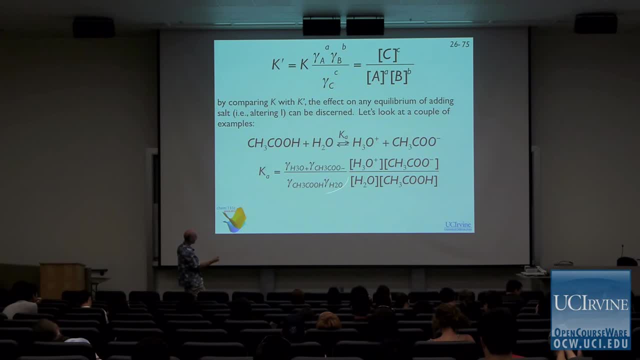 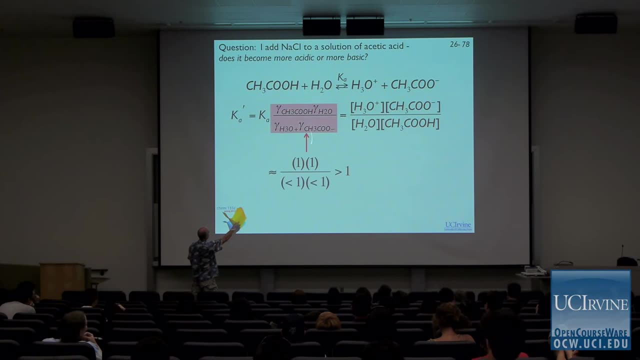 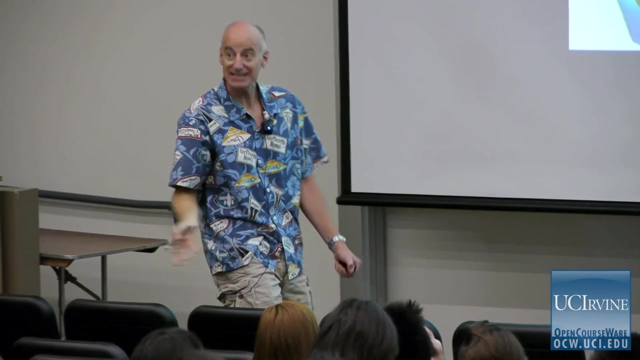 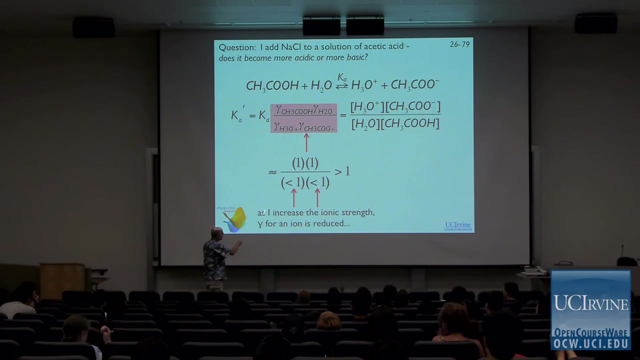 All right, Here's the equilibrium constant for this reaction. Here are the. Here's the Activity coefficients. The activity coefficients: They are less than one, Okay, And they will become lower as I increase the ionic strength of the solution. 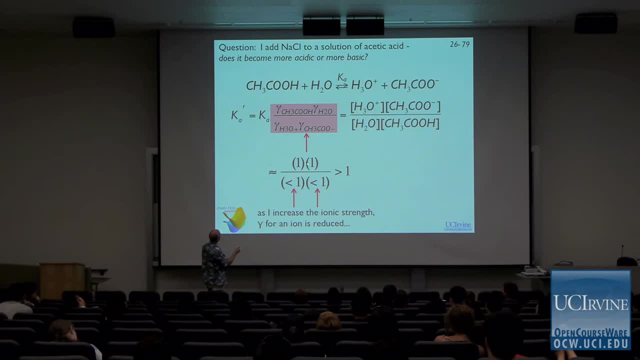 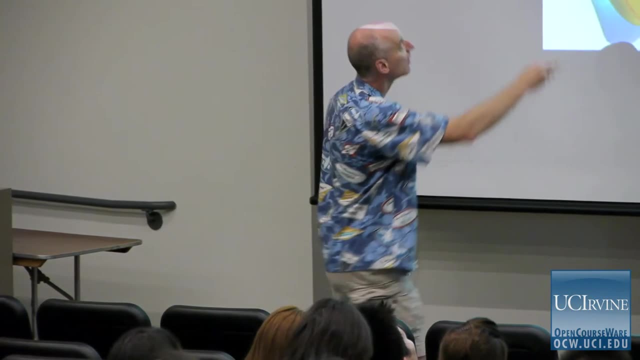 Those guys will get smaller. So you're having a greatelo, And so what that means is that the equilibrium constant that applies if we think about these activity effects is going to get bigger. If these guys get smaller, that gets bigger. That's the activity coefficient that applies. 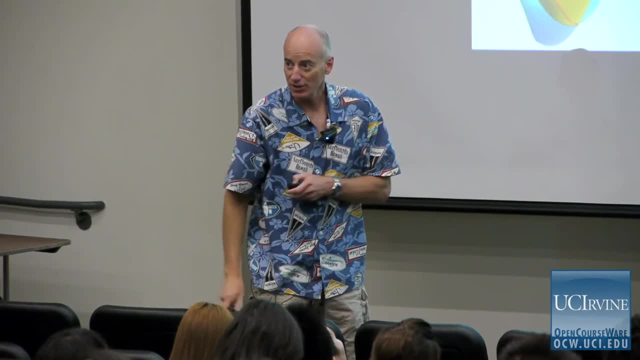 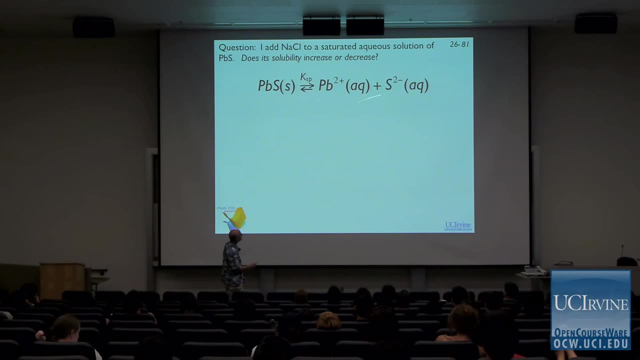 when we add sodium chloride to the solution or any other inert salt, It's going to get more acidic. What about this guy? What happens to the solubility of lead sulfide if I add sodium chloride to the solution? Sodium chloride doesn't appear in this equilibrium. 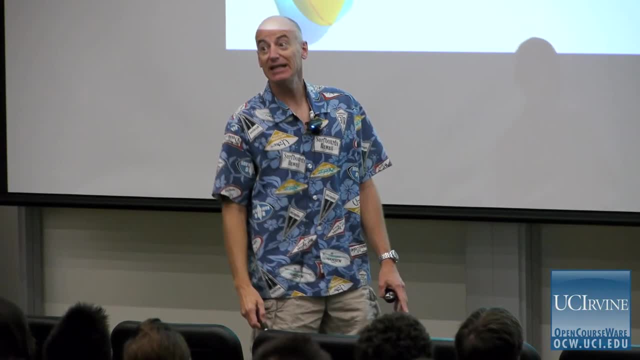 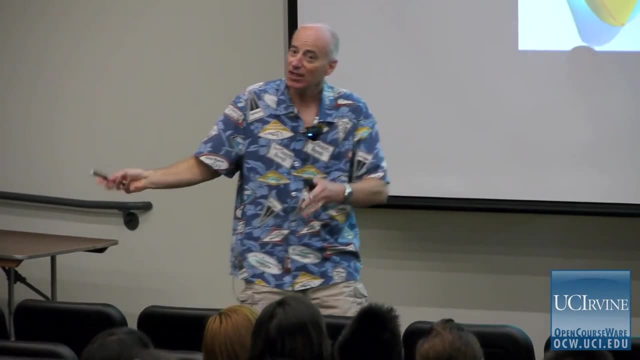 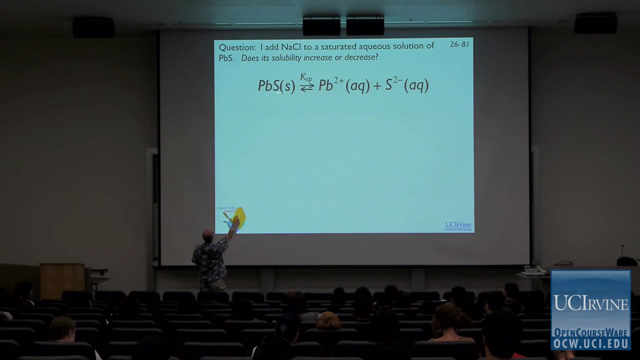 Why would it affect this equilibrium? And yet it does, in a predictable way. What's going to happen? Is the lead sulfide more soluble or less soluble when I dump sodium chloride in More? Why? Because, look, this side of the equilibrium has got a lot. 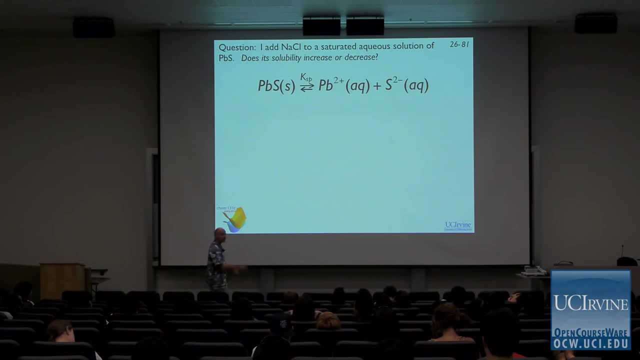 of ions. this side's got no ions. If I add more, it's going to be less soluble. If I add more ions to the solution, equilibrium is favored by the addition of more ions, And I can prove that's true by working. 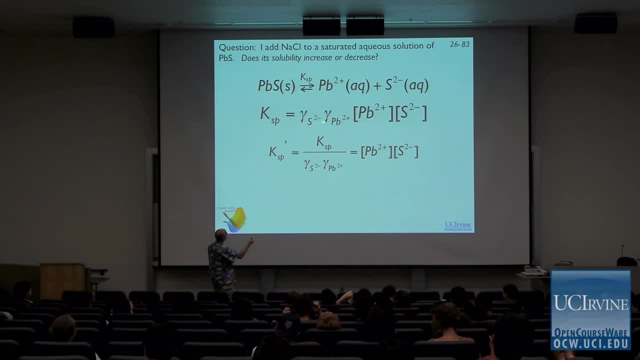 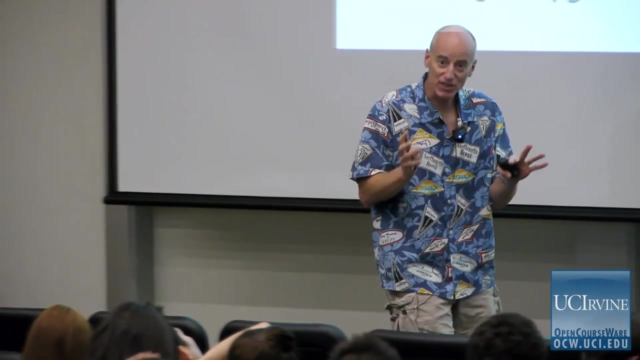 out what the new equilibrium constant is. These are the two activity coefficients. They both get smaller when I add sodium chloride, so the equilibrium constant shifts to the right. All right, every time you see an equilibrium, you can affect its position by adding an inert salt. 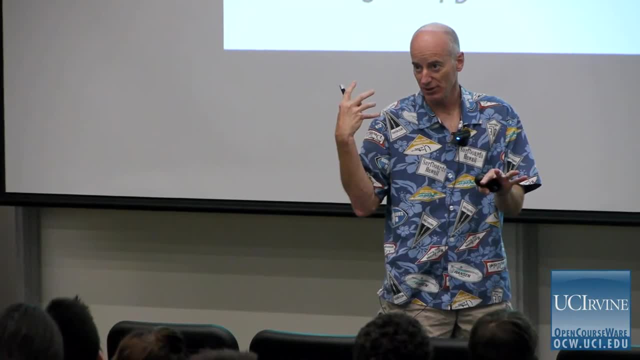 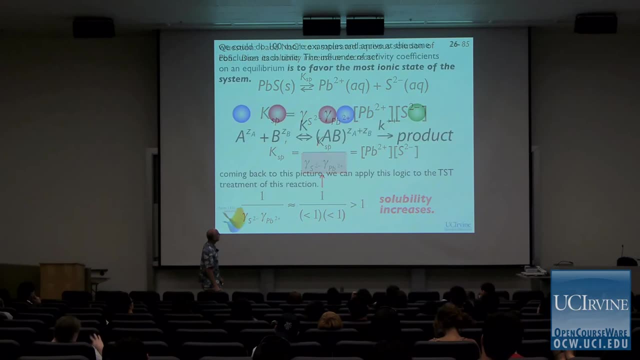 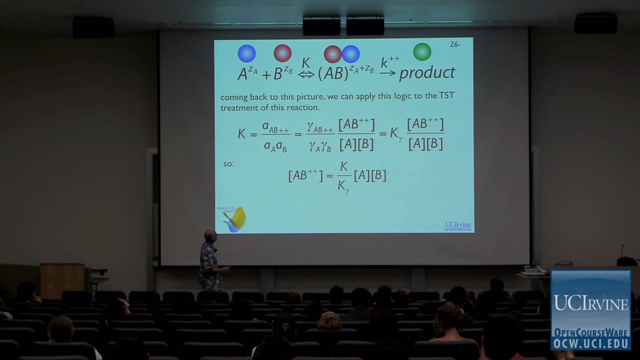 Adding an inert salt or removing an inert salt from the solution, that will also alter the equilibrium in a predictable way. Okay, what does all this have to do with transition state theory? Very simple, To make a long story short, we can work out the math. 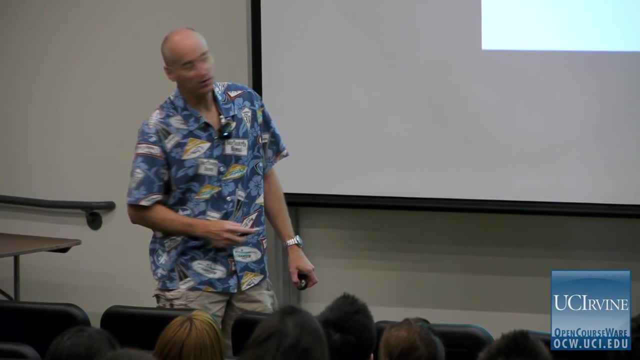 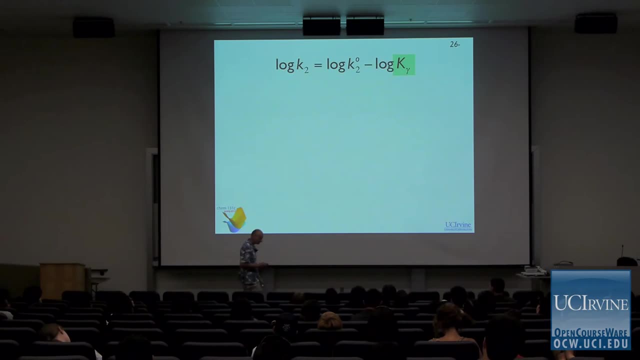 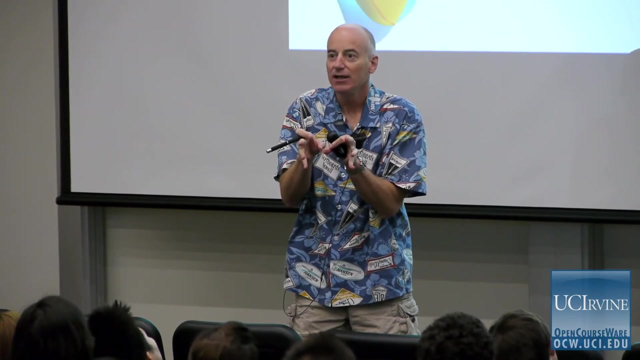 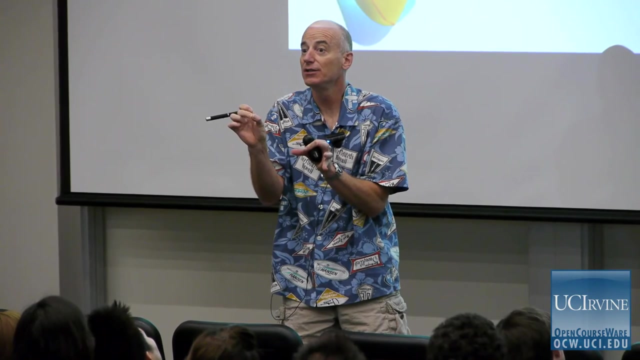 but we're just going to skip over it here because we're almost out of time. Here's the bottom line. The transition state has the total charge of the reactants in it. All right. If the transition state has a high charge, then the rate of the reaction is going to be influenced. 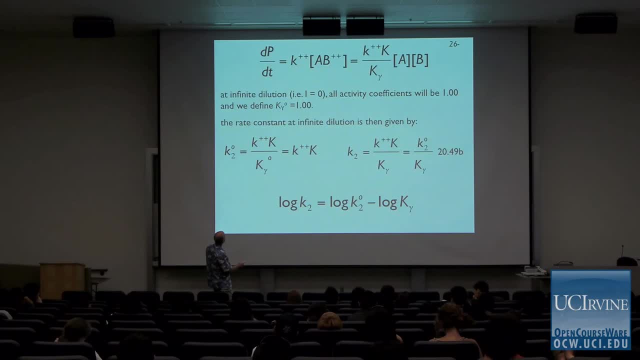 by the presence of other ions in the solution. So 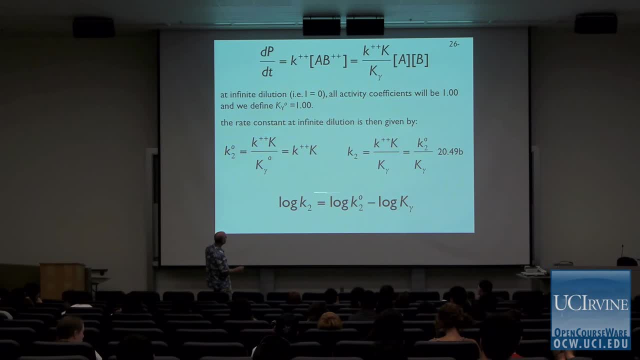 At the end of the day, when we're done, during the derivation, we get this equation right here, which is the equation for the kinetic salt effect. 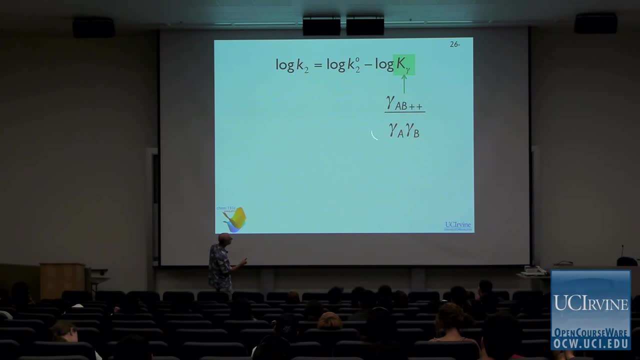 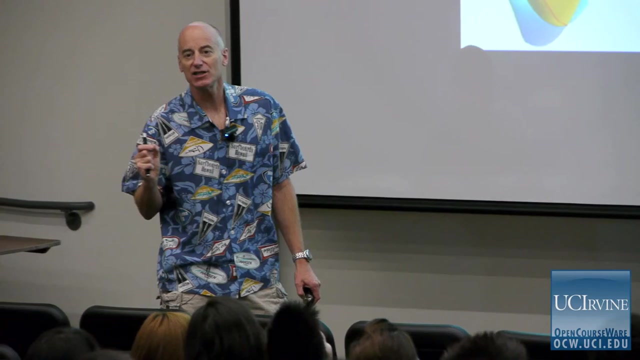 What is this big K right here? It's just the collection of the activity coefficients for the transition state and the reactants. Okay, That is the rate constant. that applies for one molar everything. That's why it's got a zero on it. 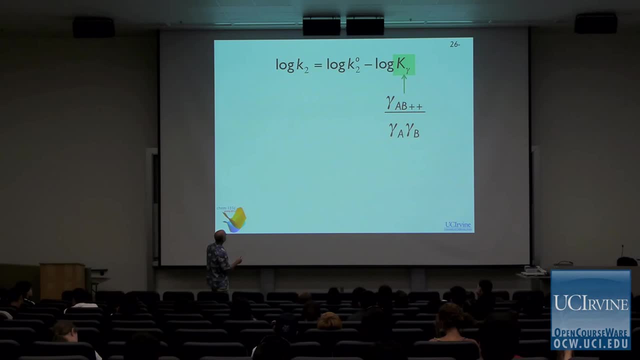 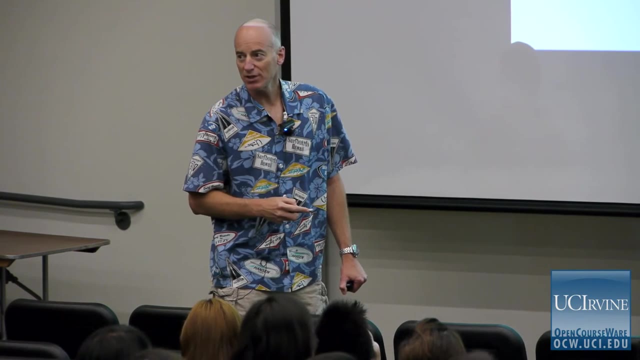 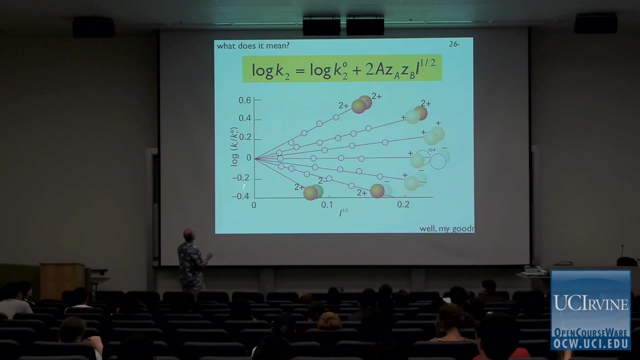 and that's the actual rate constant of the reaction. Okay, so this is the most important slide that has to do with this second concept here. All right, what am I plotting here? This is the reaction rate for a reaction that involves A. 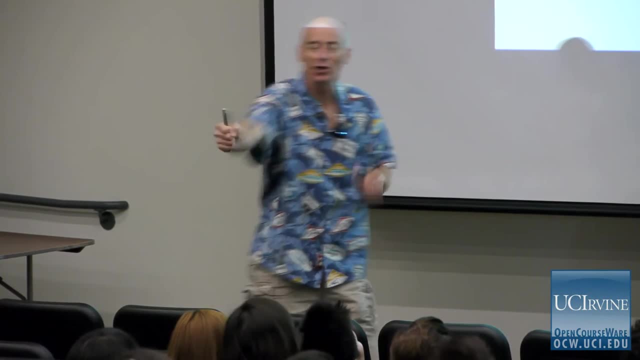 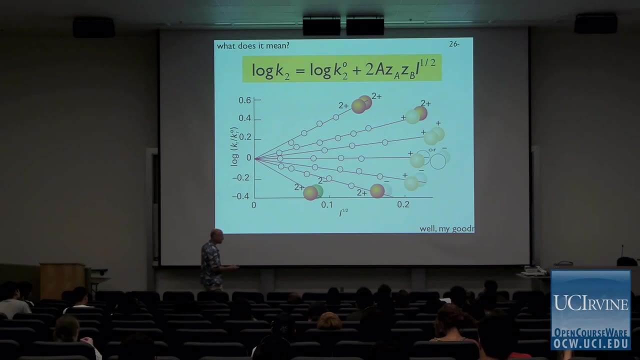 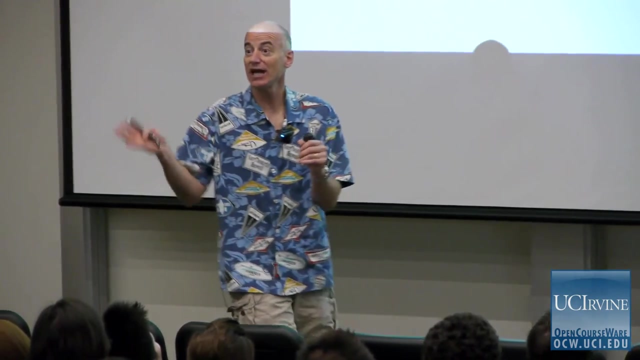 with some charge plus B, with some charge going on to products, all right, and this is the ionic strength, All right. so the key point here is: we want to understand how salt affects the reaction rate. It's easy to understand how salt affects the reaction. the equilibrium constant. How does it affect the reaction rate? The way to think about that is: if A reacts with B and they both have a plus 2 charge, they're both positively charged. they've both got a plus 2 charge. the transition state has a charge of plus 4, all right. 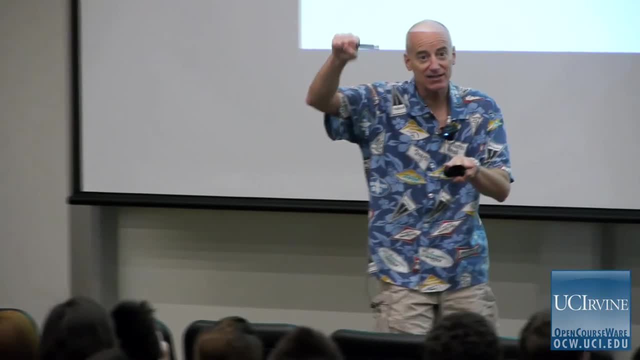 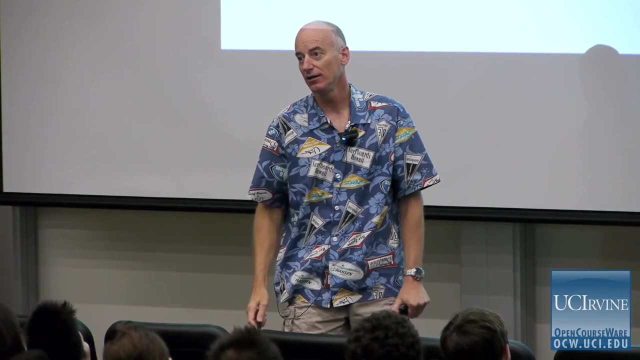 so if there's a charge of plus 4, there's an equilibrium between the transition state and the reactants. it's going to be favored by the addition of salt. The reaction's going to get accelerated, Isn't that counterintuitive? The reaction rate goes up as I add salt to the solution. Even though the reactants and products have the same charge, they have to overcome a coulombic barrier to react because they're both positively charged. the reaction rate goes up, Not down. 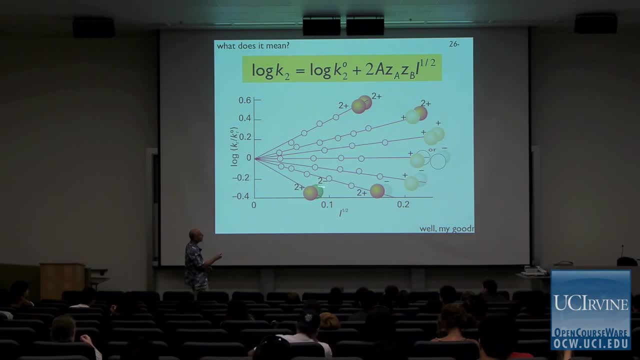 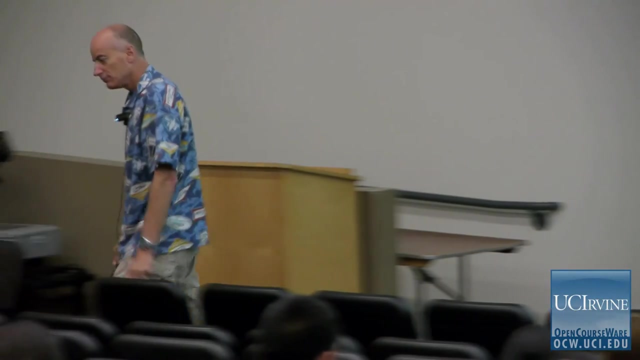 Check this out. If a 2 plus ion reacts with a 2 minus ion, you'd expect there to be a big coulombic attraction. right, Reactions should go faster. It goes slower. Does this have to do with the orthogonal components? 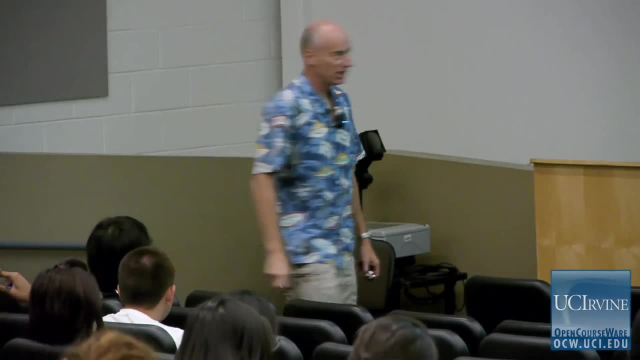 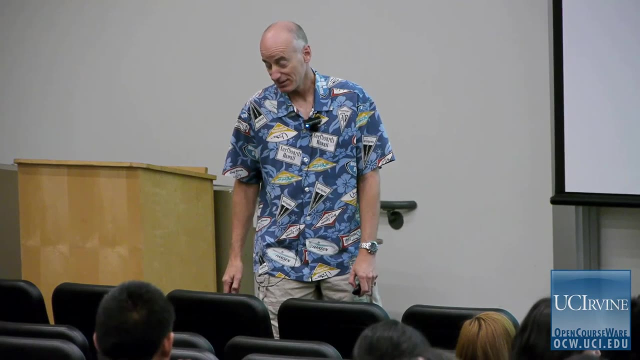 of the transition state's partition function? Absolutely not. No, No, Nothing at all. No, It has nothing to do with the energy of the voltage Zero. I'm just thinking about it. Okay, It's not a bad question, but the answer's no. 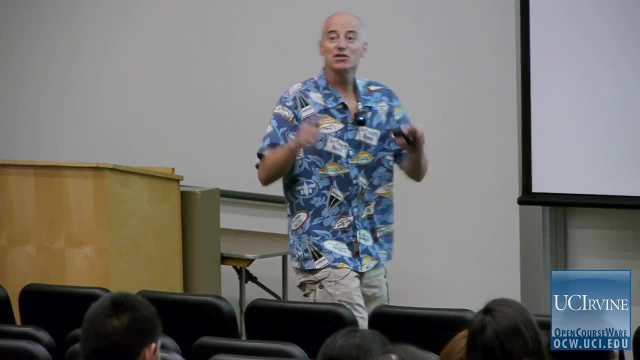 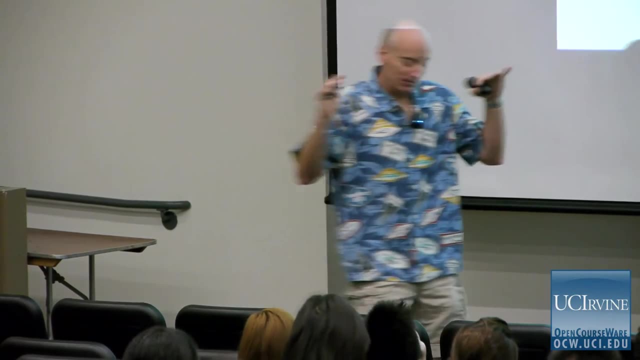 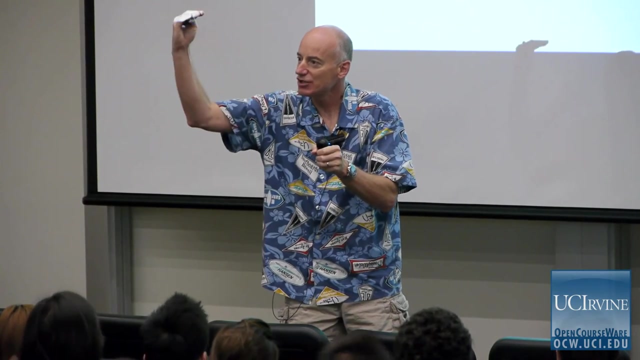 Does everybody see why this happens? There's an equilibrium, I'll say it. I'll say it. I'll say this one last time because I don't have any more time. There's an equilibrium between A and B- all right. the reactants and the transition state: all right. What we just agreed on is that we can decide which side of the equilibrium will be favored. when we add salt to an equilibrium, the most ionic state of the system is favored. okay, So if the charge on the transition state is higher than the charge on either one of the ions, because the only way 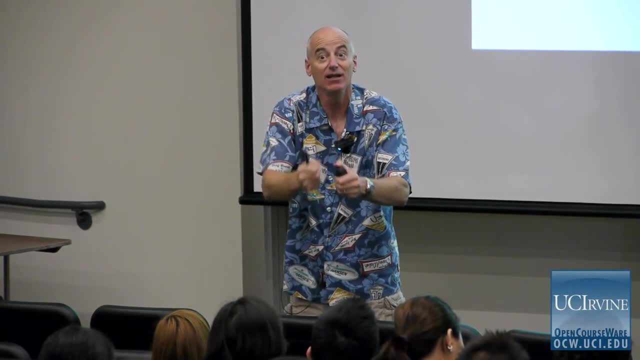 that can be true is if the ions have the charge of the same sign, like plus 1 and plus 2,, plus 2 and plus 2,, plus 1 and plus 1, right then the charge on the transition state will be. 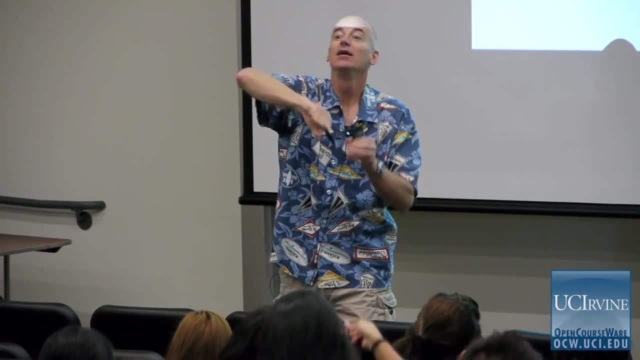 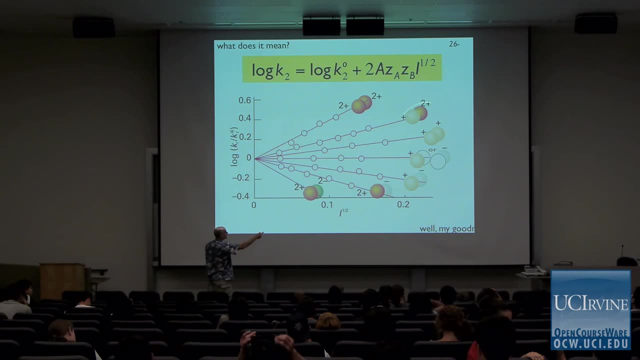 like 3,, 4, and so on. The transition state will be like 3,, 4, and so on. The transition state gets favored by the addition of salt, okay, and the reaction rate goes up. Look, it goes up here too. 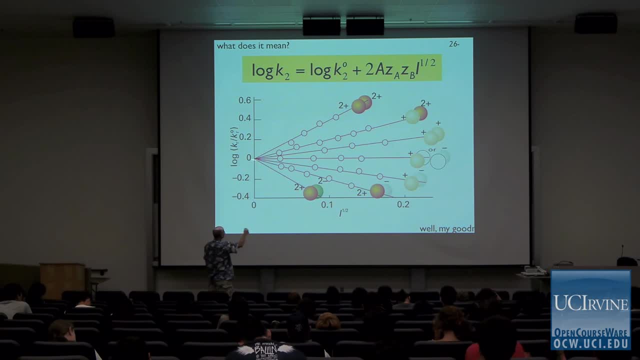 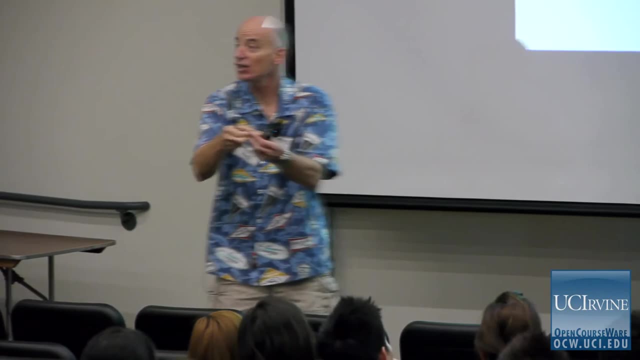 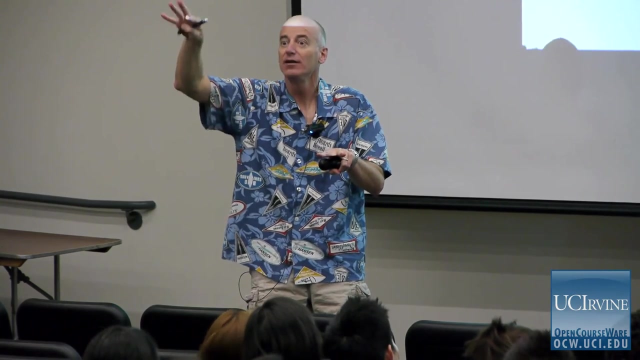 Look, it goes up here also. all right, If there's no charge, nothing happens, and if the charges on the reactants are opposite to one another, then the charge on the transition state is lower than the charge on the ions. The transition state has a lower ionic. it's the least ionic state. 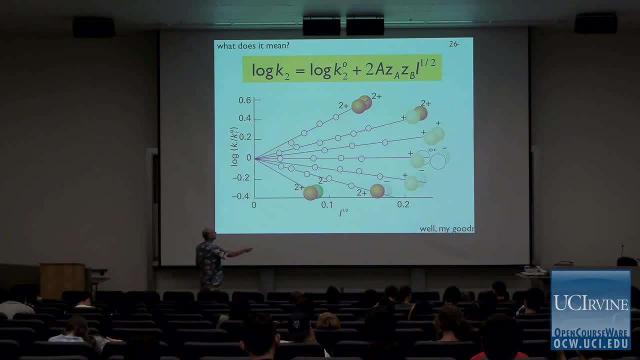 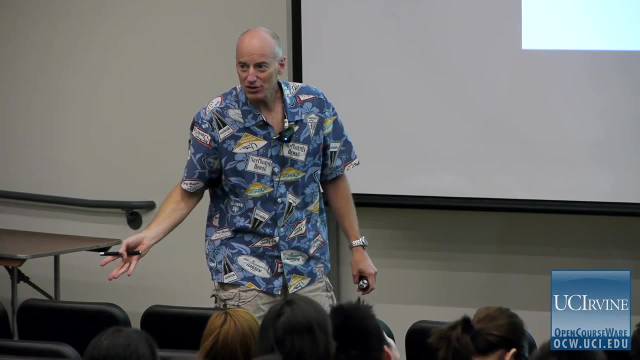 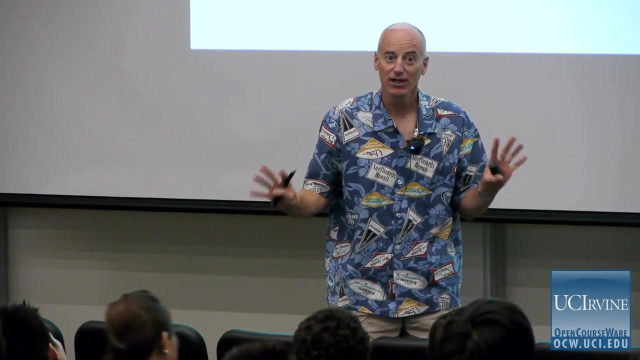 of the system. The reactants are more ionic than the transition state and the reaction is slowed down by the addition of salt. That's totally counterintuitive. If you understand that, you understand something that most chemists even are going to get wrong, all right. 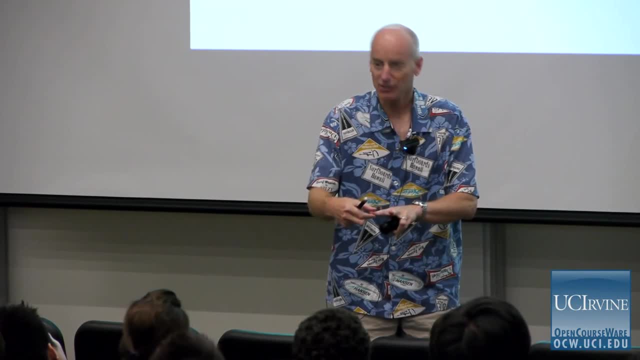 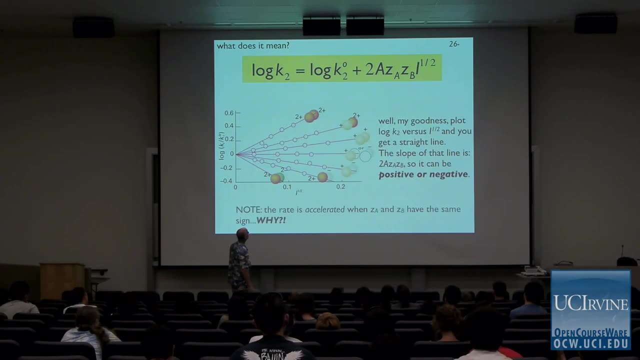 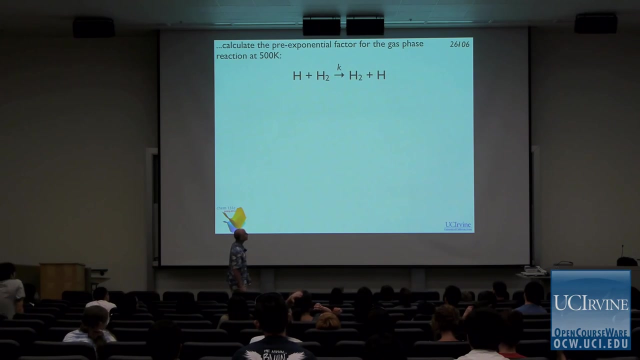 You're going to get it right, all right, You say those charges. that reaction is going to go slower. You can think about. okay, so on Friday, yeah, there's more here. Yes, oh my goodness, All right, and there's like 20 more slides that work.